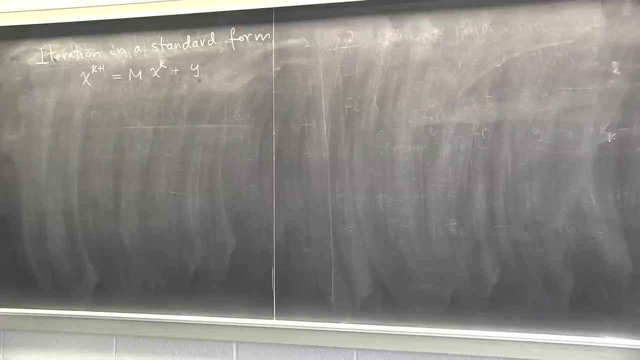 And we did it for Jacobi, and we did it for Gauss-Seidel, but we didn't have time for the SOR which we will start today. so we'll be convinced now, after we derive this, that all of them is with this form. 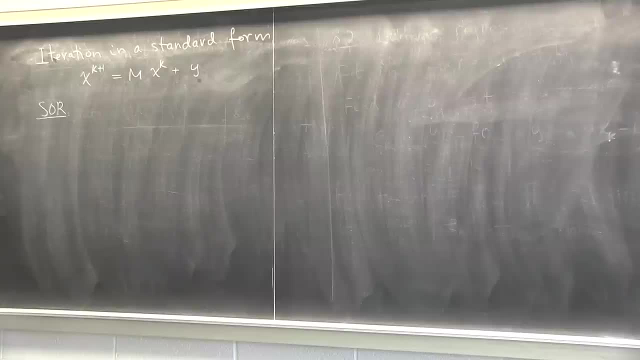 Okay. so in order to write SOR, if you recall the method SOR, it just makes a linear combination of xk plus the result from Gauss-Seidel. is that right? Okay, so I'm going to revisit the Gauss-Seidel. 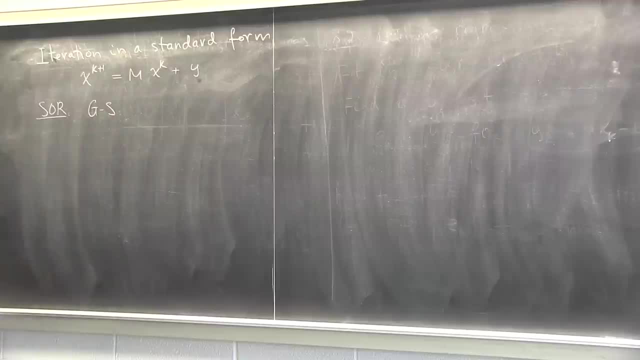 Okay so I'm going to revisit the Gauss-Seidel and write it in a more friendly way for this computation. Okay so, Gauss-Seidel. what we did with Gauss-Seidel was we kept the diagonal on the left-hand side right. 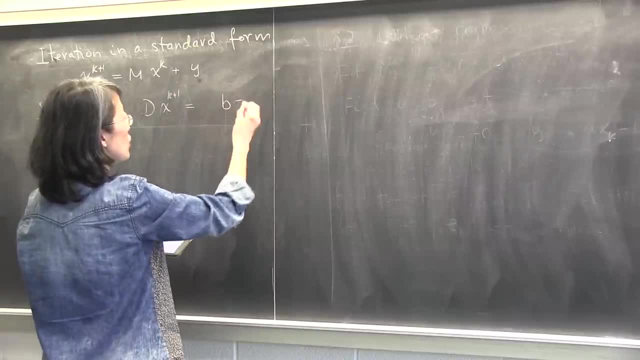 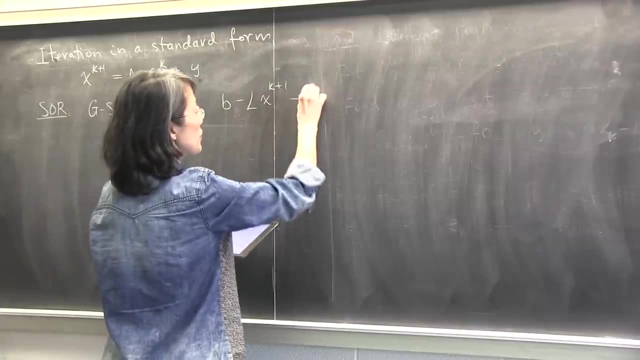 If you just write it as the Jacobi iteration, but then the L is multiplied by xk plus 1, because you have those information already, and then u is multiplied by xk. You can write it like this. You can write it like that also. 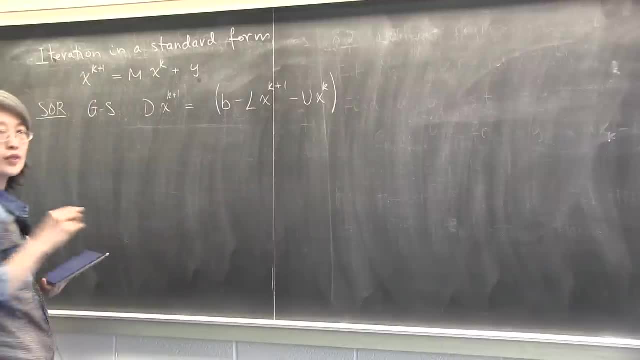 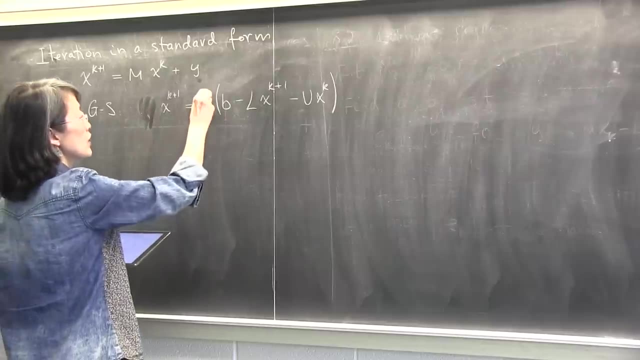 That's how you actually do your computation. you actually don't compute the inverse, you just do this multiplication right. So I can multiply both sides by the inverse and write it as xk plus 1, equal to that, And that's actually how you compute, okay. 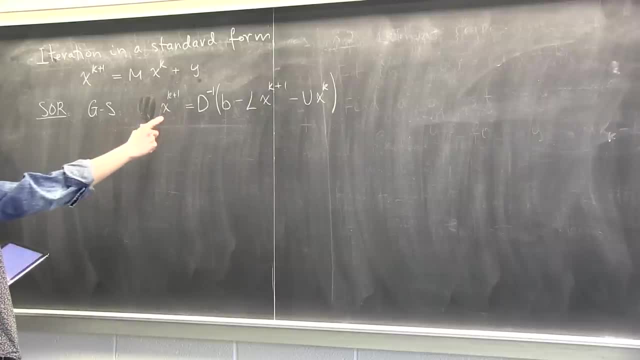 Not how you did the analysis, And it's this one that you multiply with an omega combined with xk into the SOR. Remember That's how you did the SOR, right? Okay, Now SOR. the iteration can be written as follows: xk plus 1 as a vector will be 1 minus. 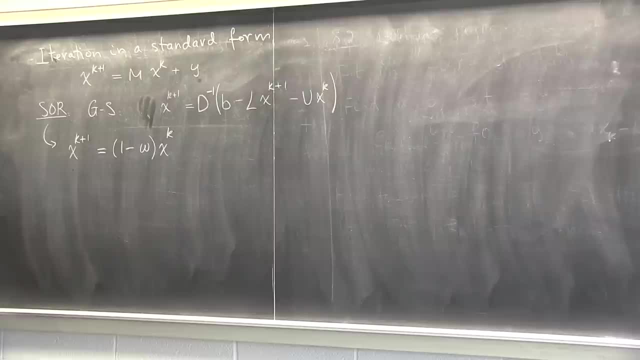 omega xk. So you prefer me to call this omega or w. It looks the same: Omega, Omega. Okay, It gets myself confused. sometimes I start to call it w but stick to omega And then omega multiplied by Gauss-Seidel. 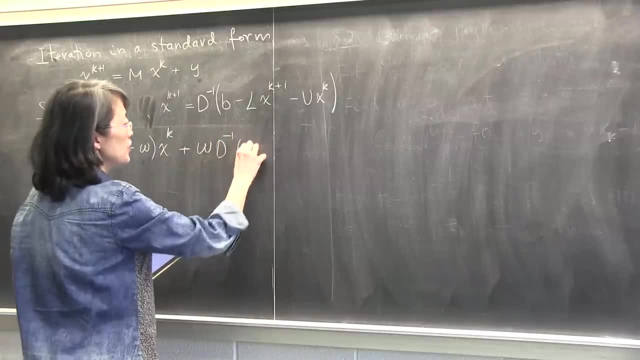 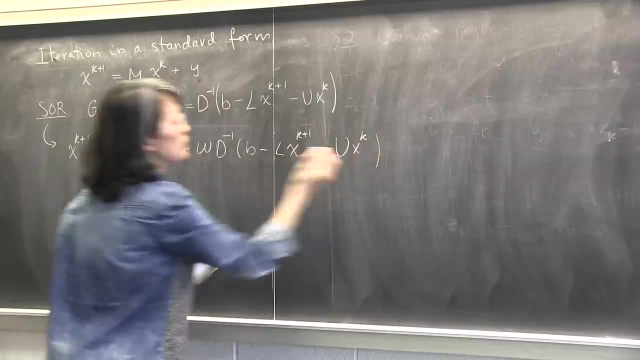 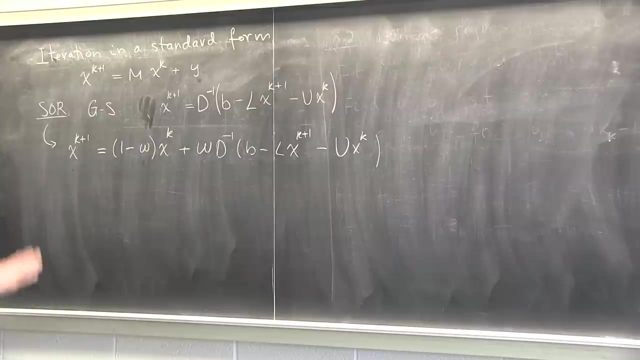 So this guy here. so d inverse b minus l xk plus 1 minus u x. So this will be actually what the algorithm will be doing, right? So what we want to do now will be manipulate this, in particular, move the xk plus 1, all. 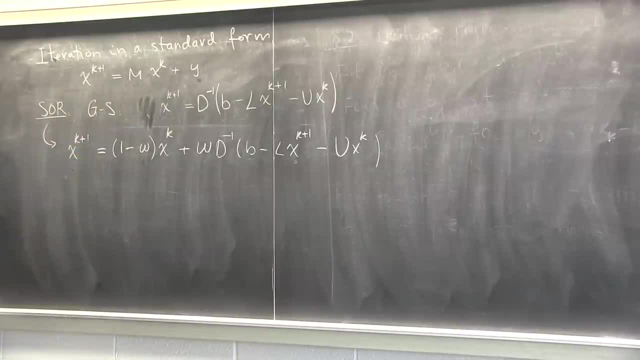 to the left and try to rewrite it into this form for some m and y. Okay. So we'll start with Okay, Multiplying both sides by d on the left, to get rid of this d inverse here. Is that okay? 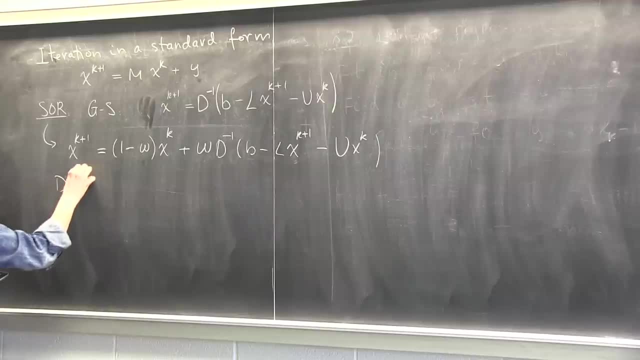 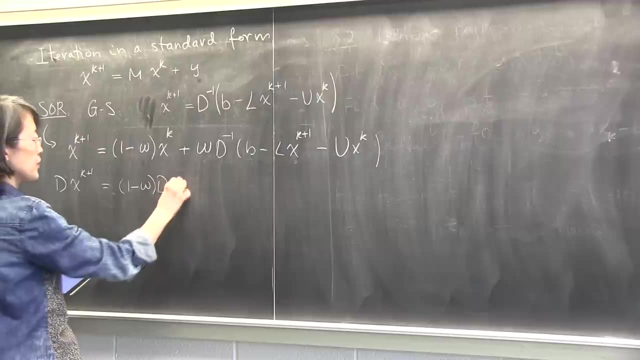 So I do that, So I can multiply by d. xk plus 1 equals 2, and that's just a number. I can put it in front. Okay, And then if I multiply by d, it cancels the d inverse. 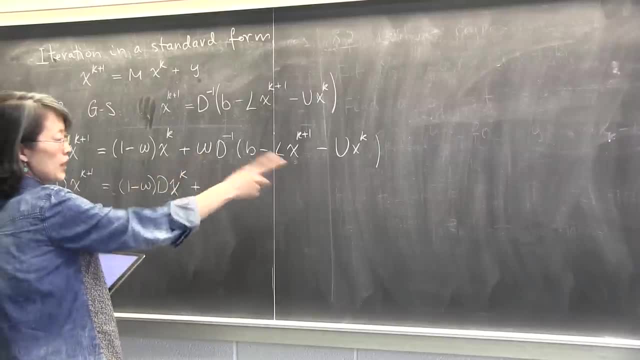 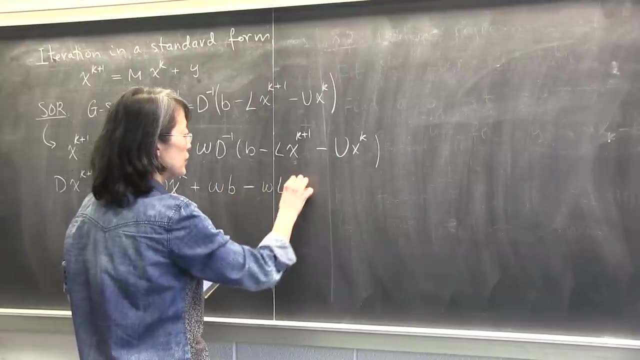 Right, And it's gone, And then I will have omega times, that- And I'm going to distribute omega into each term. Okay So, omega b minus omega l- xk, plus 1 minus omega u- xk. Okay, We, okay. 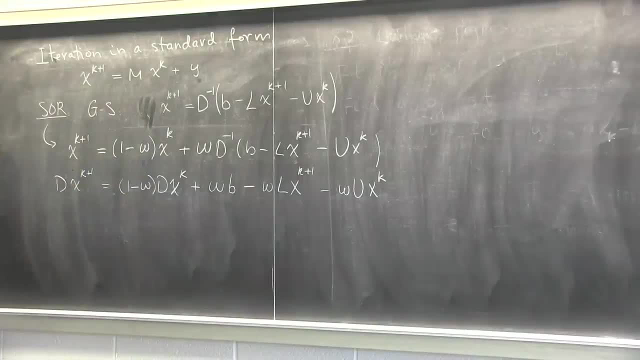 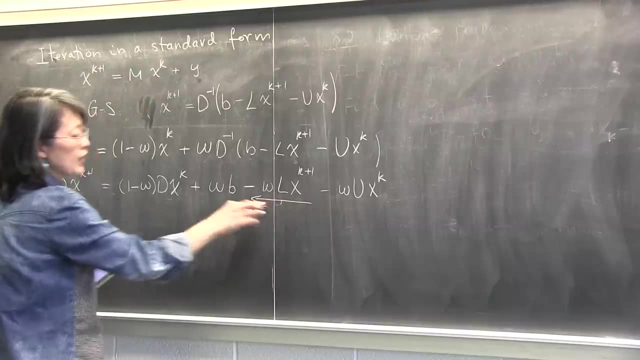 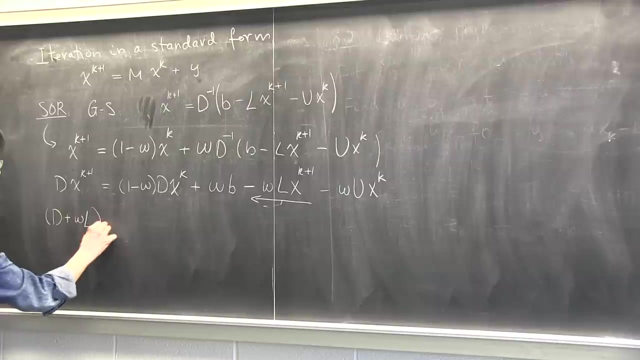 Didn't do much, Okay. And then you know, your goal is to move this to the left. So this guy will go to the left-hand side of the equation, And then I'm going to join the d with omega l times xk plus 1.. 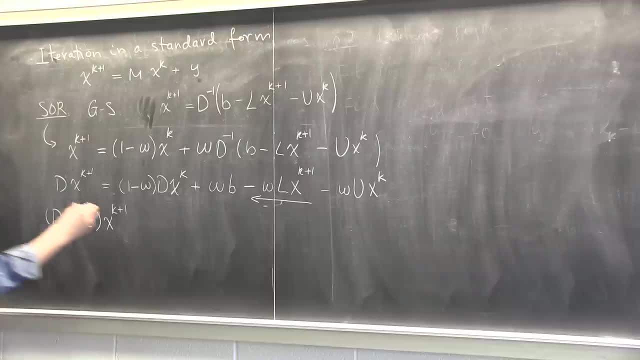 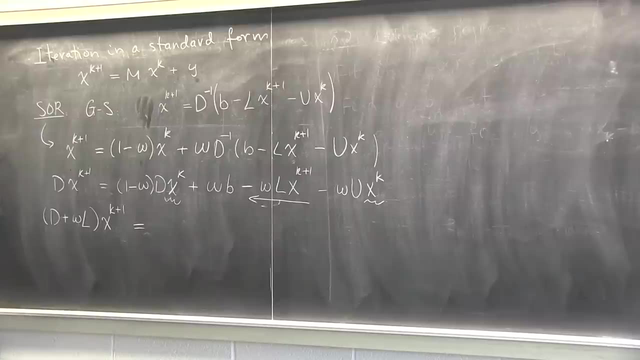 So this guy goes to the left And then I have three turns on the right And I will join the turn that contains xk. Is that okay? I put these two together, these two with xk, So I can add the matrices in front of them. just add them up. 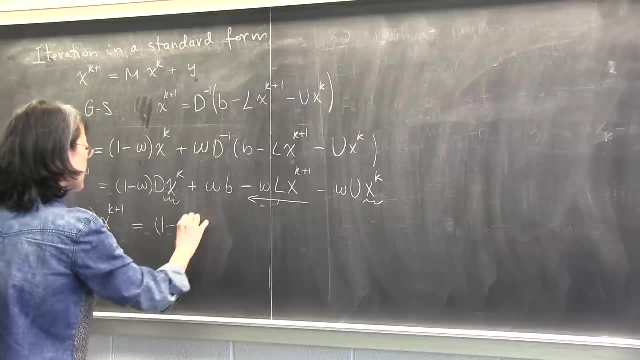 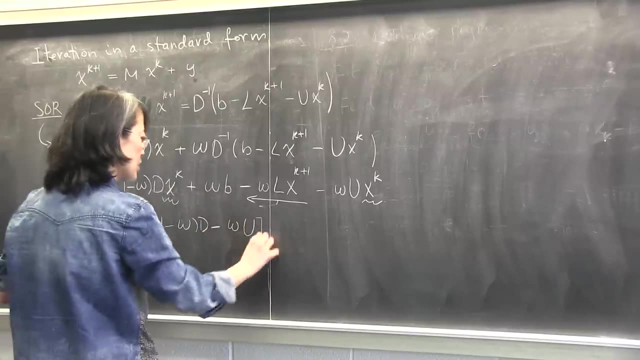 So I will get 1 minus omega of d minus omega u if I combine them, So that will be a matrix. you know, a number times a matrix. A number times a matrix is a matrix. A number times a matrix is a matrix. 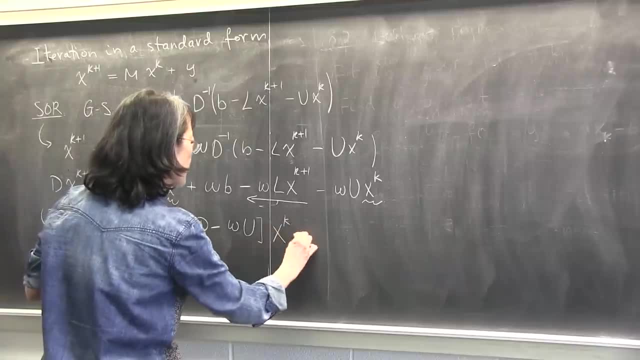 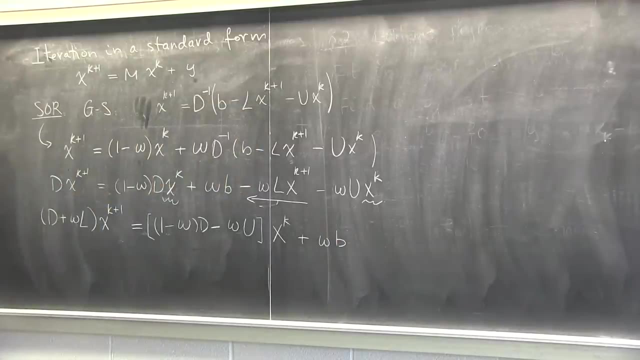 Subtract, you get a matrix That's in front of xk plus omega b A vector. Are we okay? Okay, We're almost there. So next I will multiply both sides by the inverse of this guy. Okay, And then the left-hand side will have xk plus 1 standing alone. 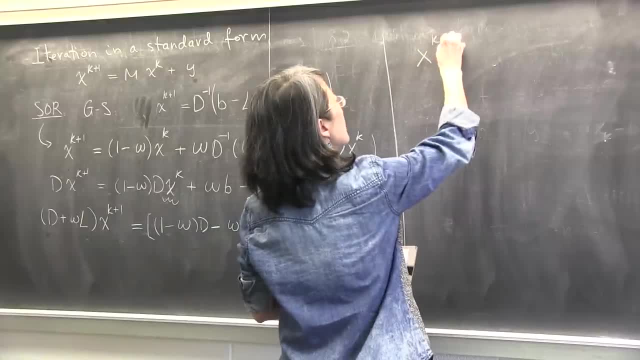 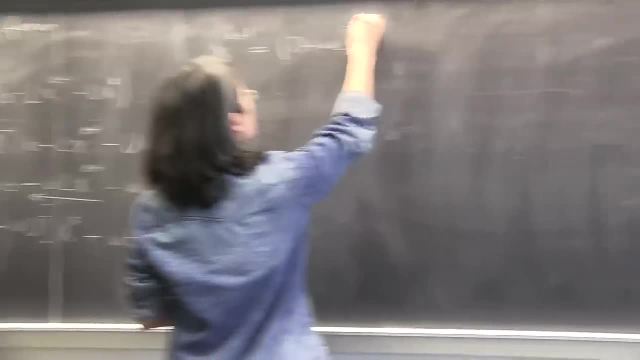 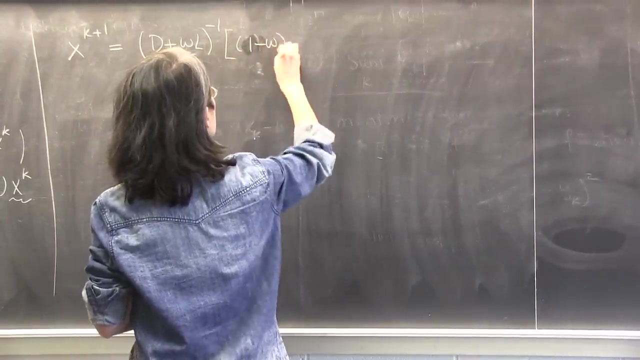 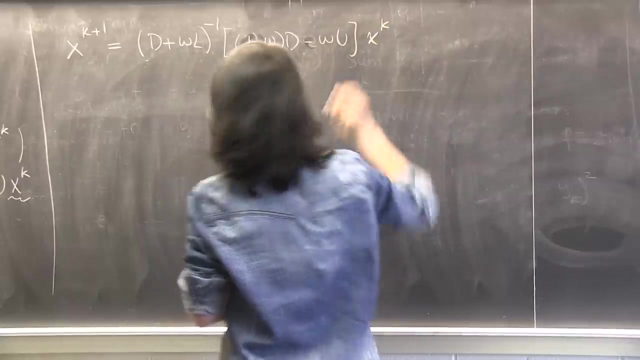 Right. So this gives me the following: xk plus 1 equals to- it just looks a bit big: d, omega, l, inverse times this big matrix. Let me write it: 1 minus omega, d plus omega. no minus omega. u times xk. 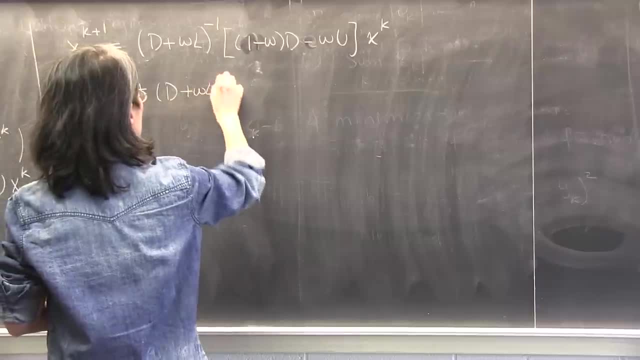 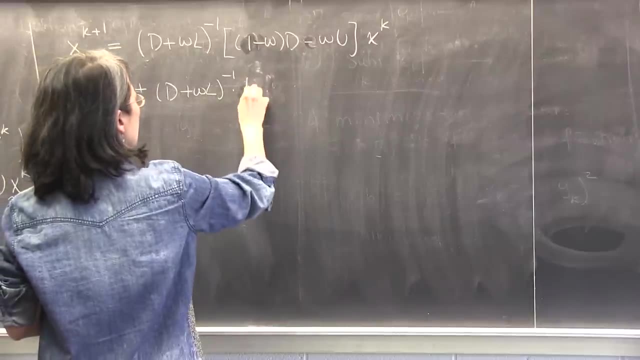 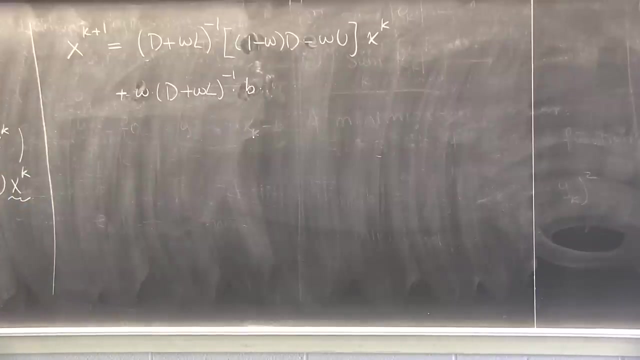 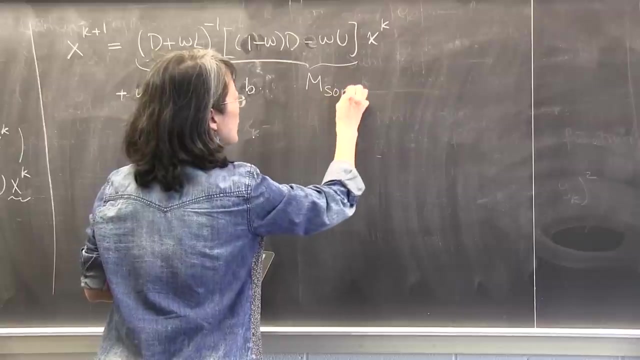 And then I have this inverse Apply on the vector. Omega is a number. It might be better if I move it to the front. It's a scalar number. Now, you see, I can call this whole thing here, which is a matrix. I call it this matrix M with SOR to indicate that's the iteration matrix for SOR. 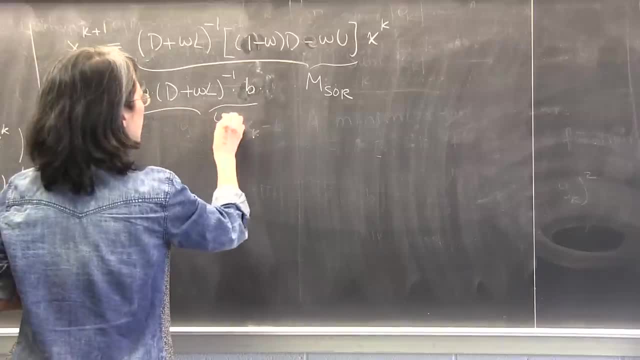 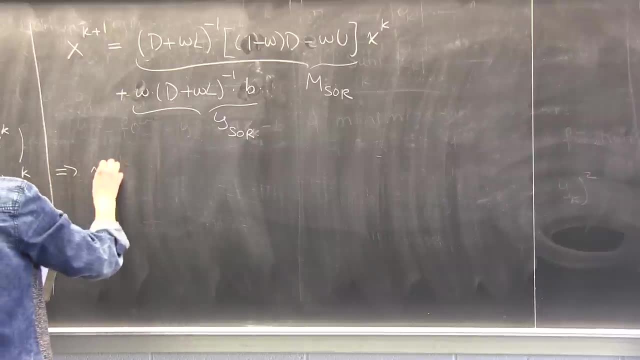 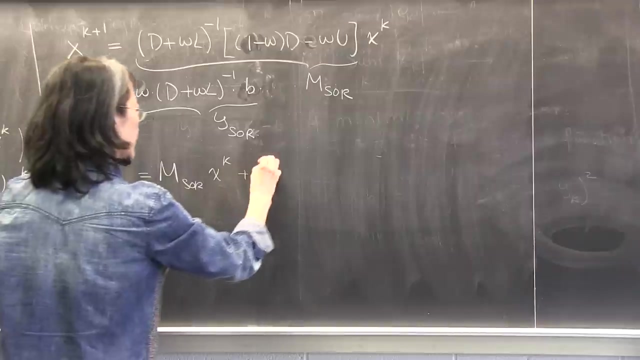 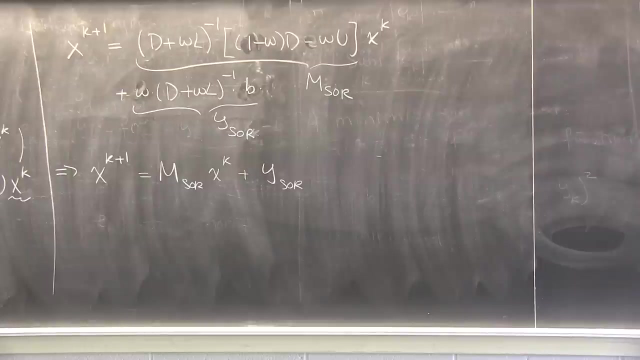 Right, And I call this guy the vector y, SOR. Is that okay, So, which means we've managed to write it as the following form, So in that standard form, as we claimed it would do. Is that clear? So, all three methods: Jacobi, Gauss-Seidel and SOR. 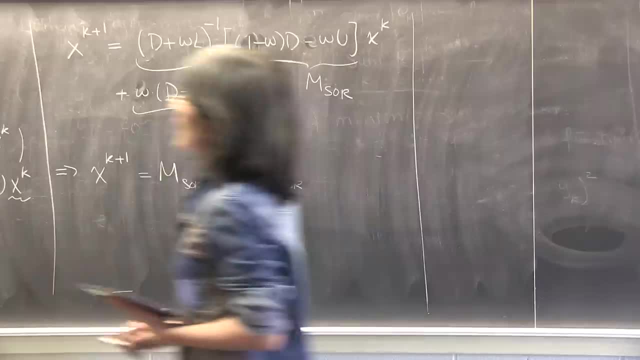 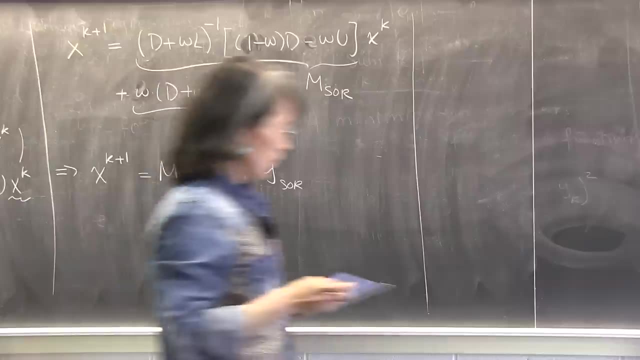 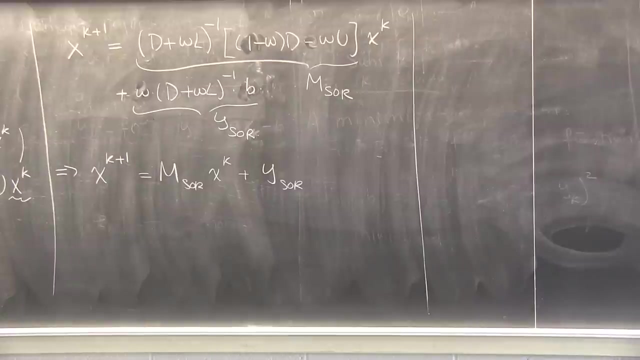 we managed to write them all three of them in the same form, which is this form, So that makes the job of error analysis easier. That is, we just need to do error analysis to that standard form Right. As I said, one shot kills three birds. 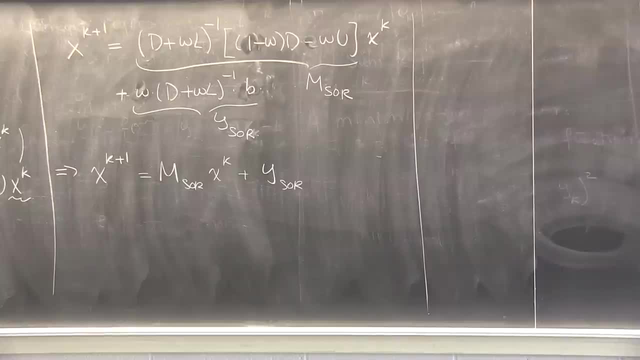 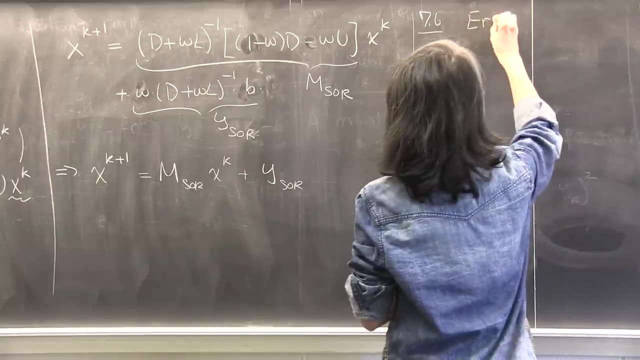 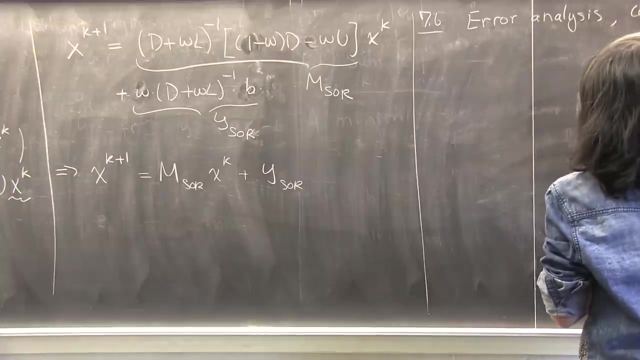 Poor birds Didn't want to kill them. Okay, Let's do the analysis. So we just need to consider the standard form. So we will do the error analysis which in the end will lead to convergence result. Okay, So we consider the standard form. 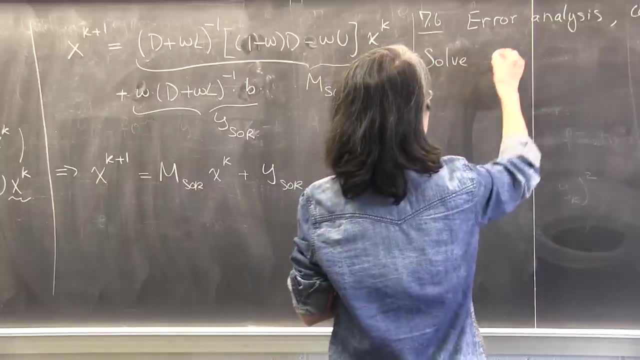 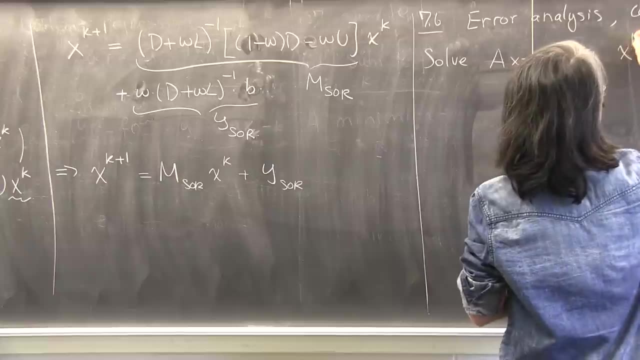 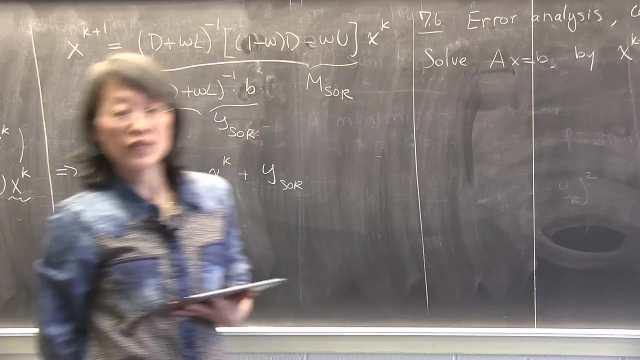 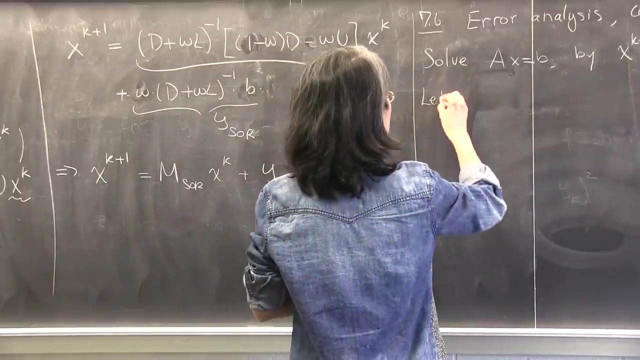 Let's say we want to solve this equation AX equals to B- by this iteration: XK plus 1 equals to MXK plus Y, One of our methods. So you know, this is a fixed point iteration for that problem. Okay, And then let now S be the solution. 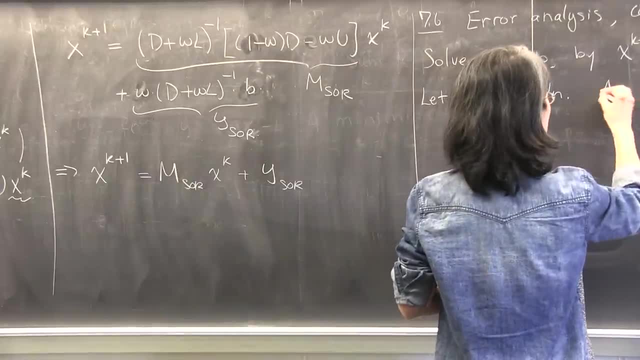 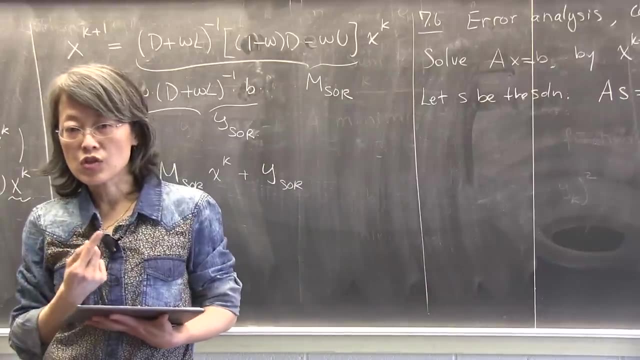 So if S is the solution, what do I know? Well, that means A times S equals to B. Okay, That means S is going to satisfy my equation. Is that right? And it's also the fixed point of my iteration. What does it mean? 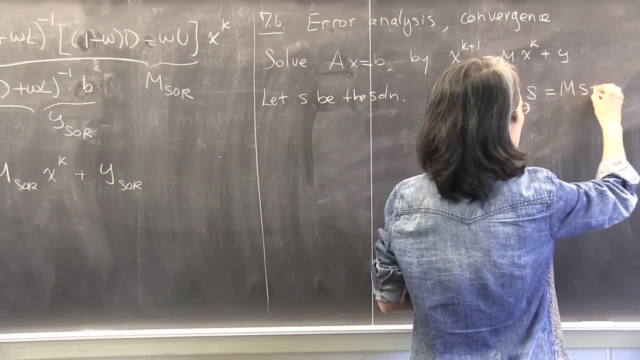 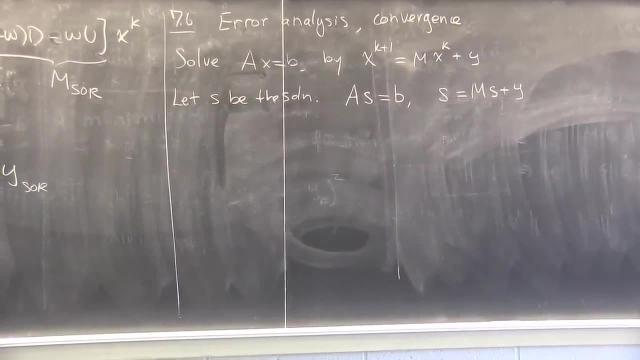 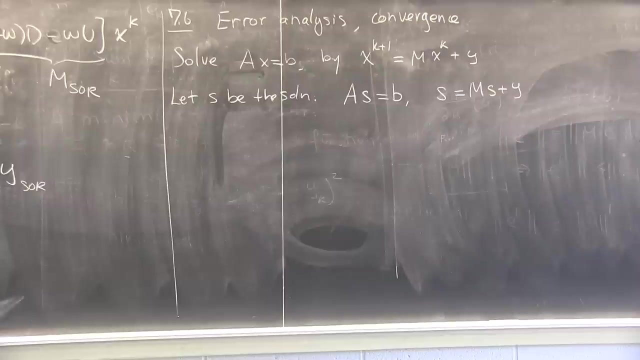 That means also: S shall equal to MS plus Y. It shall be the fixed point as well. Is that right? Okay, We have done this many times for fixed point iteration, but for the scalar function. This is just system. It's the same way. 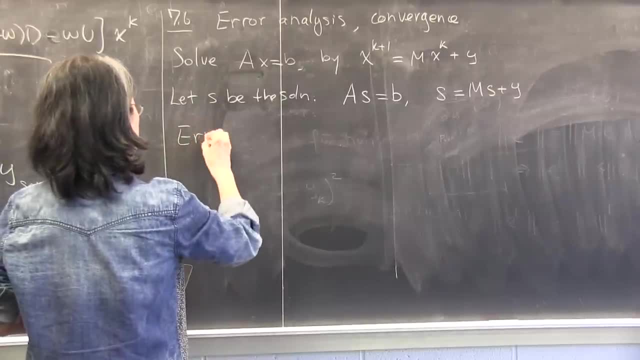 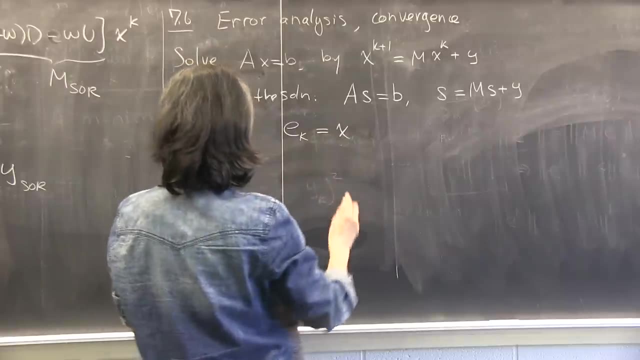 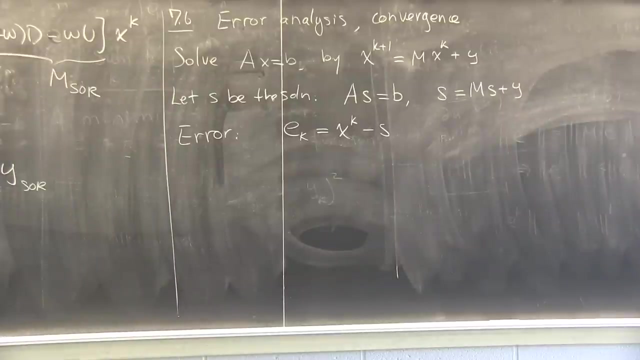 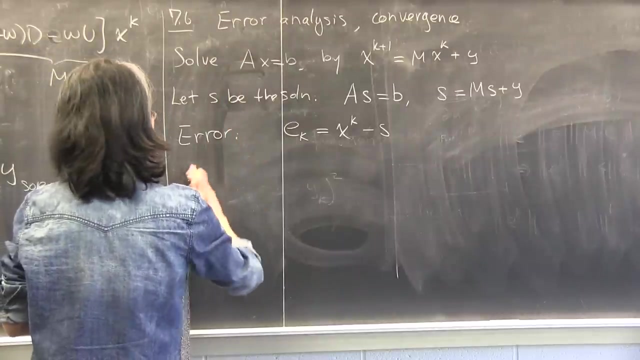 Okay, Let's define arrow. So EK right now is defined as the distance between XK and the exact solution. Okay, Right now the arrow is a vector. Okay, Let's leave that, and then we will take norm afterwards. Okay, And then we want to understand how the arrow evolves. 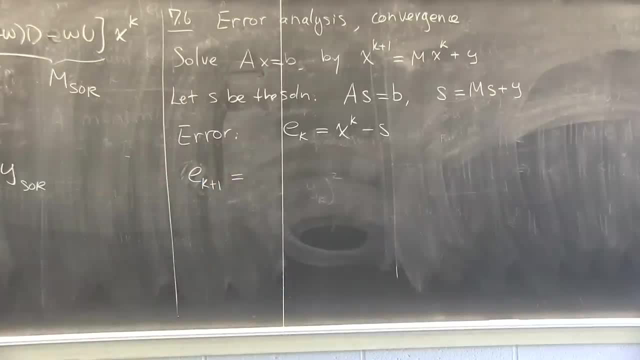 the evolution of your arrow after you take an iteration. So we want to understand how EK plus 1 relates to EK. Okay, So what is EK plus 1?? Well, by my definition, this is XK plus 1 minus S. 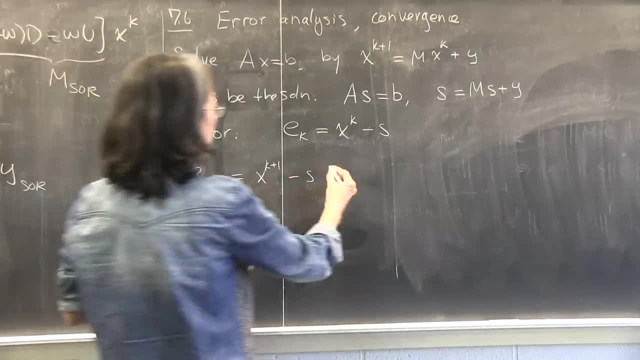 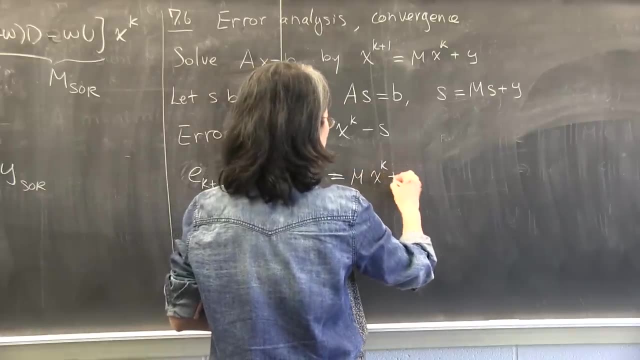 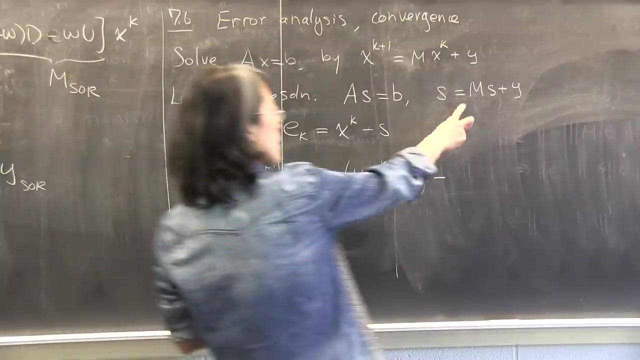 Is that right? So how did I compute XK plus 1?? Well, I did it by my iteration. So it's MXK plus Y, Is that right? And S is the fixed point, meaning S satisfies my equation, So I can substitute it with MS plus Y. 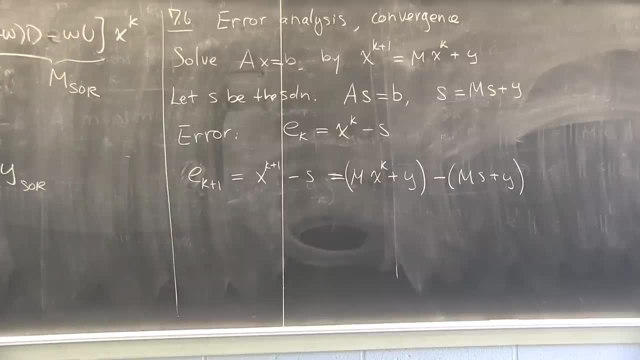 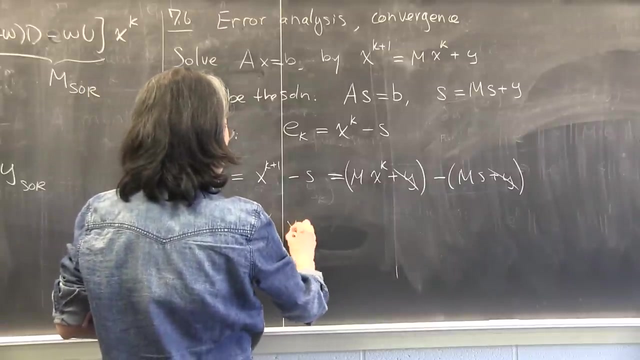 Is that right? We've done that many times for when we talk about fixed point iteration. So we see the Y cancels the Y. So all I have is the same matrix times X and the same matrix times S. I can take out the matrix and write it as XK minus S. 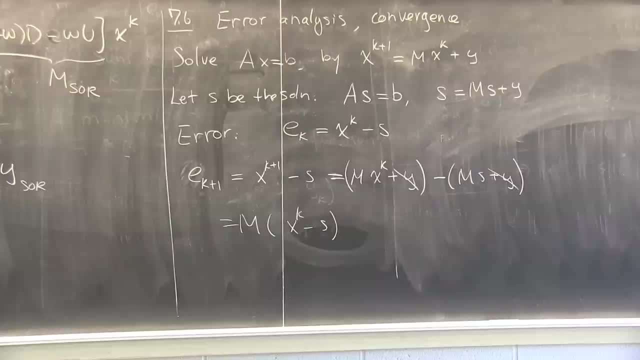 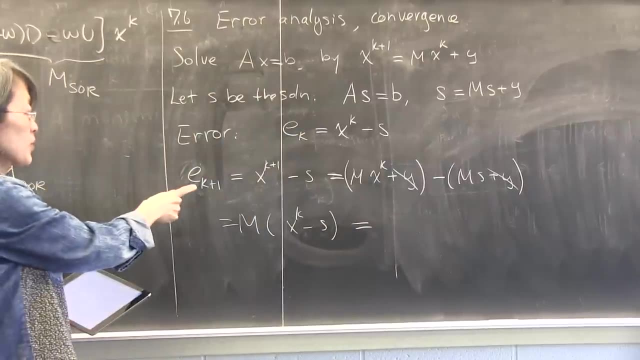 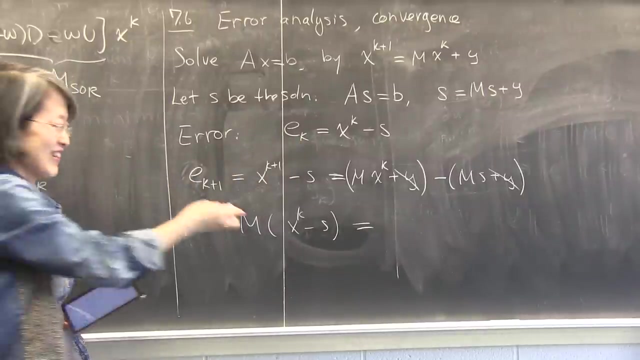 Okay. So what is XK plus 1? Y minus S. What was I trying to do? Build a relation between this one with that one. Does that one appear on my right-hand side now somewhere? Isn't this just the arrow at step K? 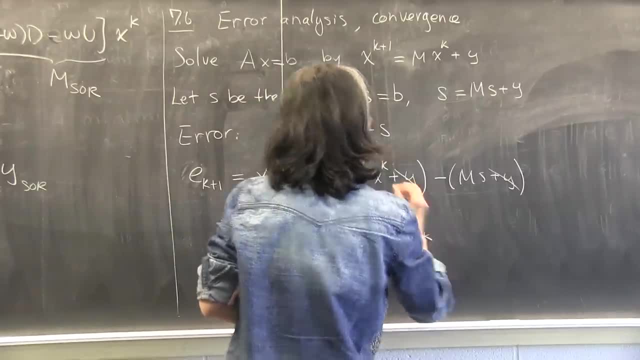 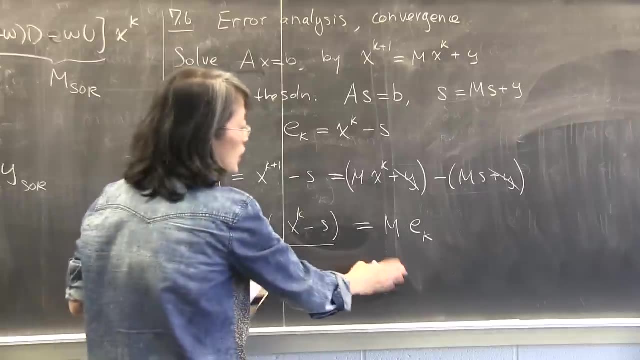 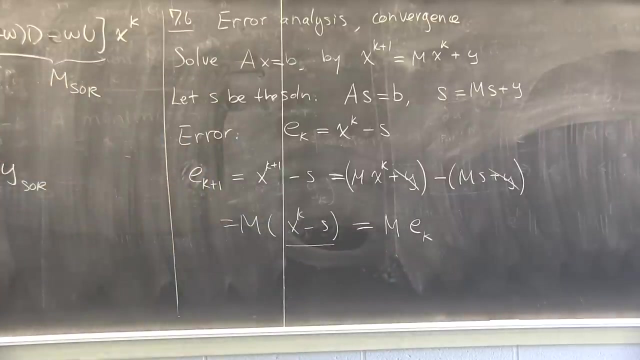 Is that right? So M times EK. Now you see how the arrow evolves in iteration. After each iteration, your arrow is multiplied by this matrix M, and that becomes the arrow in the next step. Is that clear? Only the M matters. 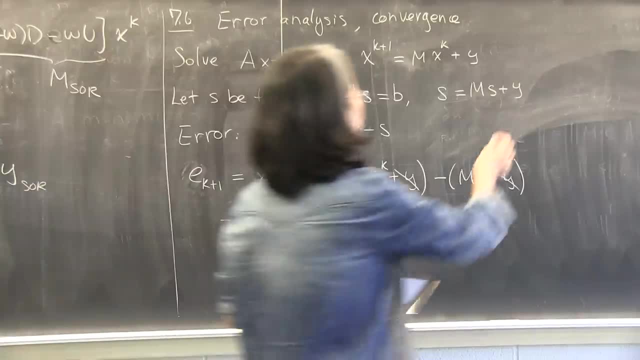 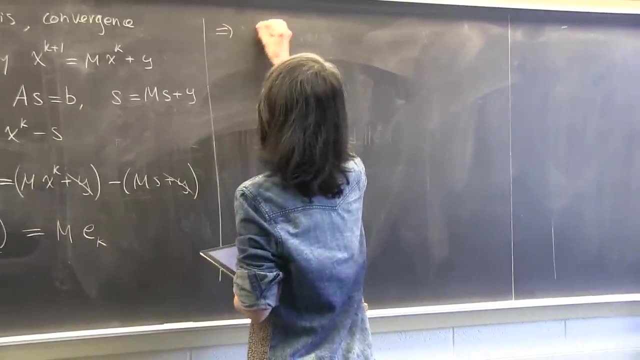 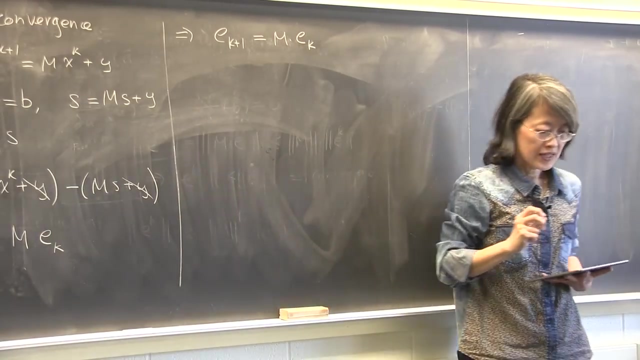 The vector Y doesn't matter. Okay, Okay. So what does it mean? Let me write it again. So we have the following arrow: evolution: EK plus 1 equals to MEK. So right now, M is a matrix and those Es are vectors. 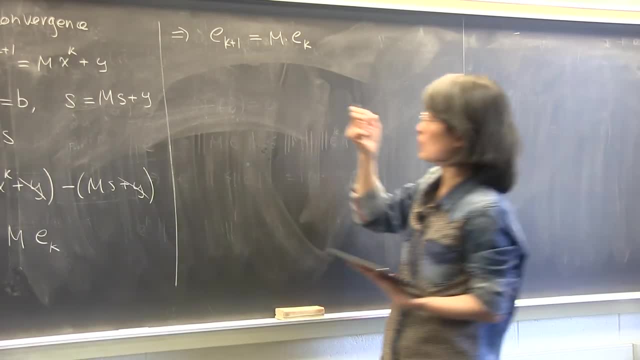 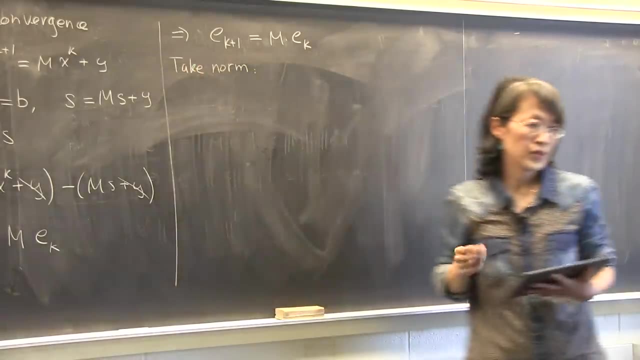 So I would like to measure them by some norms. So we'll take some norm, your favorite norm, vector norm, whichever vector norm, say L2.. Let's say, I take out L2 norm, So let's just denote it by a norm. 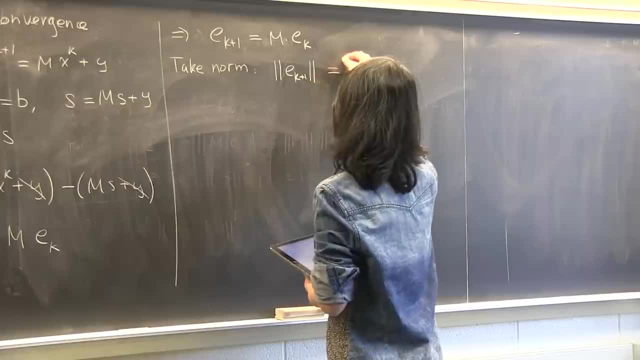 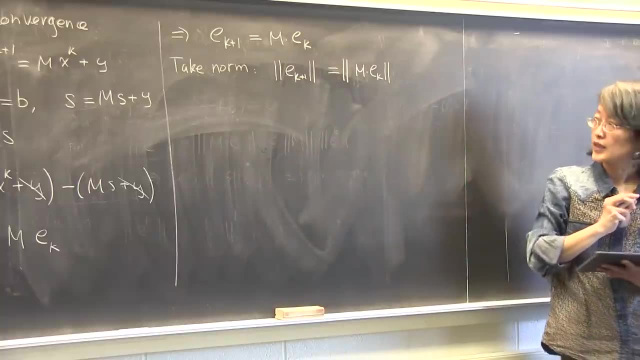 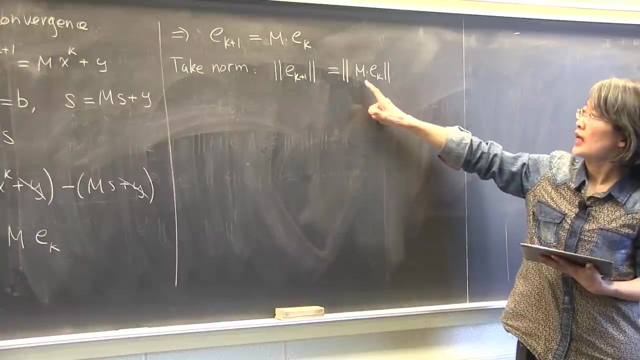 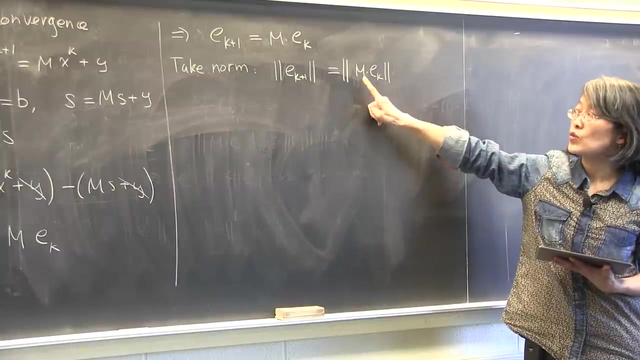 So EK plus 1 equals to the norm of MEK Some vector norm? Okay, Not specified which one. So then we'll use this relation, that is, a matrix times a vector taking norm. You can express this in terms of the matrix norm times the vector norm. 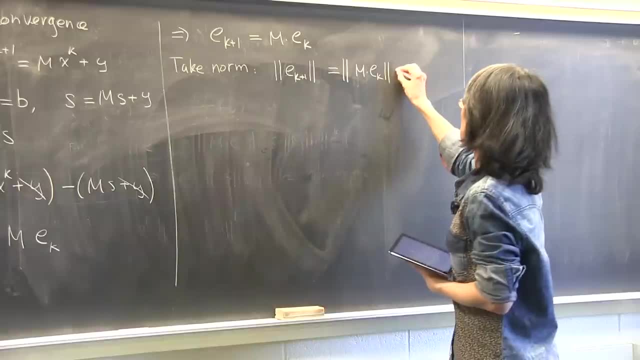 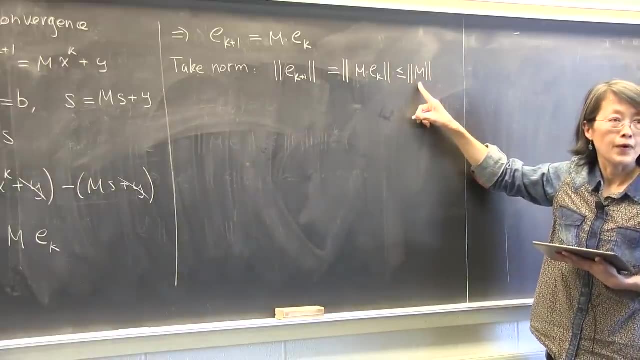 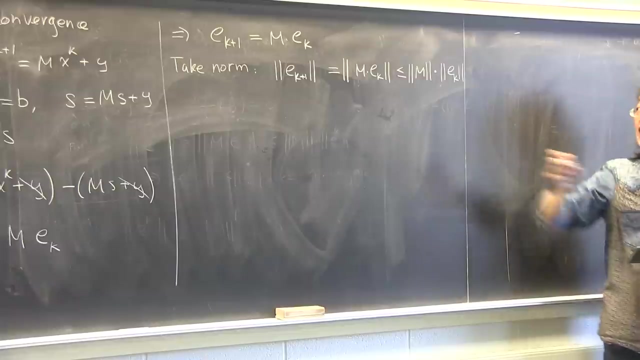 which will bound this quantity. We have used this inequality many times, So this one is the corresponding matrix norm for M, Okay, Corresponding to the vector norm you use, And that's the vector norm for arrow, And this is less than or equal to, by definition. 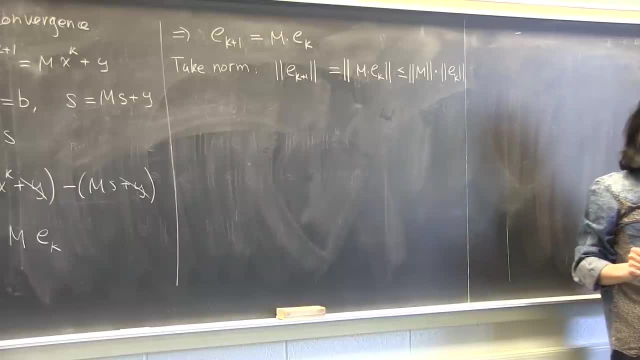 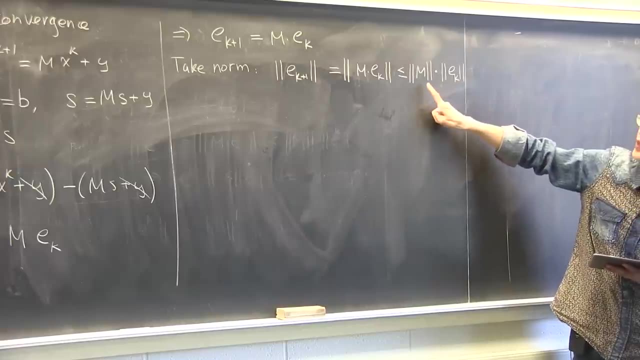 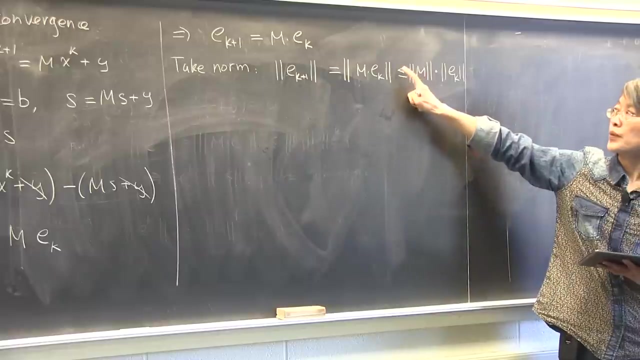 because that's the maximum, Is that okay? So what do we have? We know, the arrow measured in step K in norm, multiplied by this norm here bounds the arrow in the next step. Okay, Pay attention, This is a less than or equal sign. 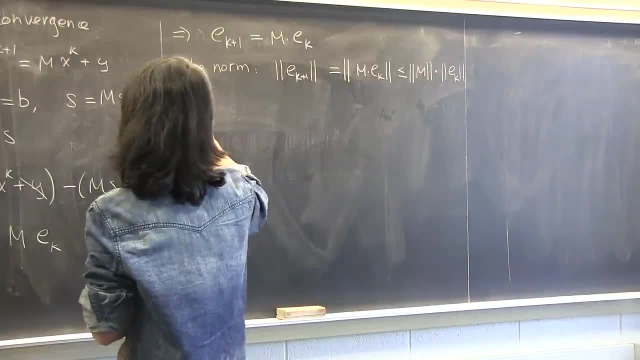 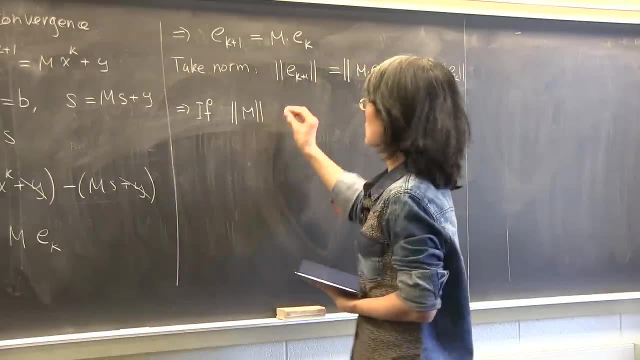 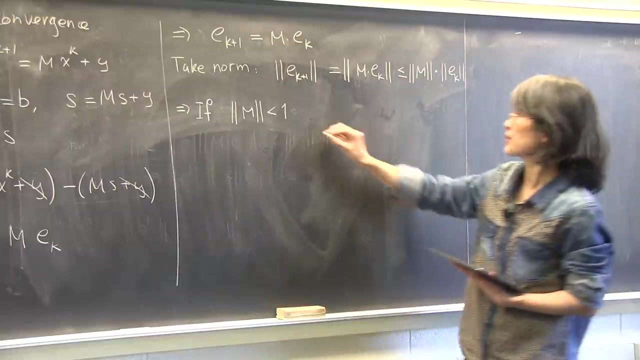 So you can have the following conclusion immediately. You see that if now I know, by some computation I figured out that this norm here is strictly less than 1. If I have that, then I'm in a very good position, Am I? What does that imply? 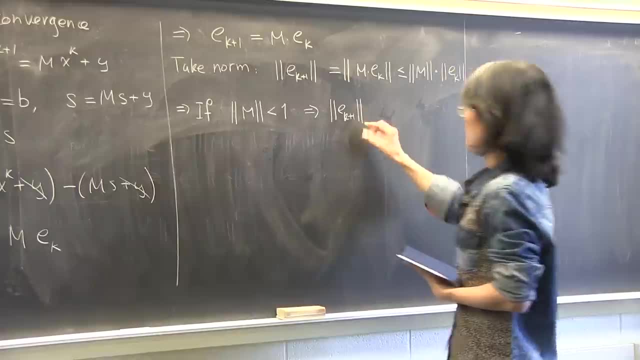 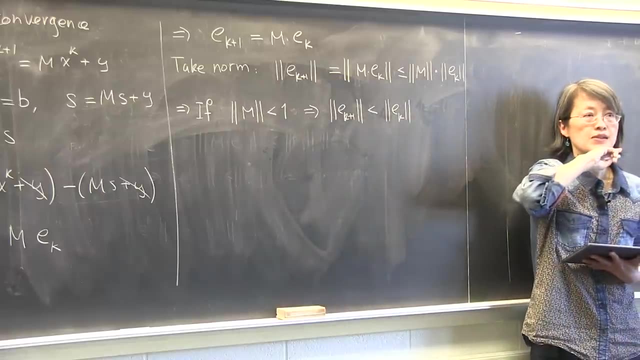 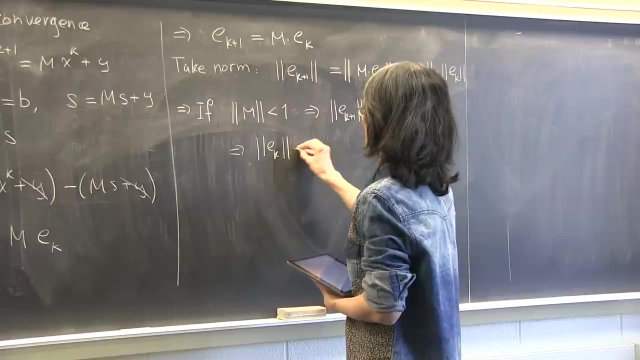 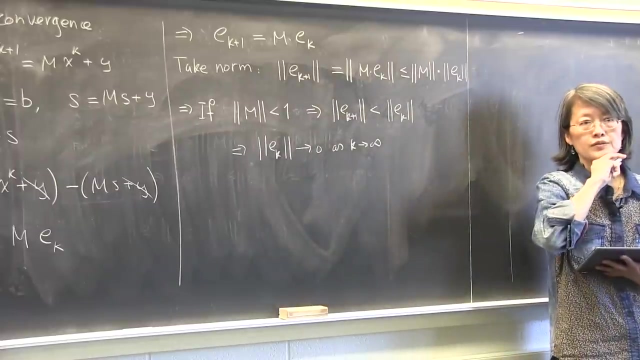 Your arrow measured at that norm will be strictly decreasing after each iteration, Is that right? And then you can conclude that the arrow K measured in that norm has to go to 0, as K goes to infinity because it's strictly decreasing, Right? So arrow measured in the norm going to 0,. 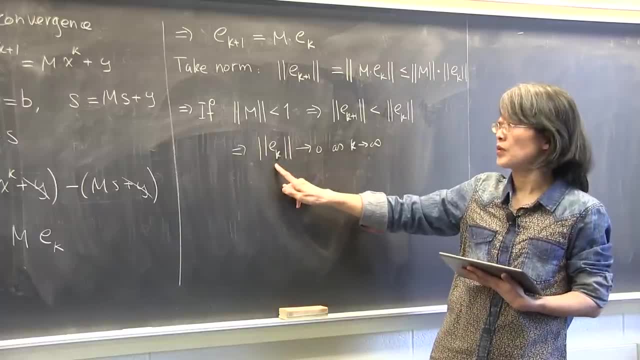 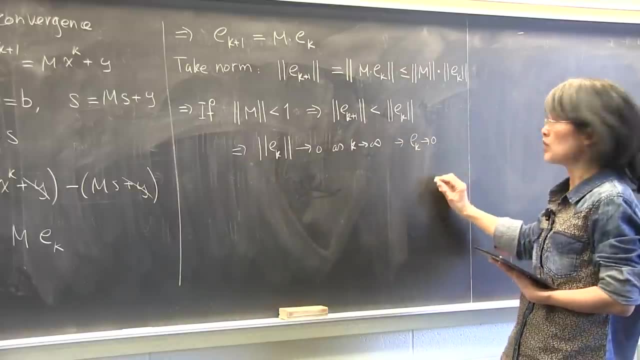 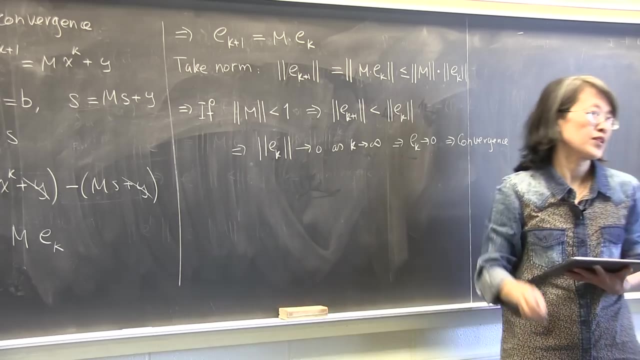 what does it mean? If the norm is 0, that has to be a 0 vector Right. So that means E goes to 0 as well And that implies convergence. Is that okay? So if this, you have convergence. 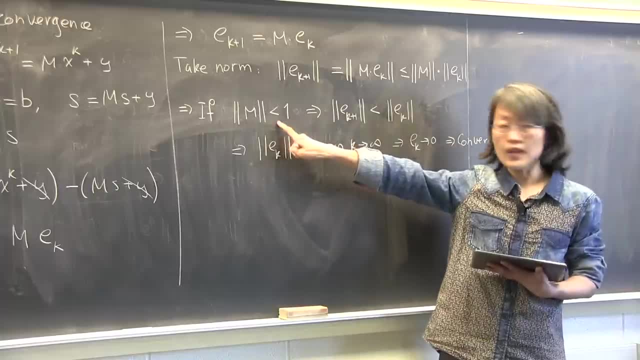 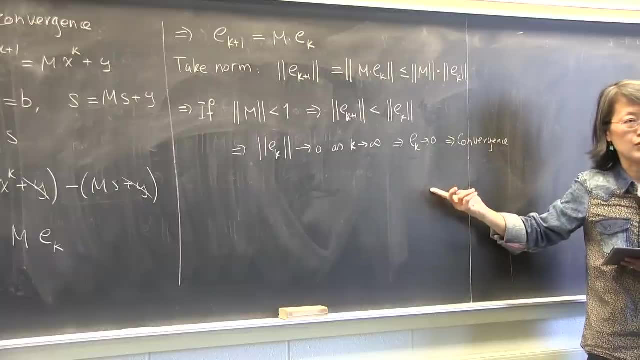 So it's a one-sided argument. Okay, If you don't have that, it does not mean it doesn't converge. It's just that you don't have an argument to show that it converges. It's not guaranteed. Okay, So it's a one-way argument. 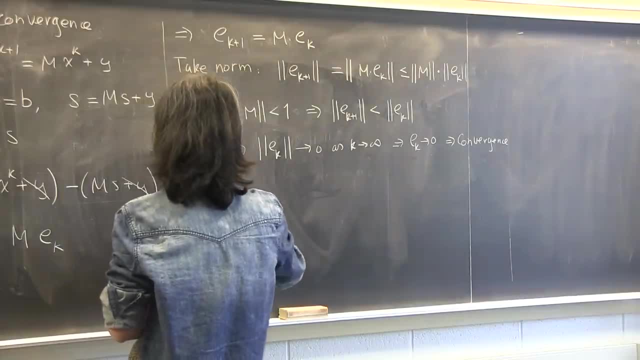 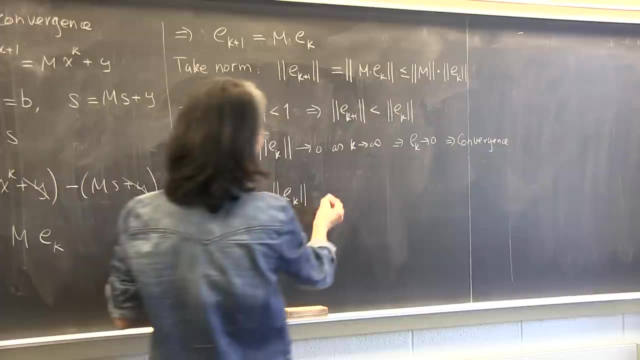 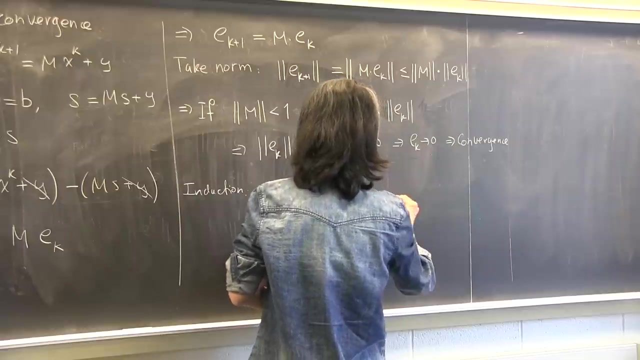 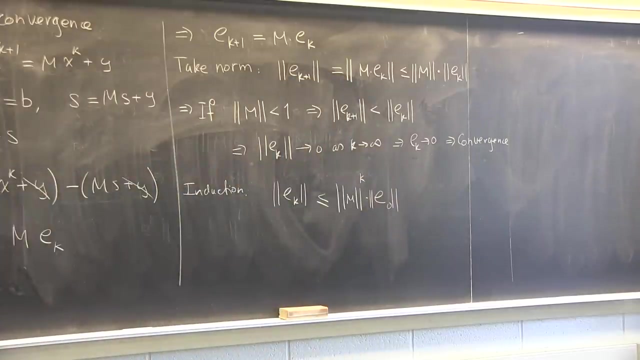 Okay, And you can easily do a simple induction To show that the arrow measured at step K shall be bounded by the m norm to the power K times the arrow measured in that norm, the initial arrow, your initial guess arrow. That's induction. so you know. 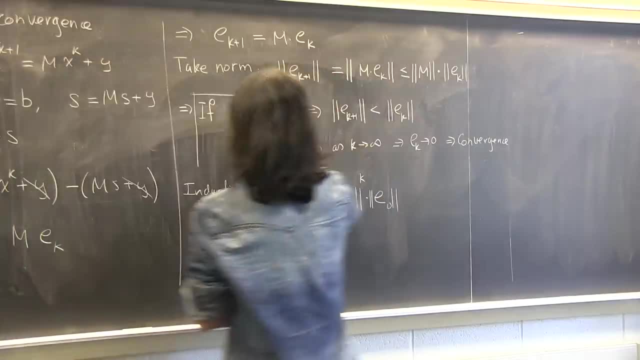 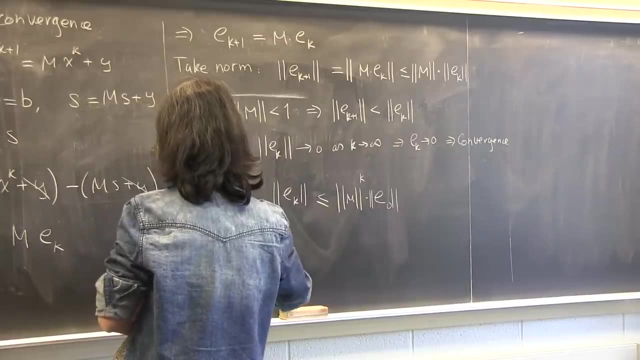 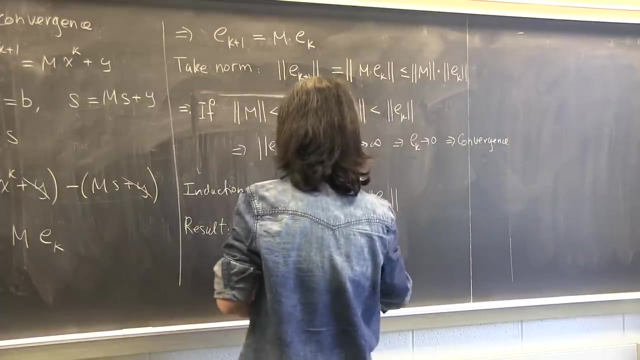 Okay, So this is the important result. Okay, let me write it again, because I have so many steps. So here is your result. Or a theorem, whatever you want to call: If m strictly less than 1,, then it converges. 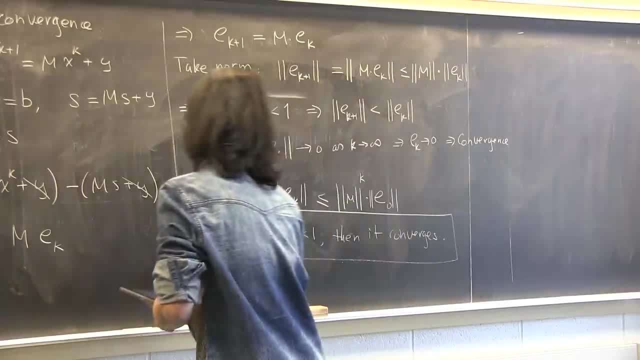 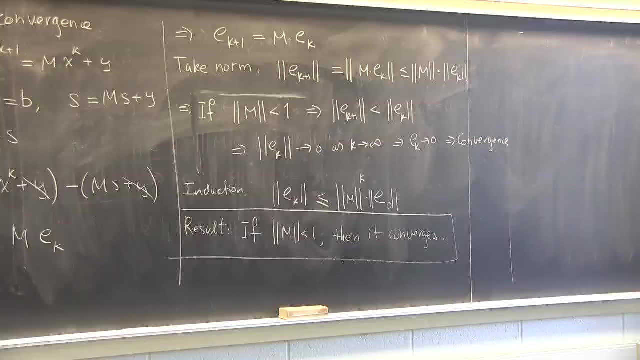 Okay, so that's your result. So you see only that matrix M matters here in this analysis. That vector B, no, the vector Y, there it doesn't matter. Okay, The iteration matrix is much more important. Okay, Are we okay? 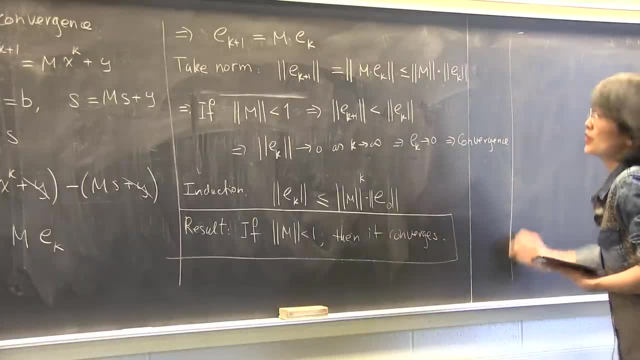 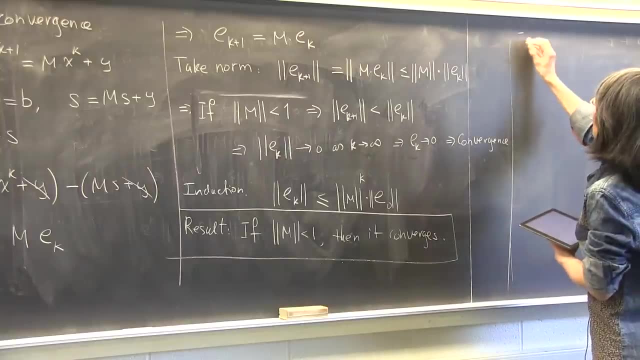 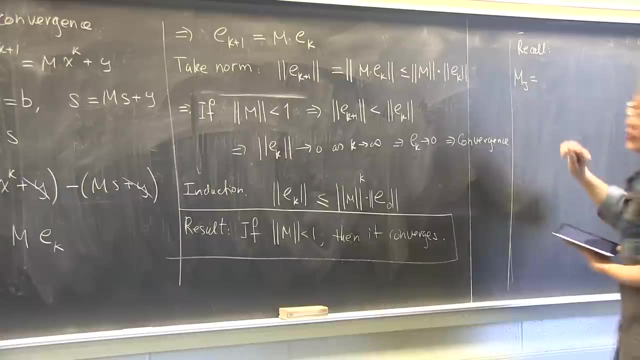 It's not bad, hm. Okay, Now we'll go back to our example. So remember, recall what we did earlier with Jacobi and J. We derived this last time, So let me write it: It's negative D inverse times L plus U. 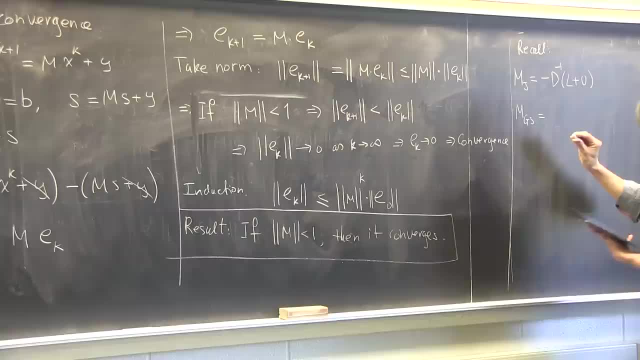 And the M on Gauss-Seidel we derived last time as D minus L, inverse times U And the SOR we just derived today, which is over there. So you see, for Jacobi and Gauss-Seidel, once the A matrix is given. 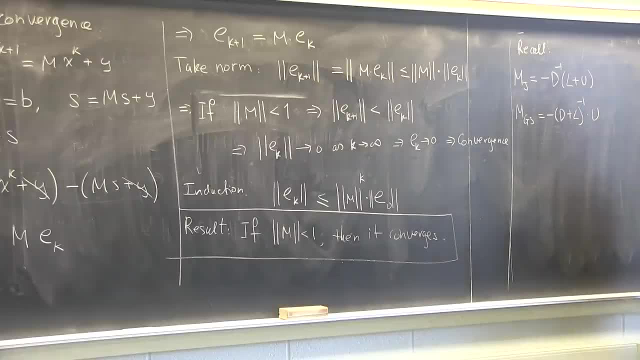 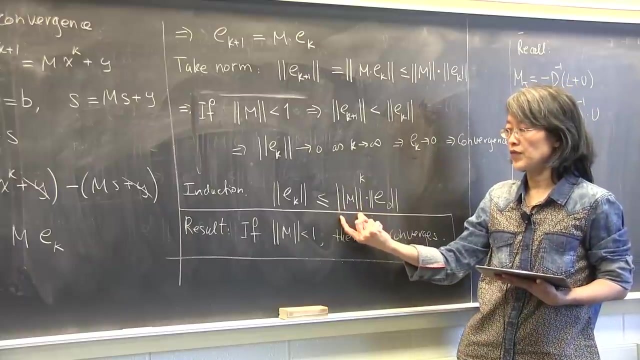 then this matrix is given the iteration matrix And then the convergence is determined. But in the SOR there's a parameter omega right. Give you some room. You can choose it in a way that to make the L2 norm of this matrix. 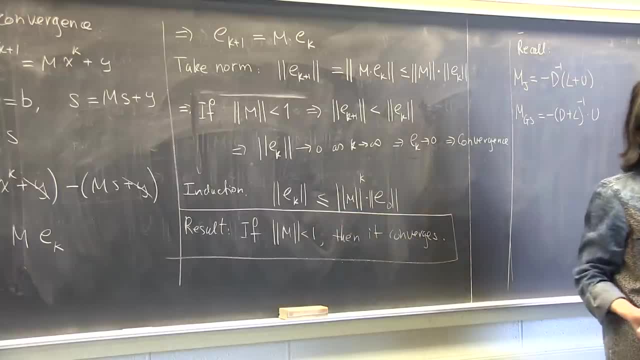 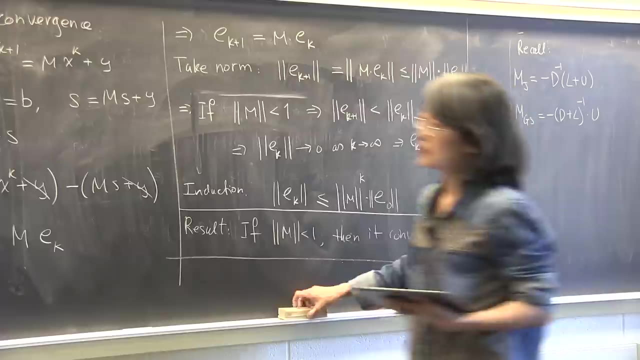 as small as possible, for example. if that's your choice, Then you know it converges faster. Is that okay? Mm-hmm, Okay. So we'll take this example, The same one as we have been using. Let me start over here. 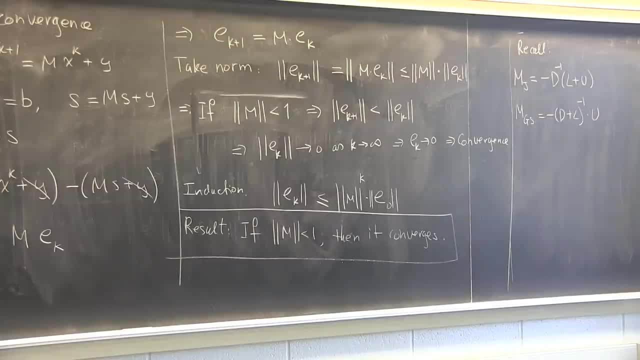 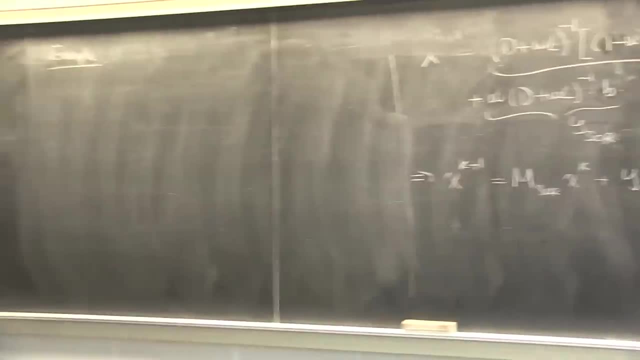 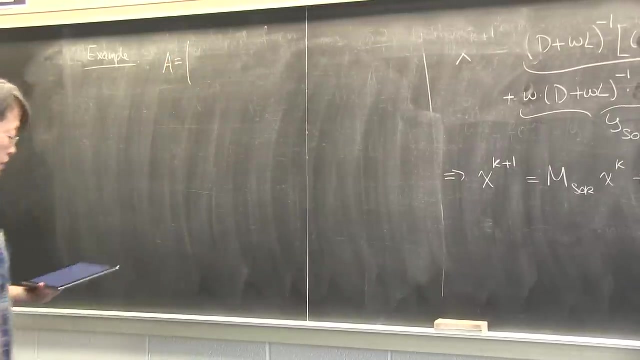 Just to put in numbers and to be convinced. So let's go back and look at that example that we have been using for all three methods And then let's check the matrix M and to be convinced that the convergence is as we are claiming it will be. 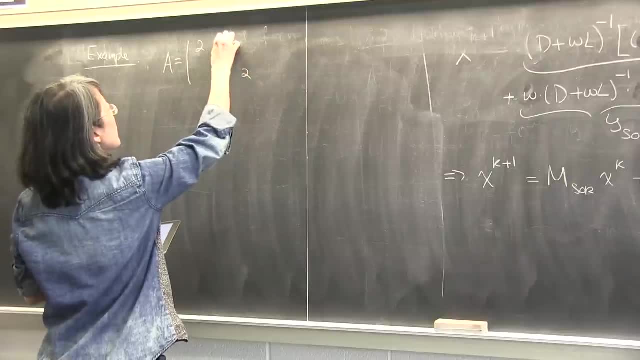 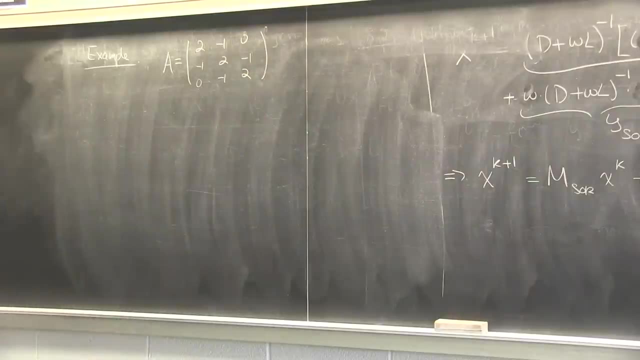 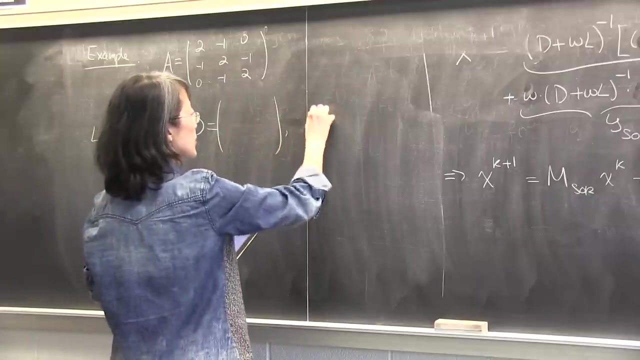 So the A is a tri kind of a tri-diagonal diagonal dominant right. It's only 3 by 3.. It's very small, Okay, And our splitting will give us three matrices: L and D, And I'll have a U matrix. 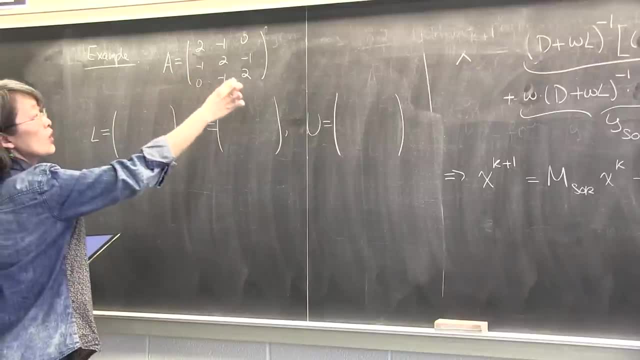 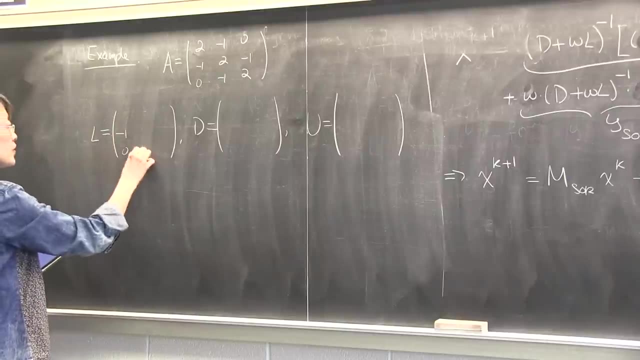 So the L matrix, what would that be? Well, they'll be taking the lower triangular part of A right And fill the rest with 0. So if you do negative 1, 0,, negative 1, that's the part you take from A. 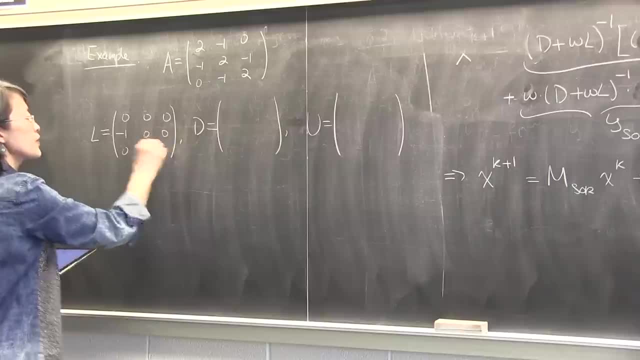 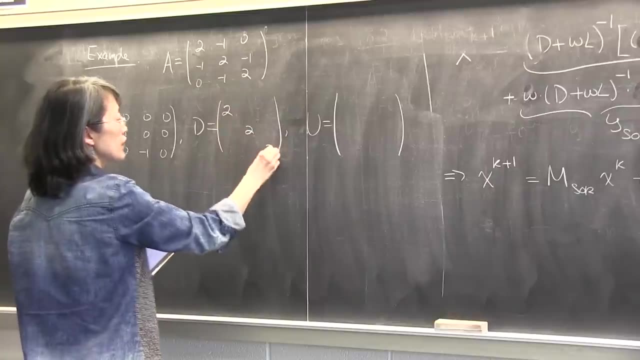 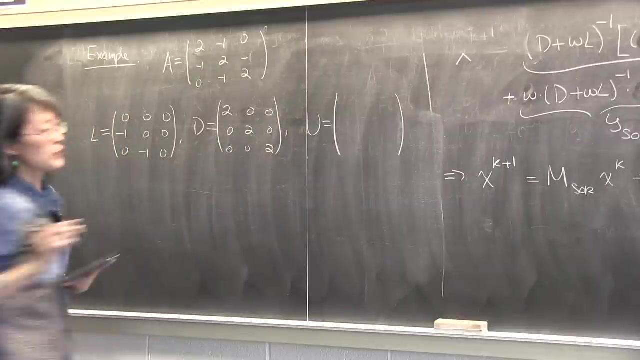 and then you fill the rest with 0. That's your L, Is that okay? And then the D will be taking the diagonal and then fill the rest with 0.. Sorry, Why do I put negative 1? That will be the D matrix. 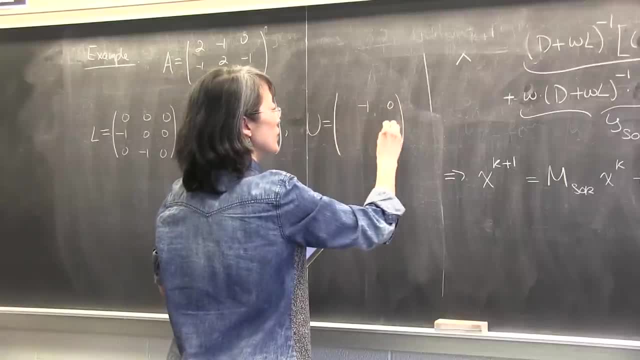 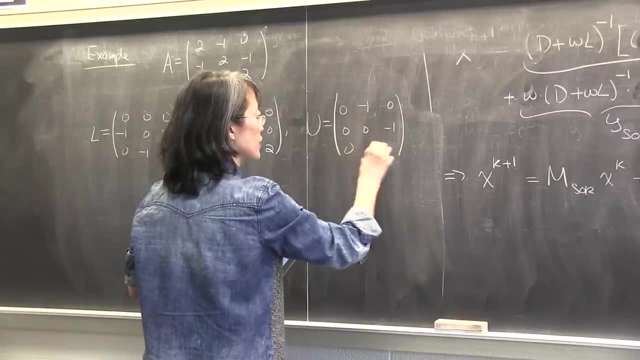 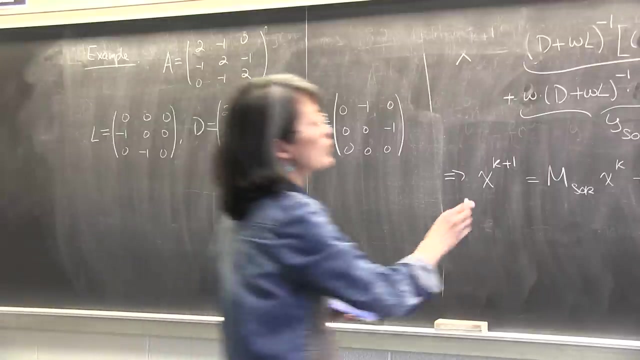 Okay, And the? U will be taking the upper triangular part from A and fill the rest with 0.. Is that okay? Okay, And then you can use these formulas: the one for Jacobi Gauss-Seidel and the one for SOR. 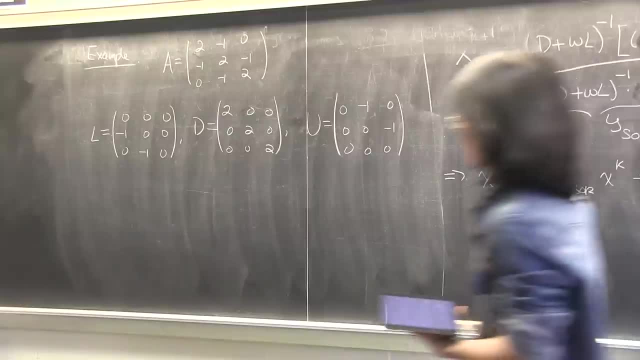 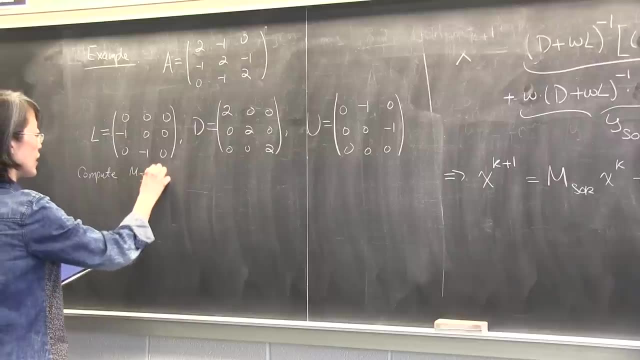 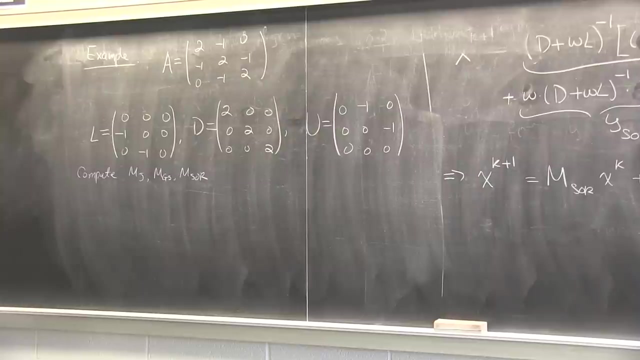 and you can find those three matrices. Okay, So you can easily compute those three matrices: M J, M Gauss-Seidel and M SOR. Do you want to see me write them out or not? Let's write them out. 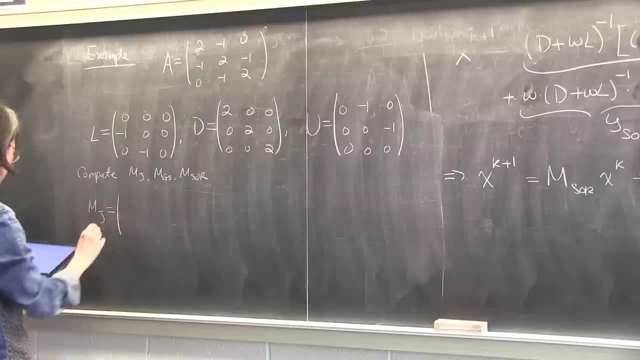 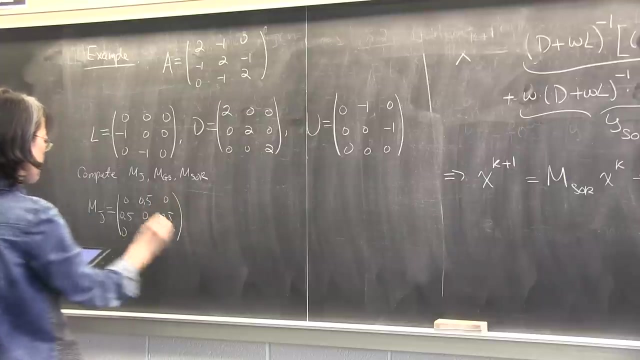 Okay, It will make much more sense the rest, if I do so. So let me write this out. So that gives me 0.50,, 0.50,, 0.50,, 0.50.. That's for Jacobi. 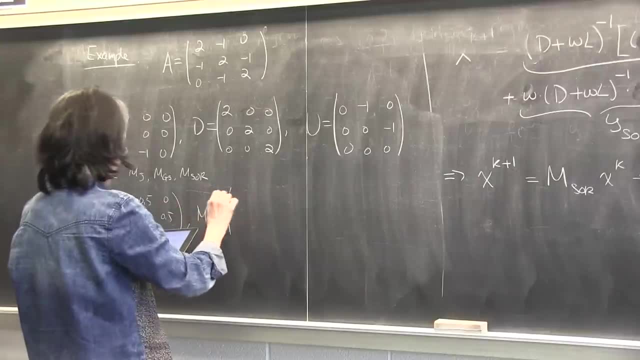 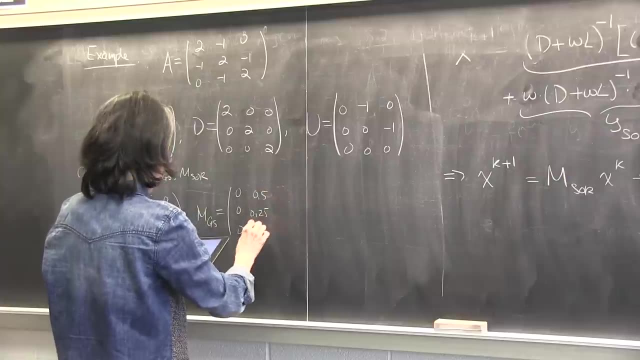 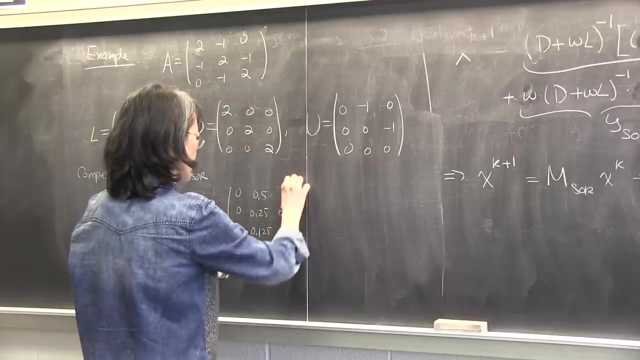 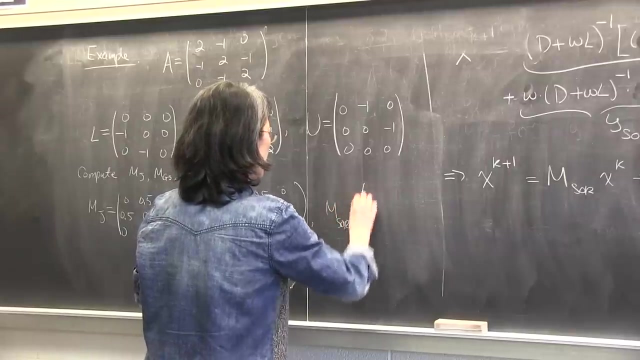 And for Gauss-Seidel I have the following: 0, 0, 0, 0.5, 0.25, 0.125.. 0.5.. zero point five, point two, five. so I mean the matrix looking at them doesn't. 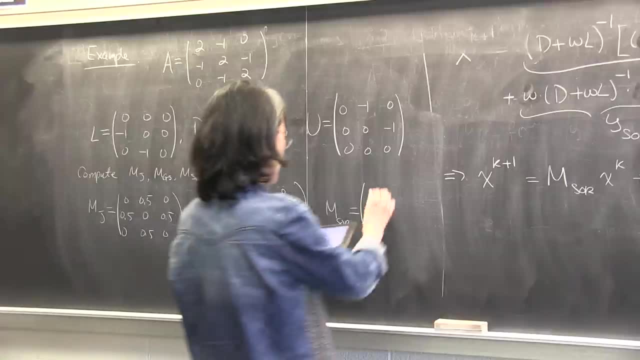 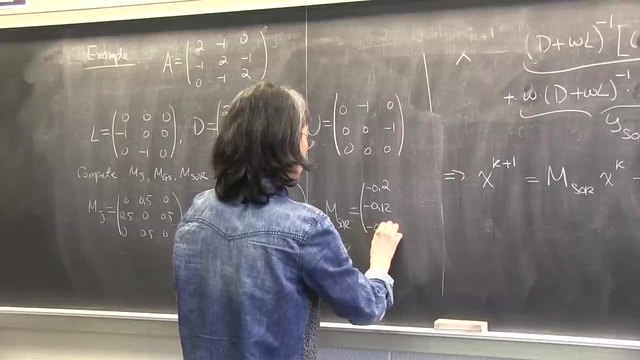 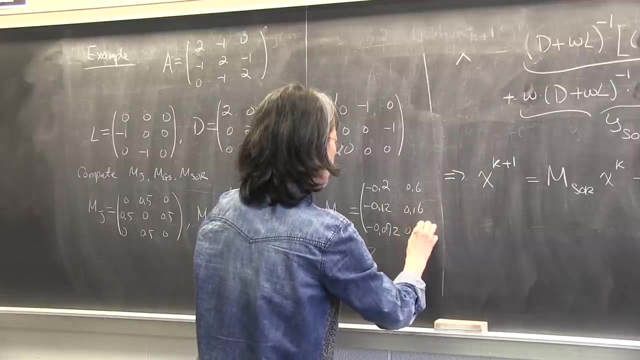 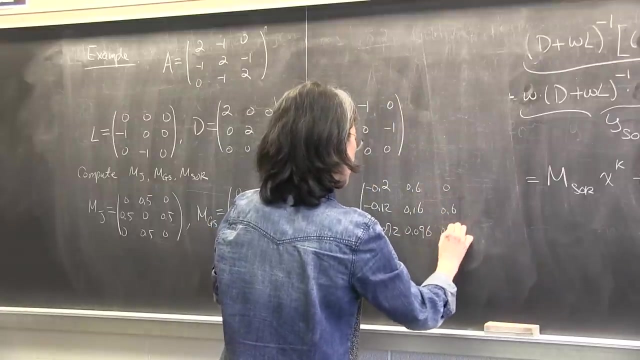 really tell you anything. you have to find their eigenvalues, their norms. then you know so: negative point two, negative point one, two. negative point seven, two and 0.6 point one six. point zero, nine, six and the last ones: zero point six, point one six. so those are the three matrices, just just computed with the 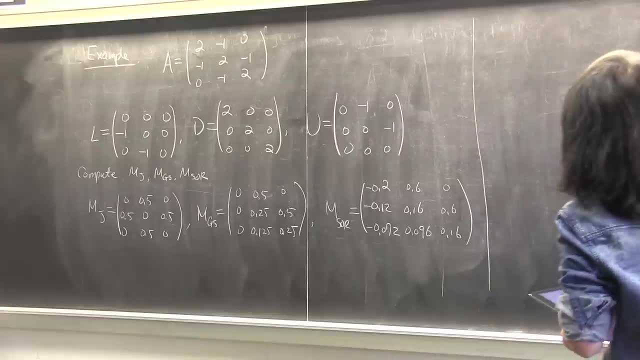 expression that we have derived and then we see they actually take those values. okay, and it's a three by three matrix. you can even call it a three by three matrix. and it's a three by three matrix you can easily give. give it to MATLAB and asked MATLAB to compute the norm. okay, so we'll. 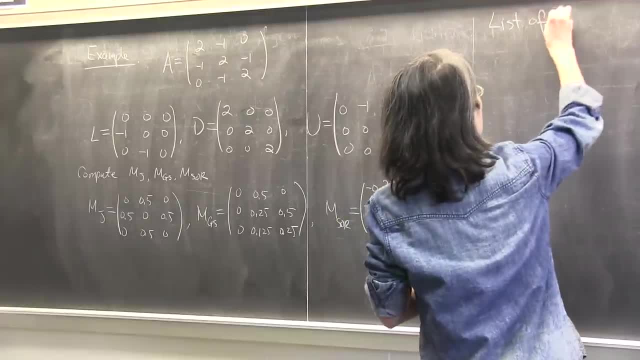 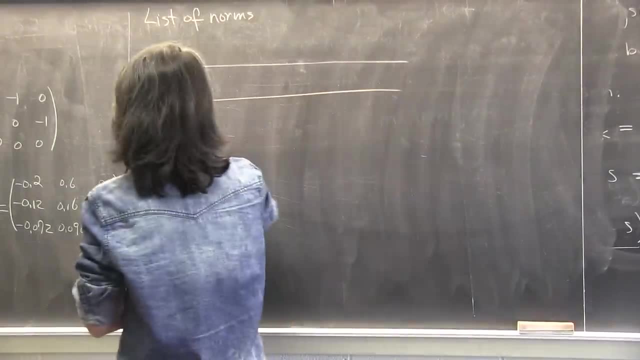 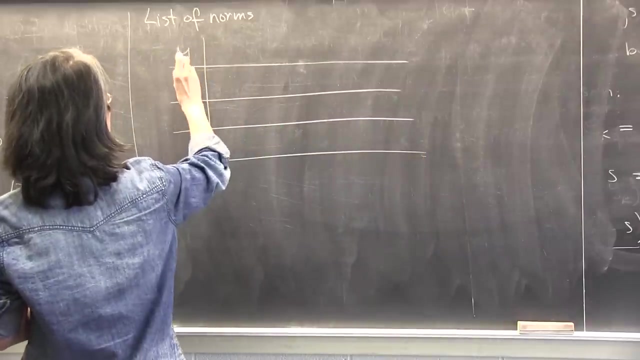 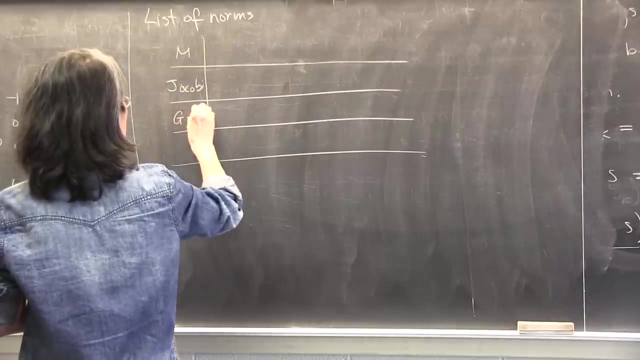 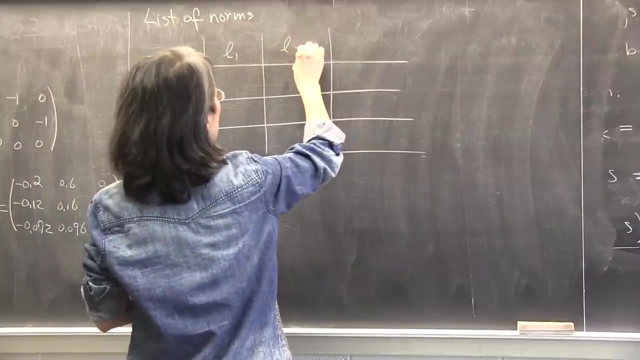 list the norms here of all these three and in three different norms and see what happens to them. okay, so here will be your matrix, different matrix. so that's Jacobi um, Jacobi Gauss-Seidel and that's SOR, And then I will put in L1, L2, L, infinity norm, the three. 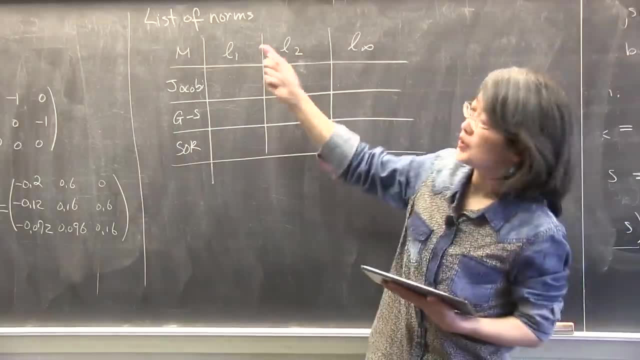 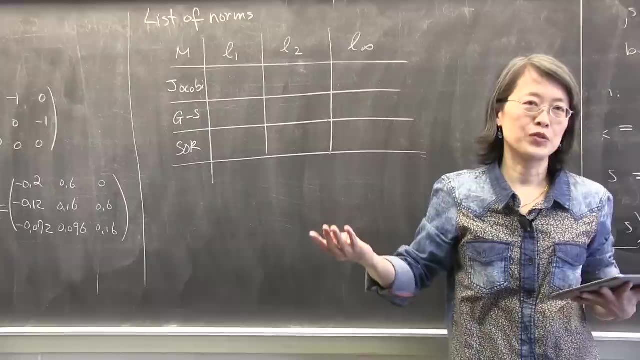 norms that we know. So anyone remembers how to compute the L1 norm of a matrix? Do we still remember I gave it to you without proof. Yeah, one tell me. Yeah, it's the max over j of the sum of the. 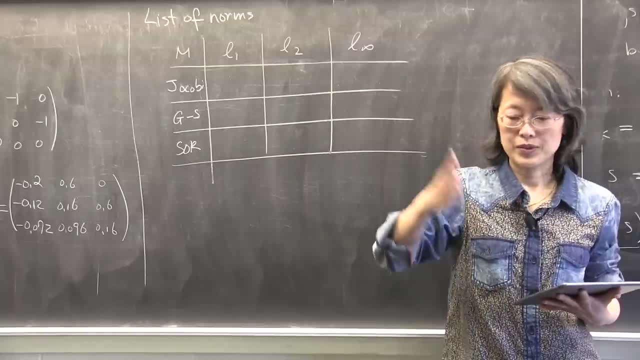 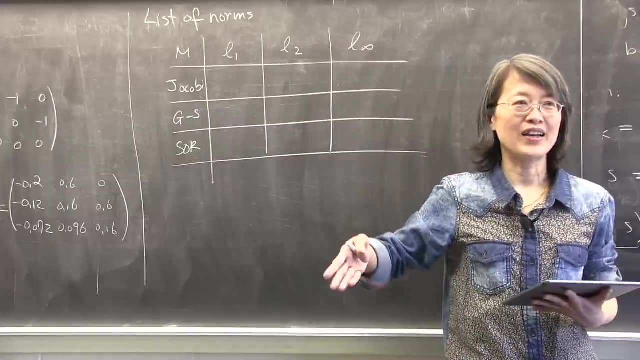 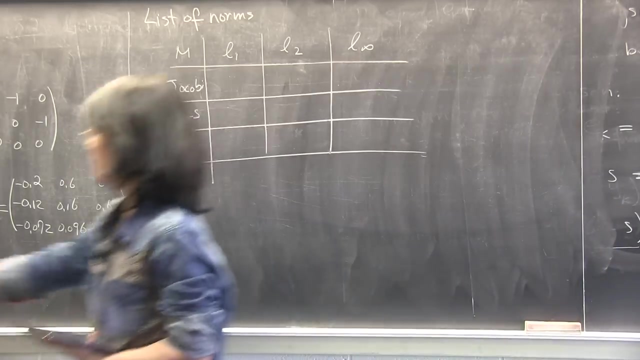 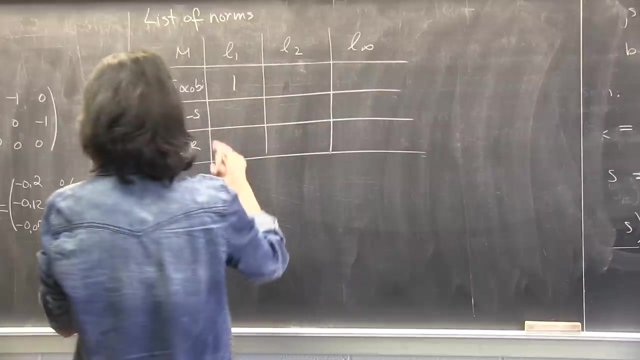 absolute value of aij, Which means you add up each column in absolute value and choose the largest sum among three of them. So you can see, if you add these up, the large one will be 1.. So I will not do all of them, I'll just give you the number. 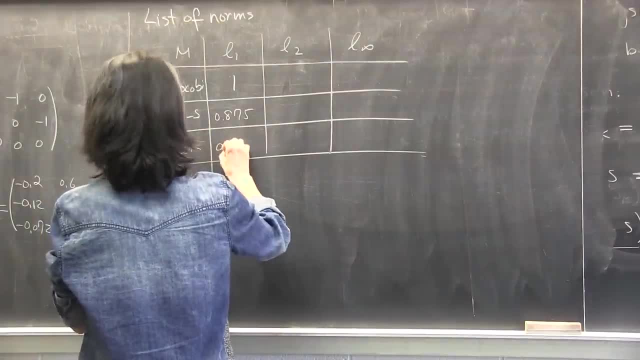 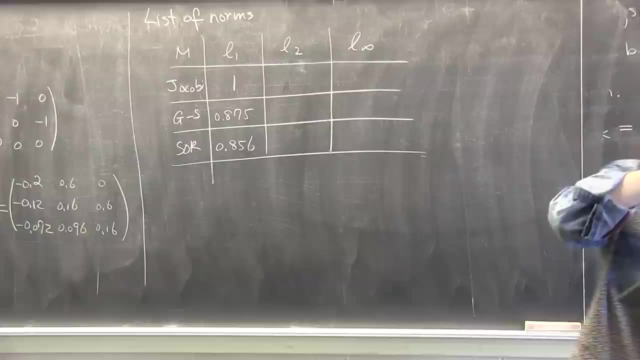 That's 1,, that's 0.875,, that's 0.856.. The L2 norm, what would that be? That's the interesting one: The largest eigenvalue In absolute Yeah, in absolute value, Yeah. 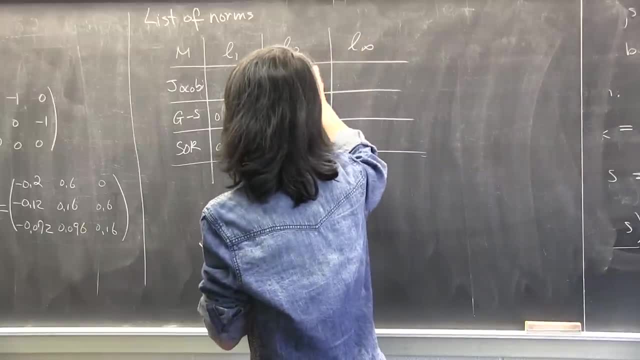 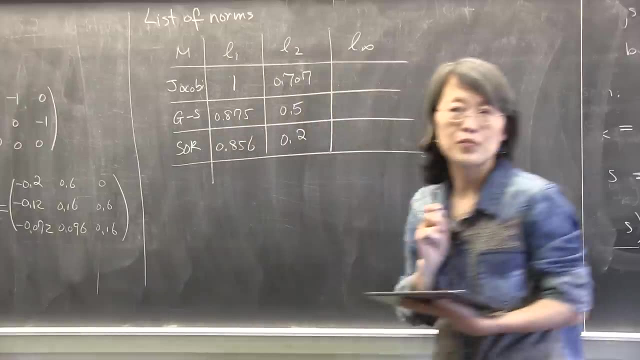 Yeah, OK, So because they're all positive, right. So the norms: 0.7.. If I, you can ask Matlab to compute the eigenvalue of this matrix and you get these numbers. What about the infinity norm, 0.7.. 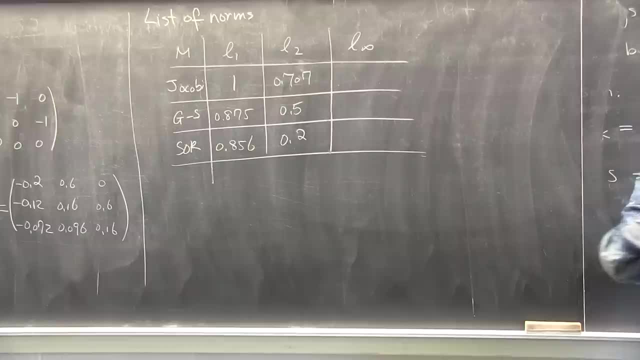 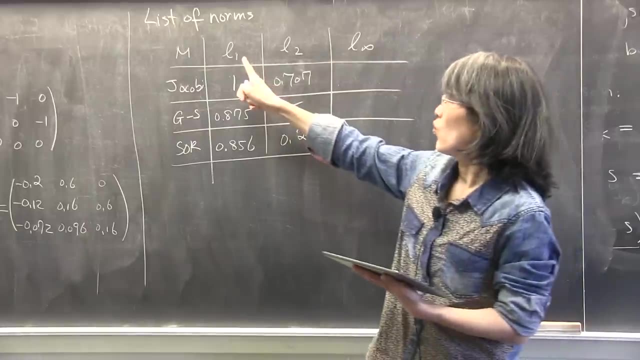 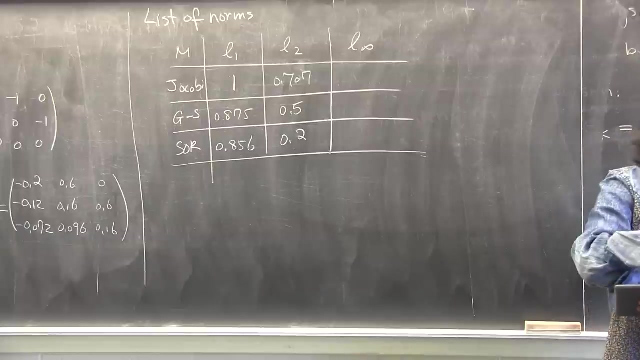 It's similar to the L1, but you reverse the order of summation and taking max right. So this is my trick of memorizing it. One looks like it's standing up right, So I take the columns first, I add up the columns and I do the max right. 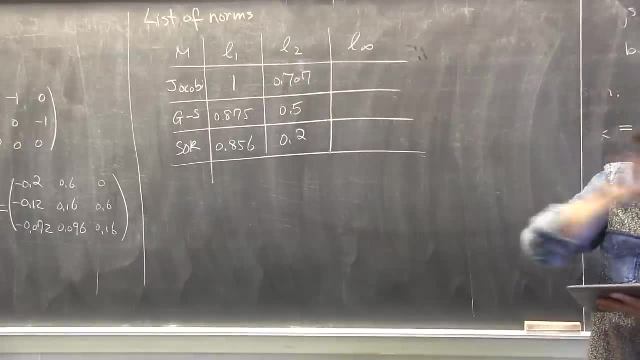 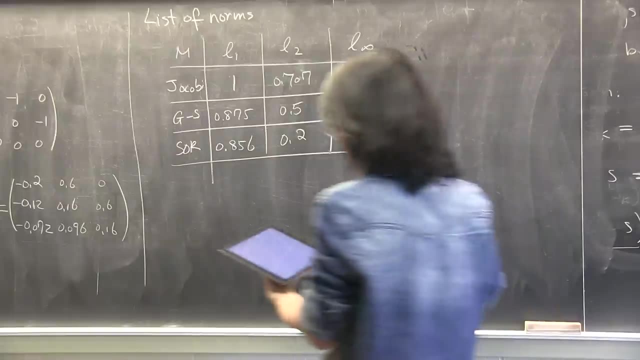 L infinity is lying flat, So I'll add up each row first and then I find the max. Does that make it easier to remember, Mm-hmm? OK, So if I do that, this give me 1.. This give me 0.75.. 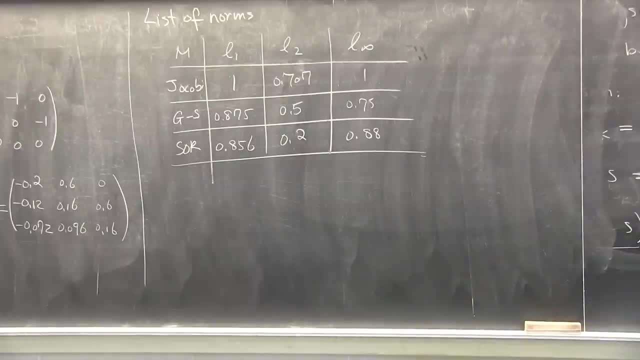 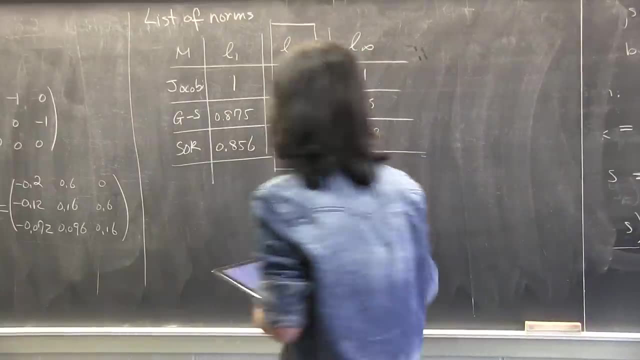 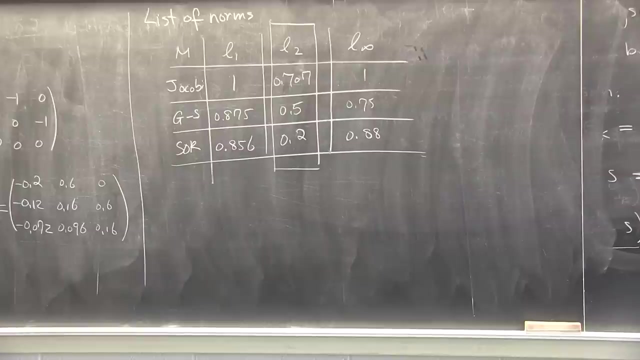 This give me 0.88.. OK, So I want to highlight the L2 norm. I'll block this. That's the interesting one here. L2 norm are the eigenvalues and they're also called spectrum radius. They have many, many other applications. 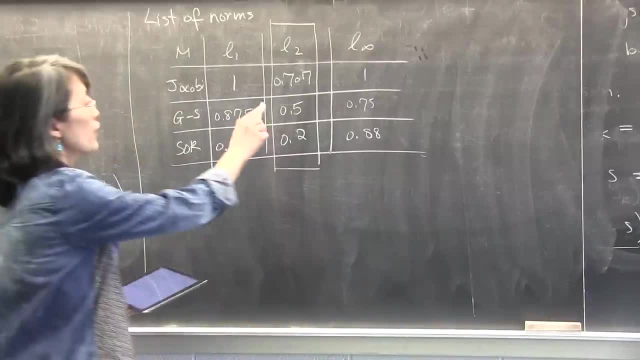 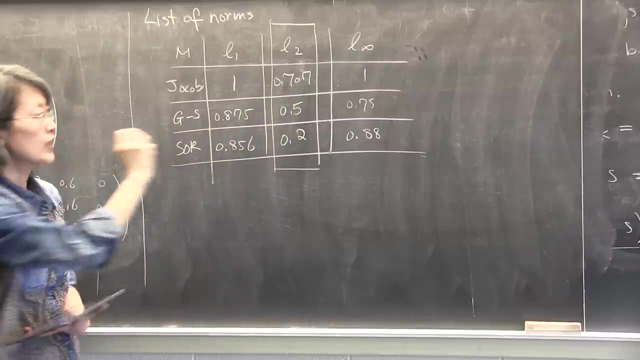 They tell you a lot about the matrix A. So you see, for Jacobi, this is 0.75.. OK, This is 0.7.. So it converges, And each time your error is guaranteed to reduce by a factor of 0.7.. 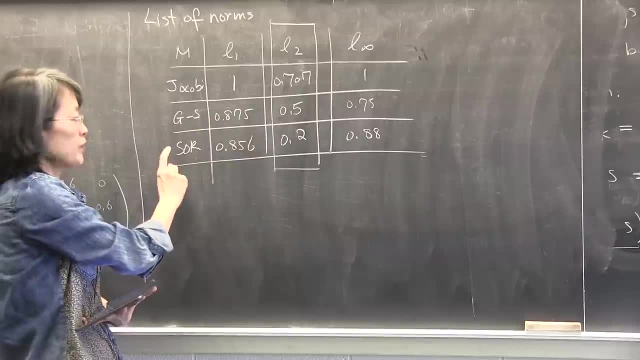 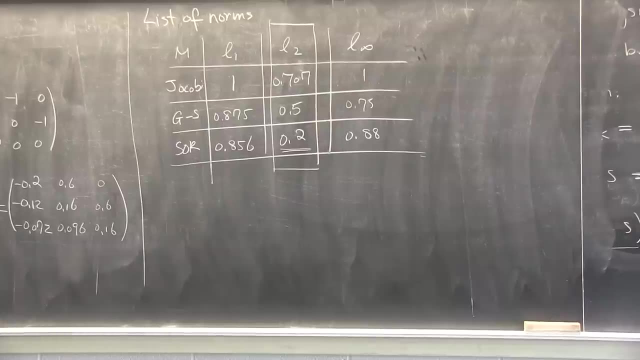 And L2 norm for the Gauss-Seidel is 0.5 and then for SOR is 0.2.. So this one is much smaller. So each time your error is reduced by a factor of 0.0, multiplied by a factor of 0.2 every. 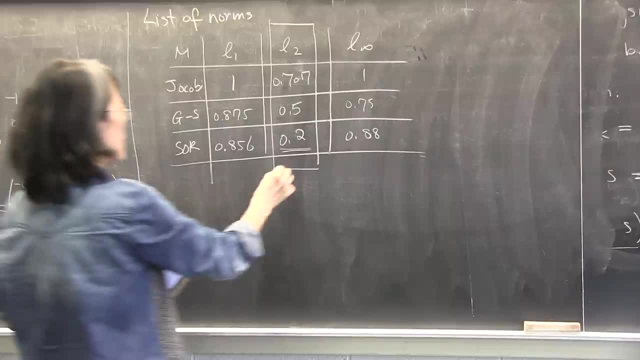 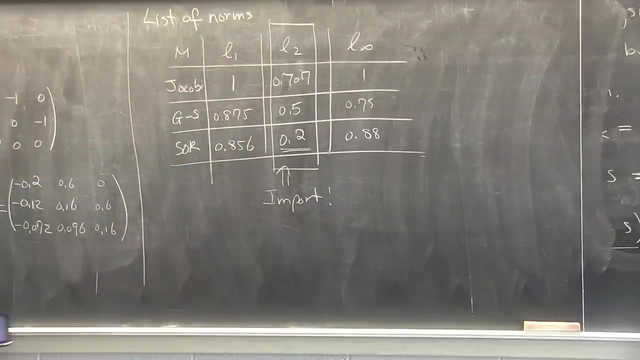 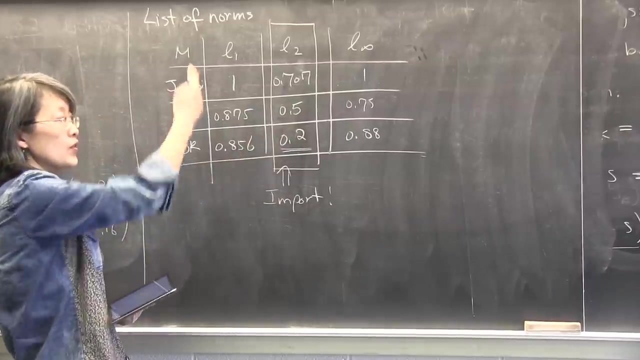 iteration. OK, So this one is the important one. OK, So if the error, if you have this and then you know that they converge in L2, then you can use that to show that they converge actually in any other norm. OK. 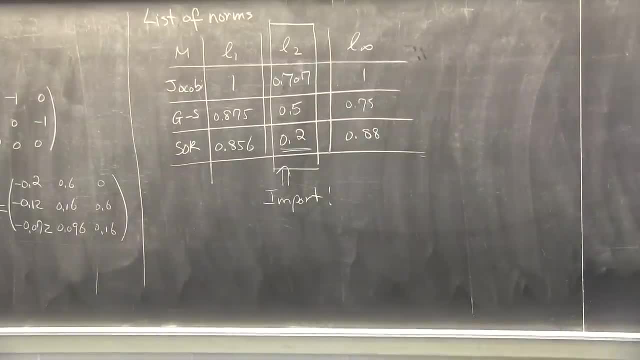 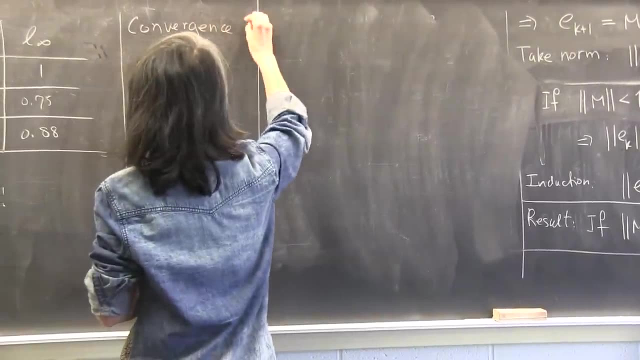 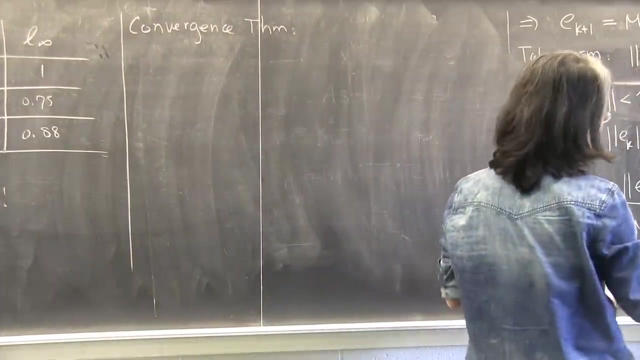 So let me give you the formal formulation of the final convergence theorem. OK, So for this example, we know, We saw that it converges. Actually, the hard thing is to show for some kind of A matrix, some norm of this M matrix. 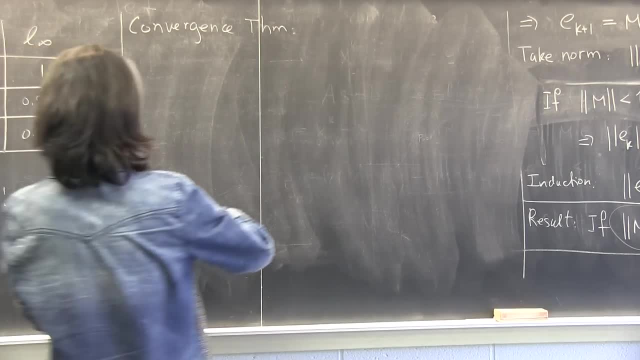 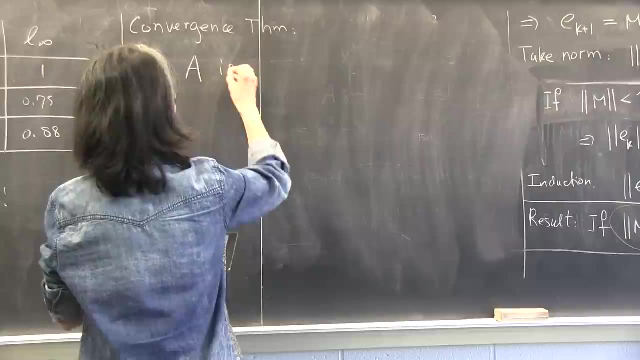 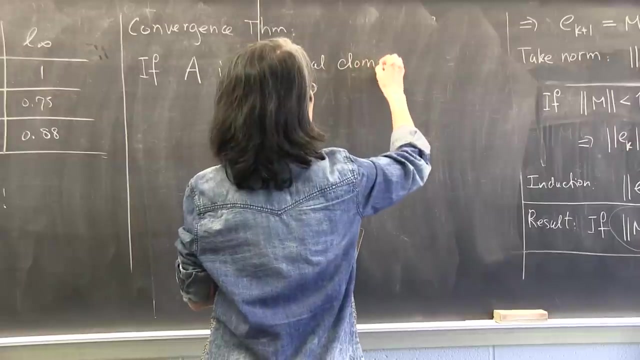 become less than 1.. Right, So I will give you this theorem without proof, because it will take a really long time. So here's the condition: If your A matrix is diagonal dominant, OK, Actually, I'm strictly diagonal dominant, I forgot. 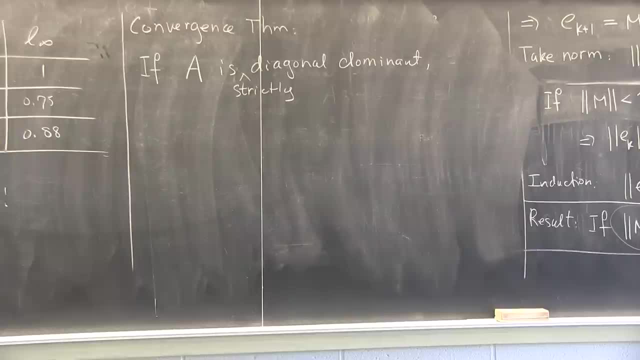 I always forgot. Do we still remember, what it means to be diagonal dominant, That the diagonal element is big. Right It's bigger than the sum of all the rest in the same line or column. OK, And those matrices are very desirable. 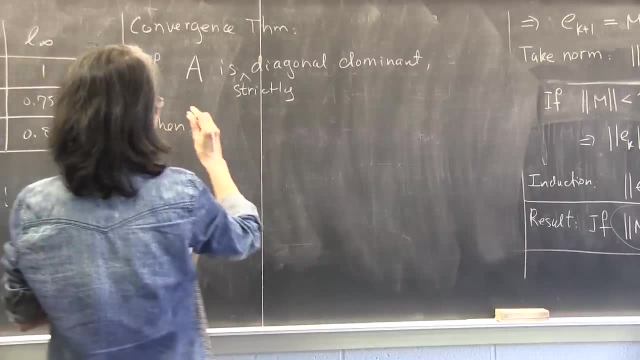 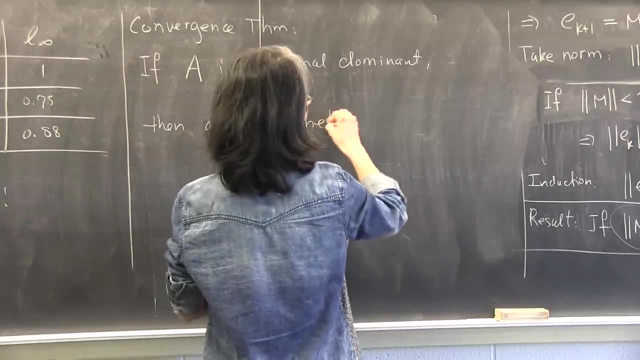 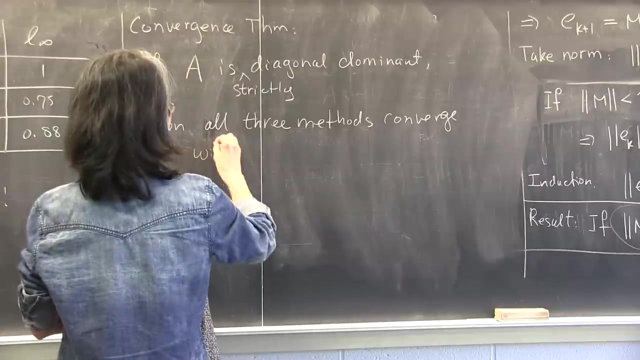 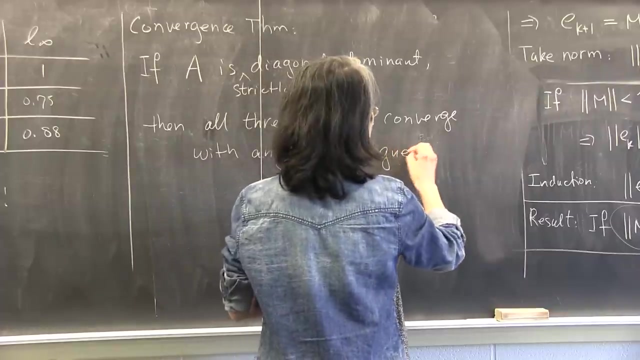 If that is the case, then you know for sure that all three, All three Of those methods, all those three iterations converge. OK, And they converge with any initial guess. So the initial guess doesn't matter, OK, As long as the arrow is decreasing. 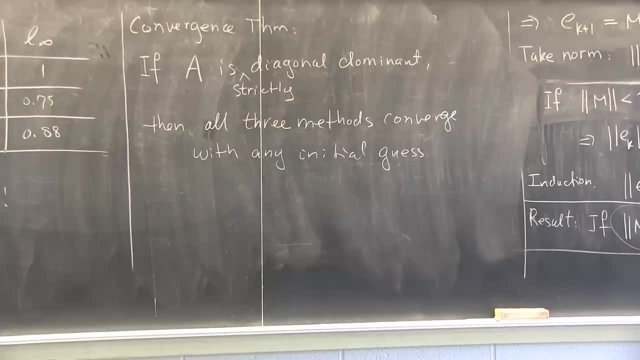 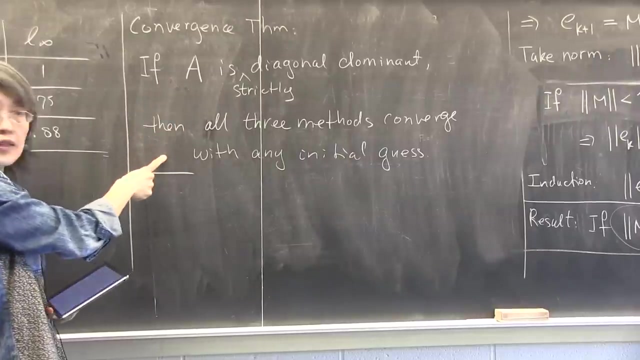 That's the term. by the end, It always converges, OK. So I want you to pay attention to the formula, The formulation of the theorem. The theorem says: if A is diagonal dominant, then it converges, OK. It doesn't say if A is not diagonal dominant, then it doesn't converge. 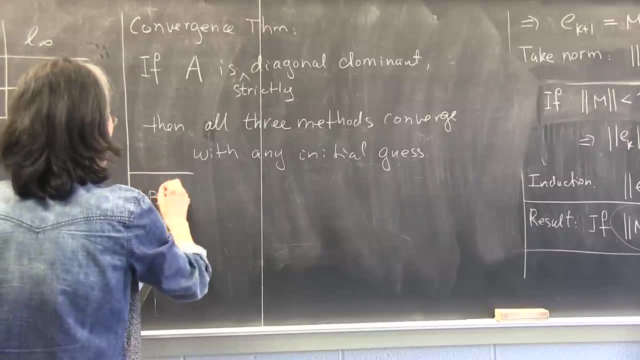 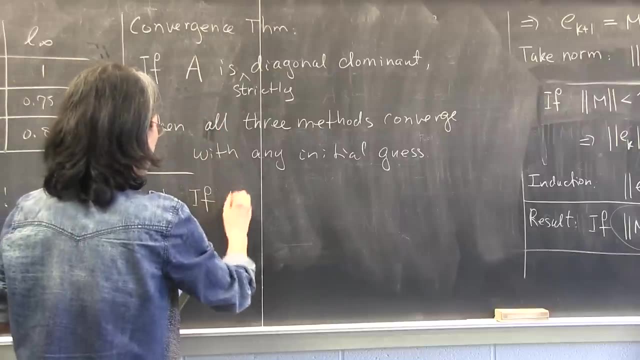 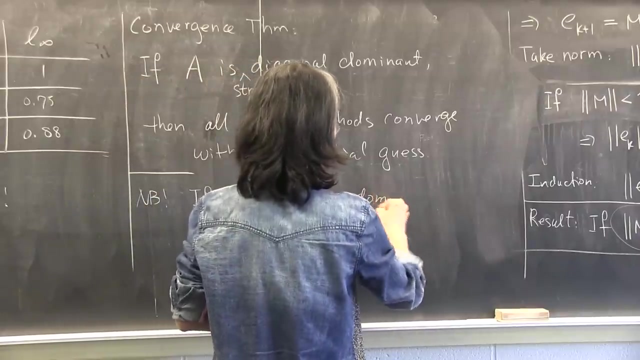 It doesn't say that. OK, So I want to catch your attention Now. that's a very desirable property, but you don't always have that Diagonal dominant. So if A is not diagonal dominant, OK, All these methods, they can still converge. 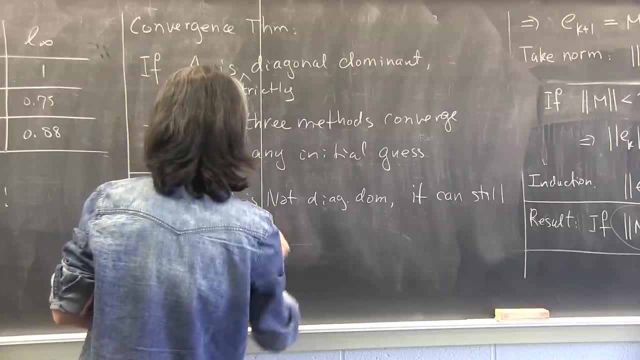 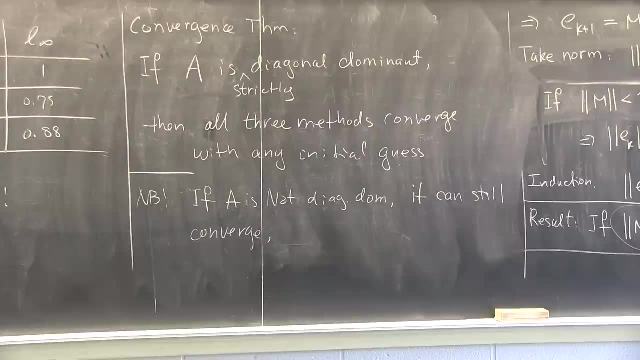 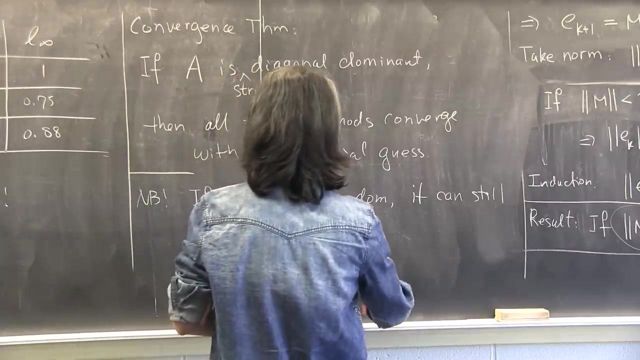 In fact we observe it in many simulations. But then just, you cannot use this theorem to have a guaranteed convergence. You have to dig out something else to show it converges. OK, So not guaranteed by this theorem. OK, Is that OK? 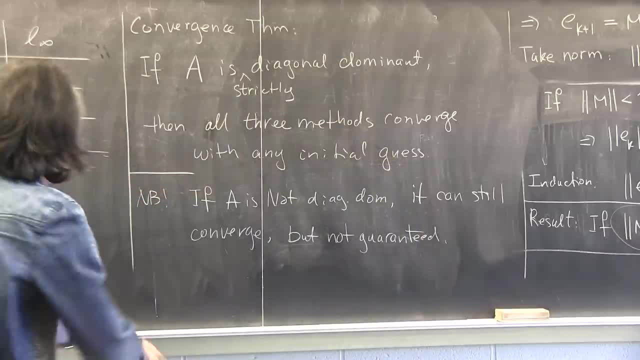 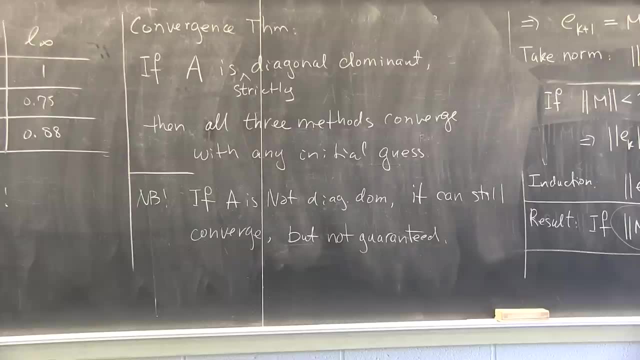 Any questions? So I. If you want a detailed proof for this theorem, then we have to dig out all linear algebras and eigenvalues, and I'm not ready to do that. Uh-huh We OK. OK, Let's see some simulations. 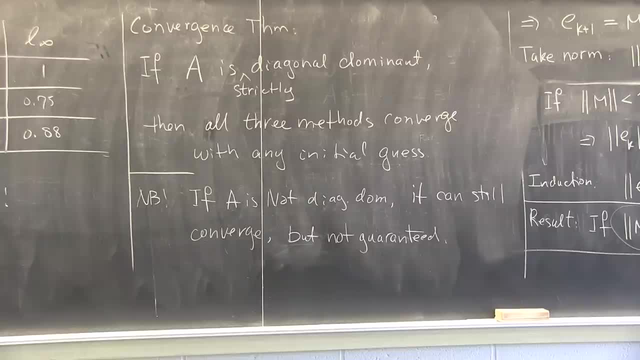 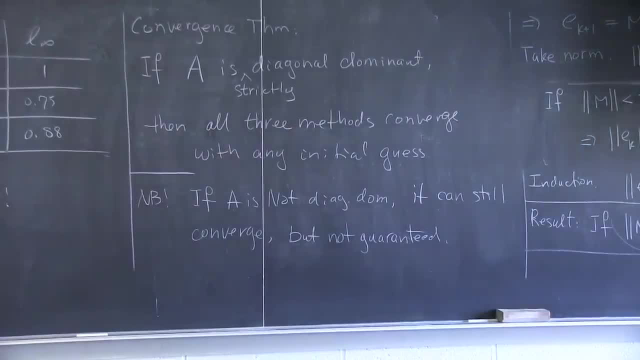 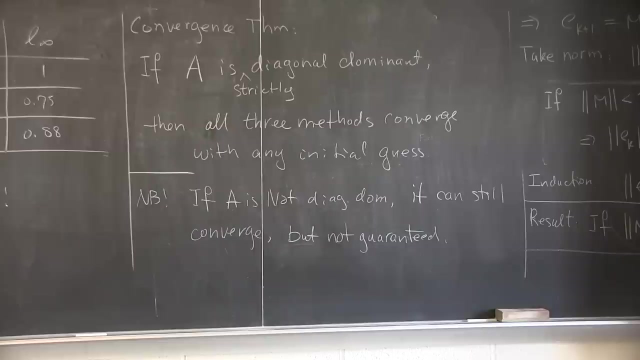 SEAT 5.. SOMEONE LOCK ME OUT. OK, I don't remember shutting that down. Okay, it shut it down. I'm sorry we have to wait a second for it to warm up. Okay, it's coming. Okay, so you have a homework problem due on Wednesday where you're supposed to use the 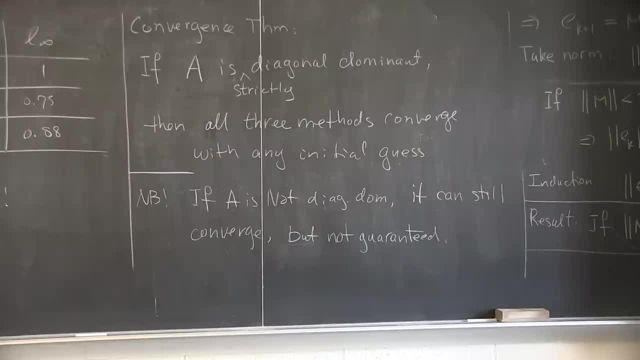 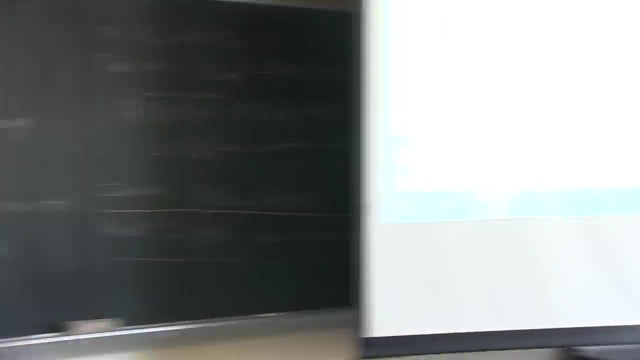 code- Naive Gaussian Elimination- which is available. you just have to download it and learn how to use it, And I give a- what do you call that mechanical construction- for you to see some applications of systems of linear equations. So, and I say that there are some, 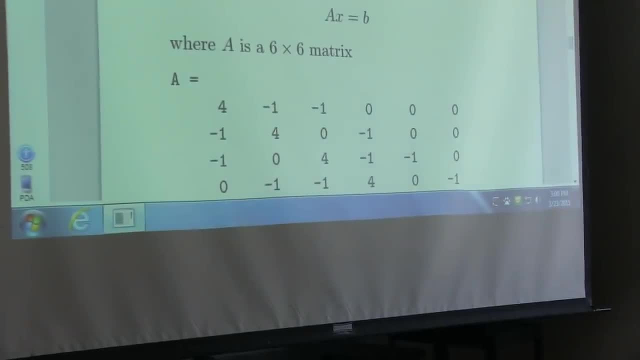 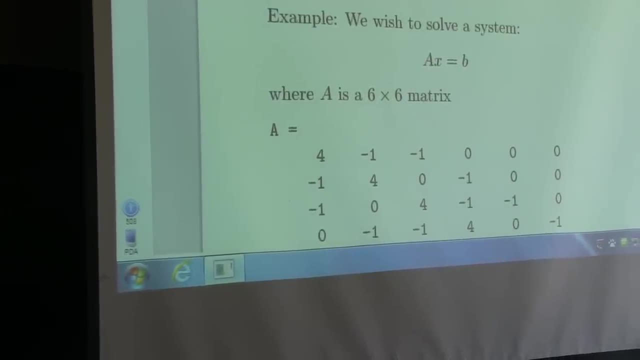 errors, mistakes, because I'm famous of making mistakes. Who is not famous of making mistakes? Who dare to say that We're all right? So you can try to find the mistakes and solve the correct system. and if you don't do that, 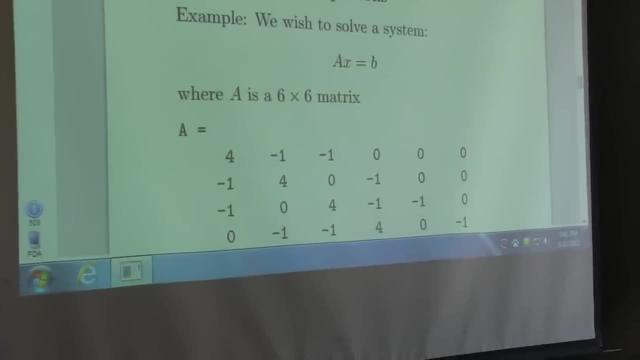 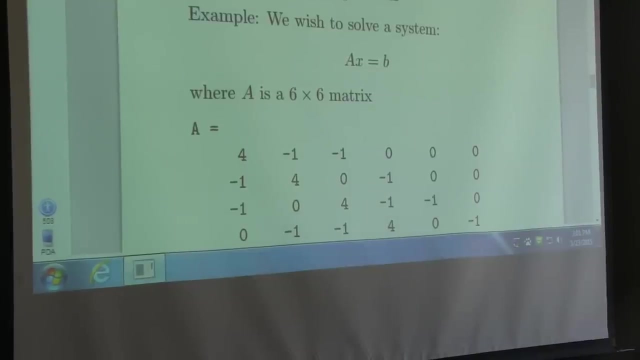 that's totally fine, because this is a course on numerical simulation. Okay, you just say I didn't find it and you can just solve the system that's provided. That is totally okay. Is that clear? Okay, All right. So what we'll be talking about is: 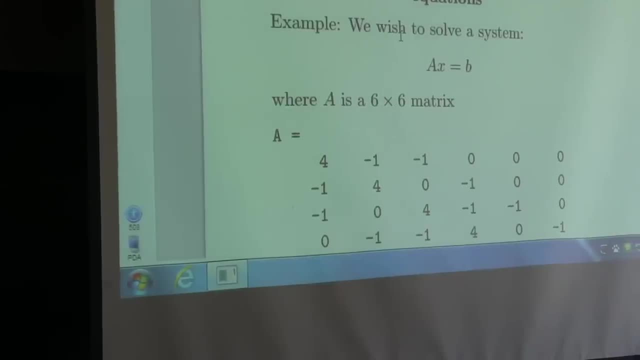 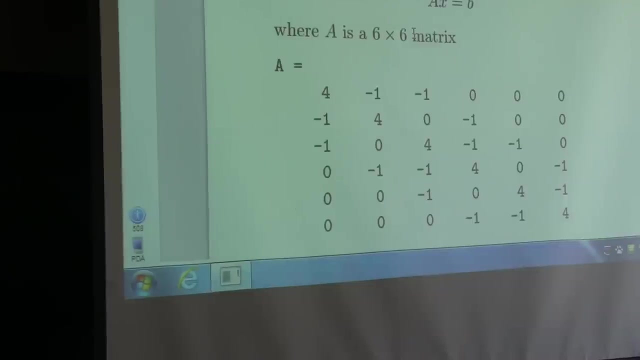 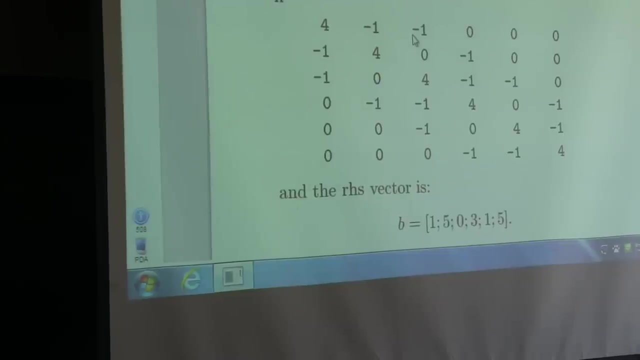 um, some iterative methods for system of equations. I just want to show you how these three methods perform in action. Okay, so we choose a system Ax equal to b, where a is a six by six matrix. and you see that it's given like that. 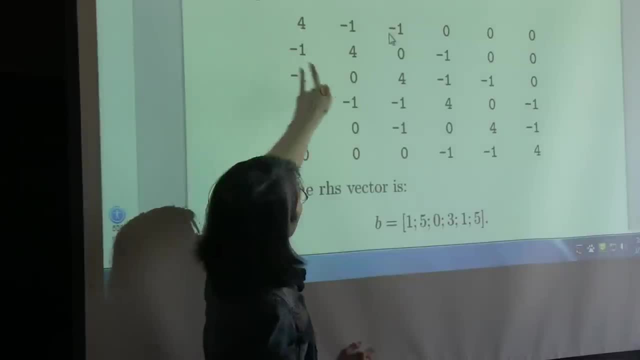 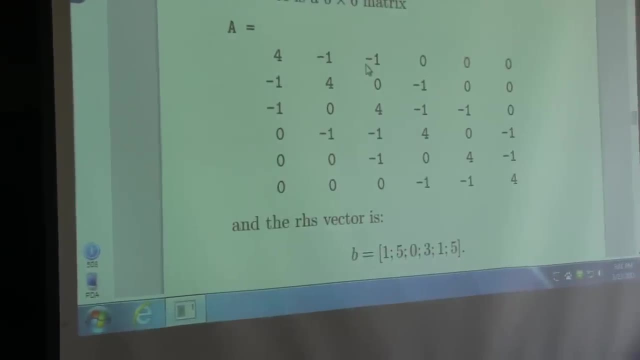 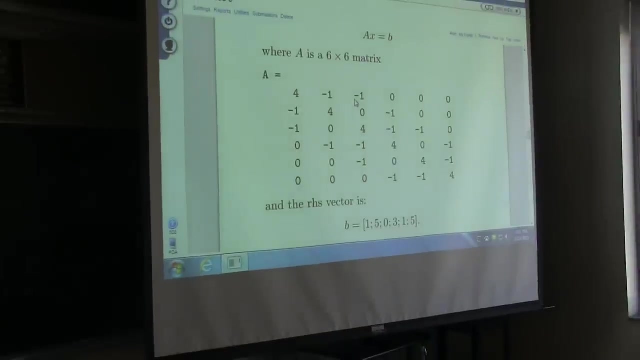 So I purposefully chose a matrix with a property. What do you think that property is? by looking at the a, It's diagonal. Yeah, the diagonal is really big, isn't it? Yeah, So we know all these methods are guaranteed to converge, right? okay, and there is a b vector. 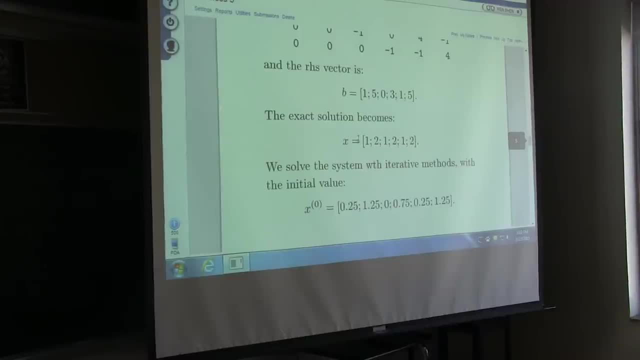 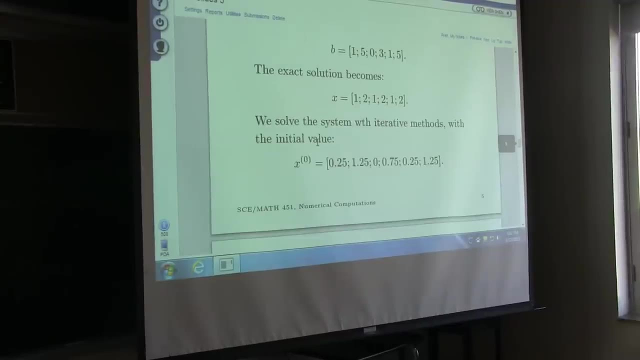 the right hand side, b is like that and the b is chosen such that the exact solution is this: factor: one two, one, two, one two. so it's easy for me to see if my iterations converge. okay, and we'll start with initial data. that is actually just the b vector divided by the 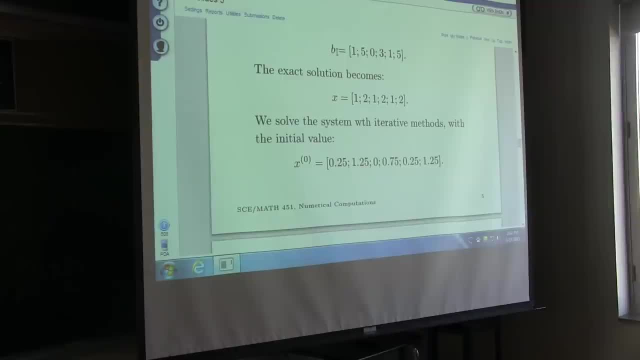 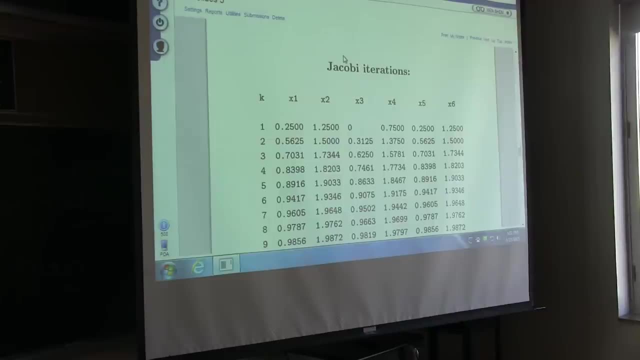 diagonal four. so it's this: x zero is just one fourth of the b. okay, Then we'll run the three methods. so, Jacobi iteration, we'll run it and then we will ask the iteration to display at every step the iteration number k and each element and it. 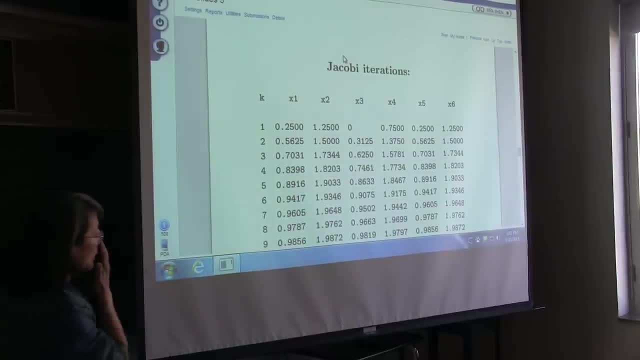 displays in four decimal places, and my stop criteria would be that your approximate solution is accurate up to four decimal places, meaning error tolerance will be ten to the negative five. Is that clear? Something like that? Okay, so, Jacobi iteration, I performed these other data, the code output for me. so after 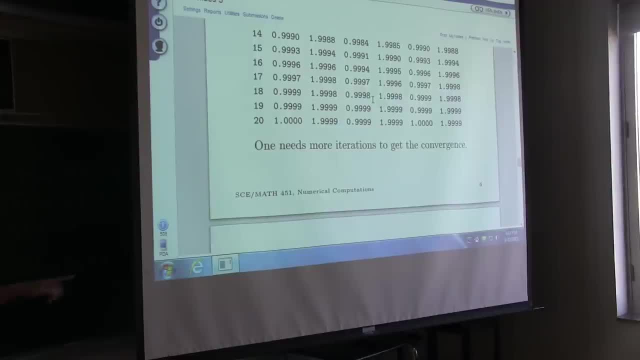 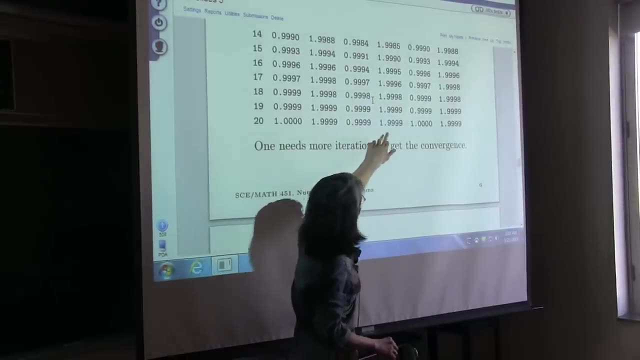 twenty iterations. I get these numbers and I see that this one is good because the answer shall be one, two, one, two, one two. but these numbers are still not good yet, but they are very close, so possibly after a couple more iterations I shall be good. okay, so about twenty? 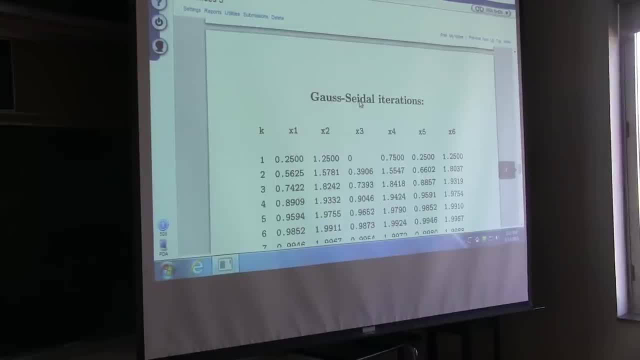 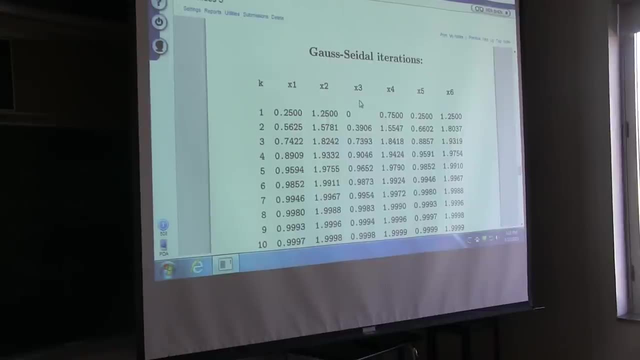 some iterations For that. okay, and then I can do the same thing with the Gauss-Seidel, with my code of Gauss-Seidel, and this is the output. I just listed all the every step, every iteration, every output. and then we see that, if I go a little bit down, at iteration number twelve, 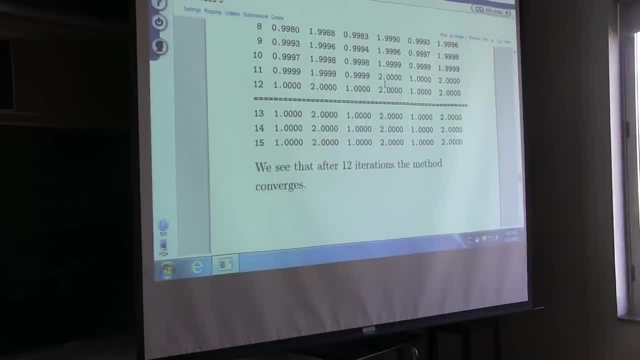 I see that I have one, two, one two, one two accurate to four decimal places right. and then I stop because the criteria is met and I believe I was measuring the L-infinity norm here. each element must be accurate to ten to the negative five. is that clear? that's the L-infinity norm. 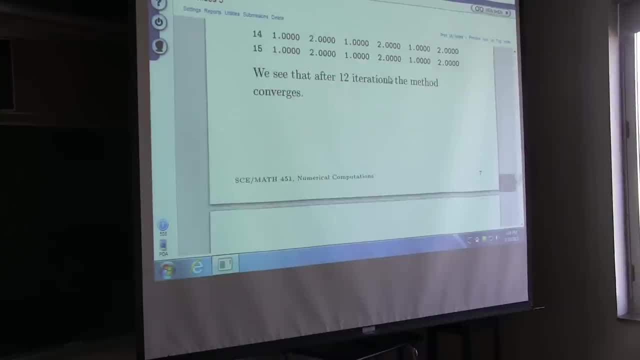 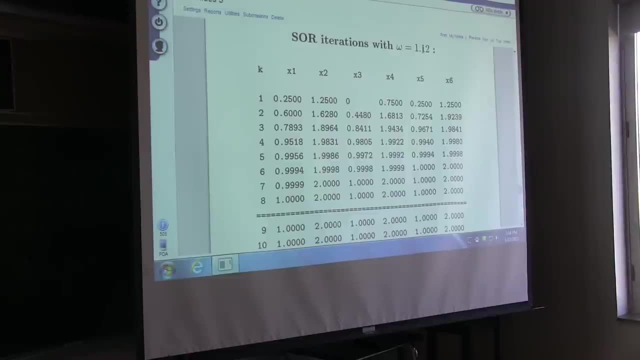 I'm measuring, Okay, so about twelve iterations, and then we did it with SOR and I chose my relaxation parameter to be one point one, two, just a little bit away from Gauss-Seidel. if you choose this number a little bit bigger, It might perform better. okay, so just a little bit, and then let's see the improvement from. 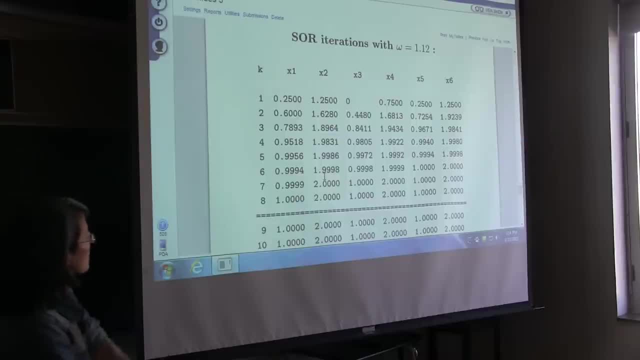 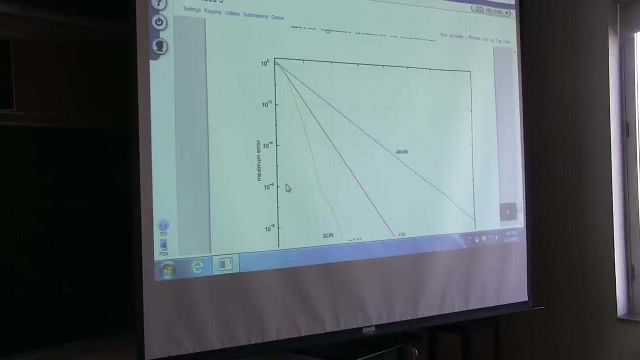 Gauss-Seidel. so remember, Gauss-Seidel was twelve iterations, and here we see, after eight iterations, it's good enough, Is that okay? So that's all that. that's like just one iteration. so what I want to do next will be analyzing these three methods side by side in the same graph. how do you represent your result? 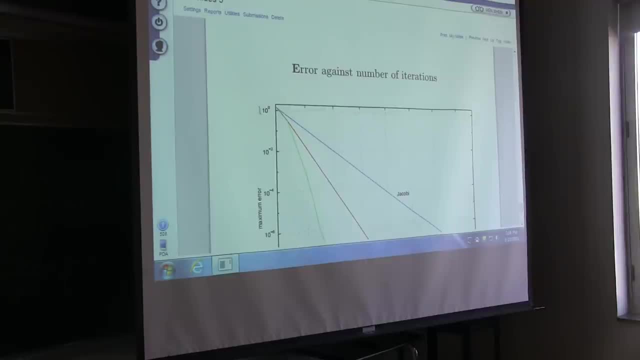 Well, I'm going to plot the arrow against number of iterations. so you know, each iteration you run the L-infinity norm of your arrow will become bit smaller and bit smaller and eventually converges. so I can plot these okay. so these are the arrow plot. let's shoot the. 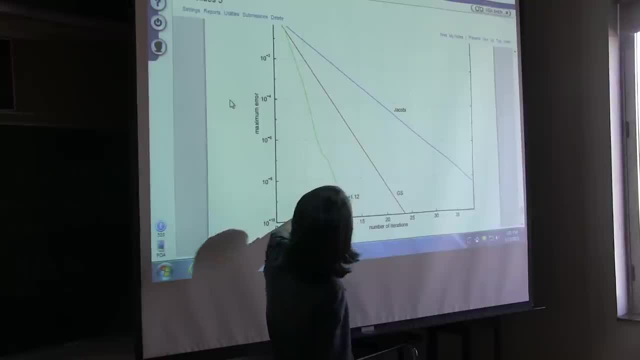 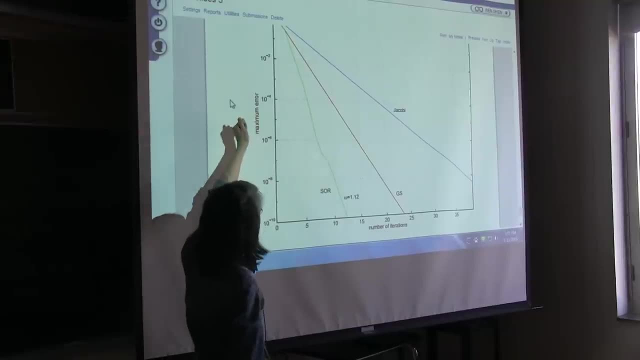 blue one is for Jacobi and the red one for Gauss-Seidel and the yellow for SOR. so you see arrows, all Okay, The arrow decreasing, and this is plotted. the arrow is plotted in the logarithm scale so it's easier to see the magnitude. so let's say your tolerance is ten to the negative. 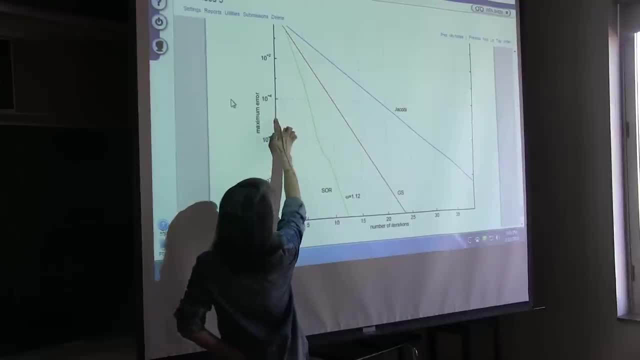 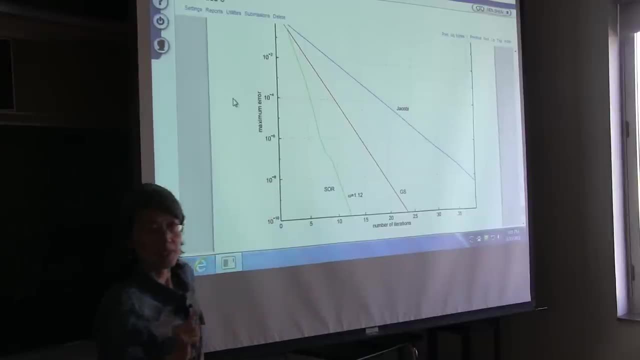 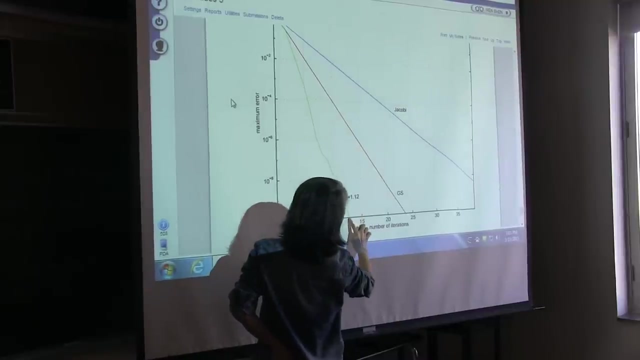 five. how many iterations do you think that Jacobi will have to perform? you check over here. ten to the negative five. you look down you see probably twenty-four iterations. do we see that? and the Gauss-Seidel coming over is about here and twelve or thirteen iterations. 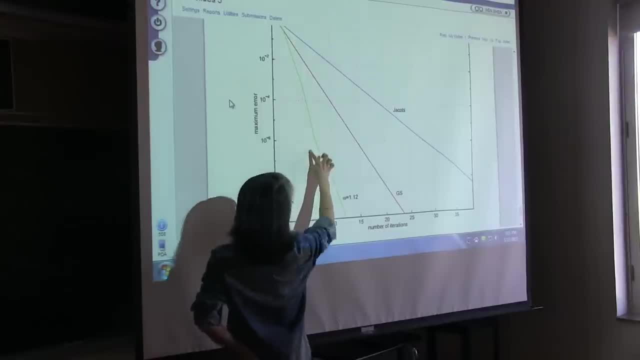 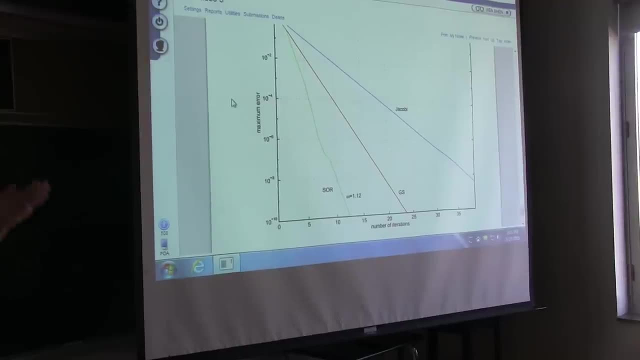 right, and SOR hit over here, come down, see about seven iterations. okay, so SOR goes down faster here, but they all go down in a straight line, because this is linear convergence. all right, is that okay? so for your next homework there will be something a little bit similar. 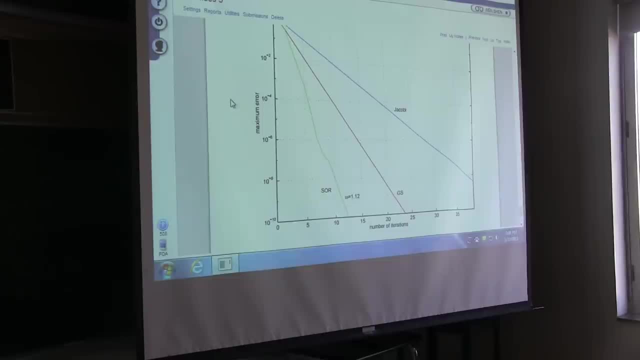 hmm, did I ask you to do that? no, I think there will be an SOR and ask you to plot um number of iterations needed as a function of different relaxation parameter. okay, so you have to plot something else there, okay, is that okay? any questions? hmm, this is not. 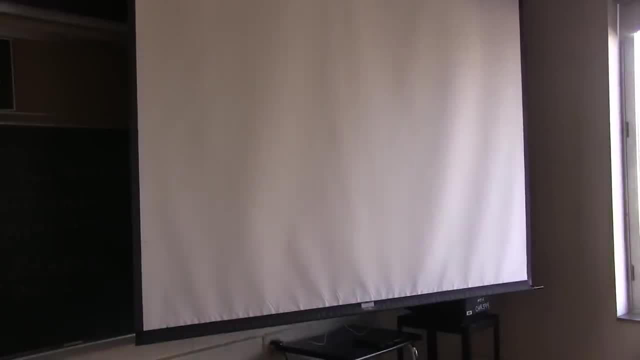 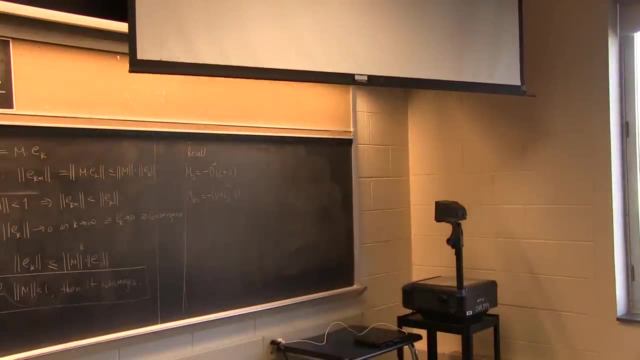 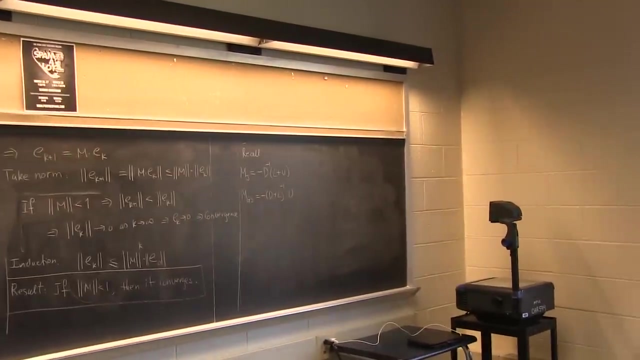 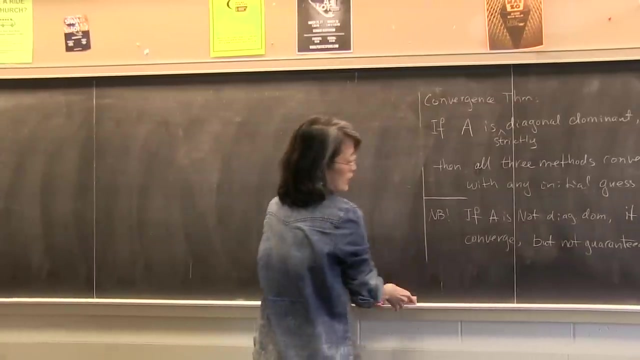 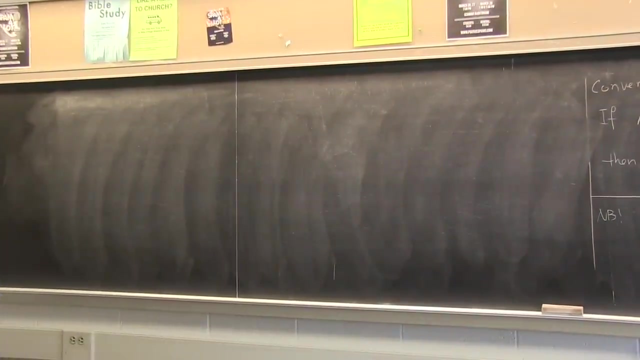 listening to me. okay, screen up, check one front, all right. if that's okay, we move to the next topic. so, as I say, that's not the end of story of numerical linear algebra. okay there, these are just very soft methods. there are many other hardcore methods, much harder, much better, but okay, so we change the order. okay, so we. 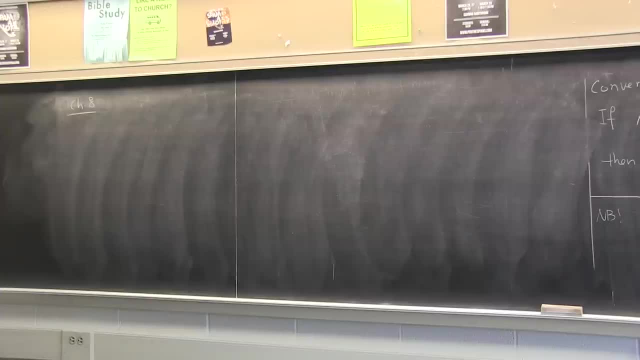 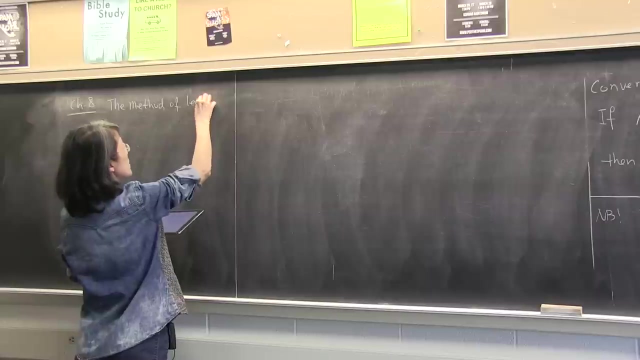 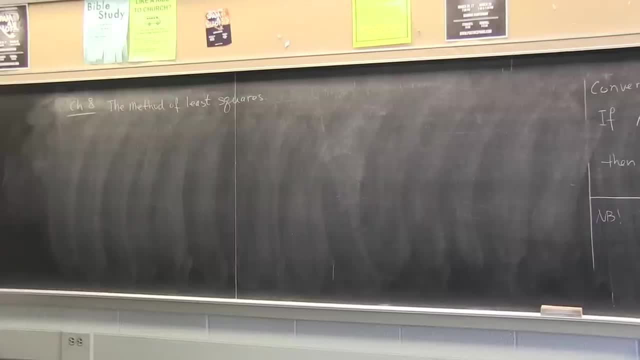 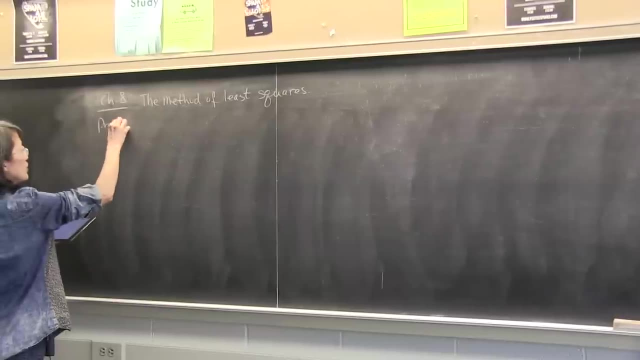 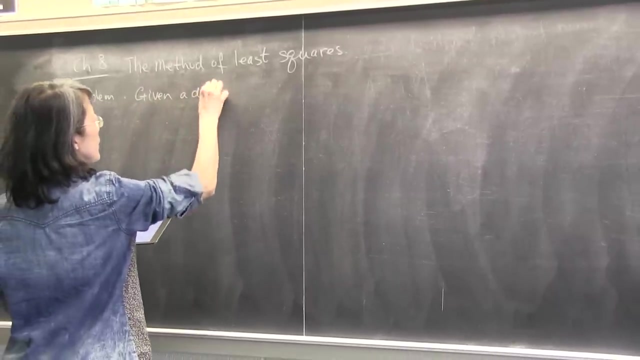 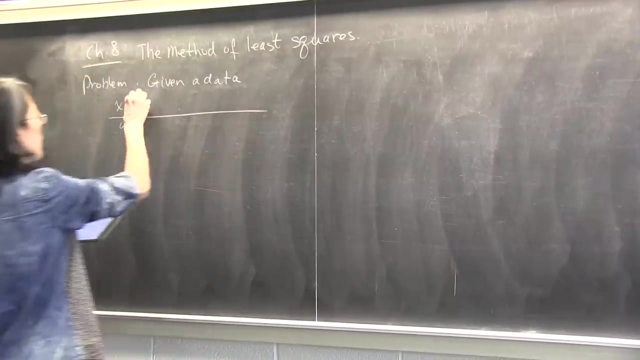 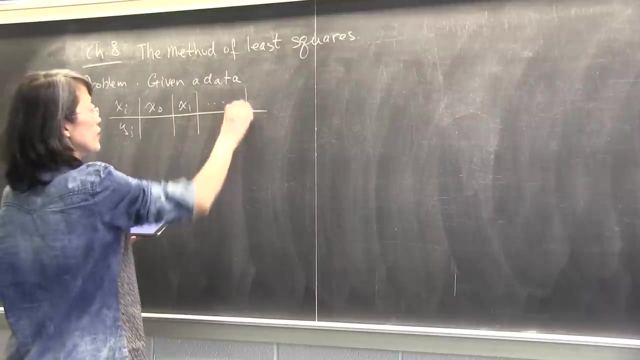 squares- have we heard of it? the name sounds familiar- least squares. okay, so let's set up the problem. so the problem is the following: I am given a data set data, so x in y, I. it's similar like polynomial interpolation, but not really. we're not interpolating, we are feeding X, mmm, okay, and 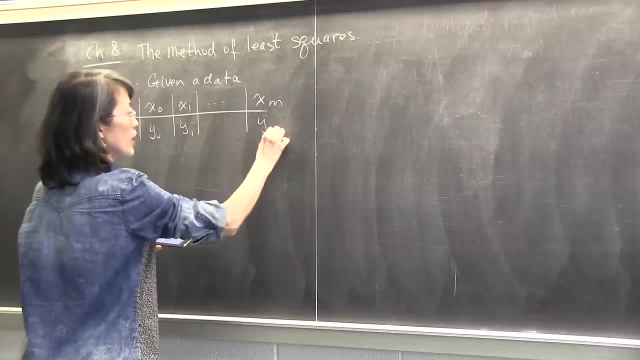 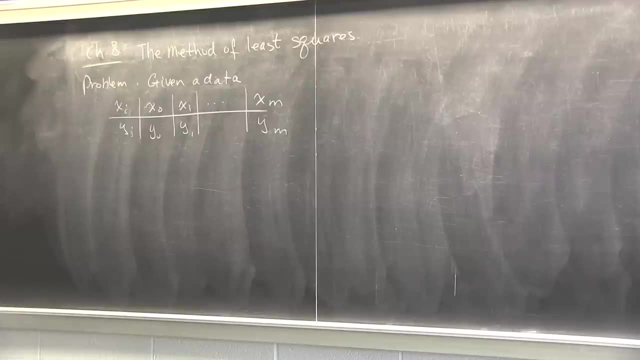 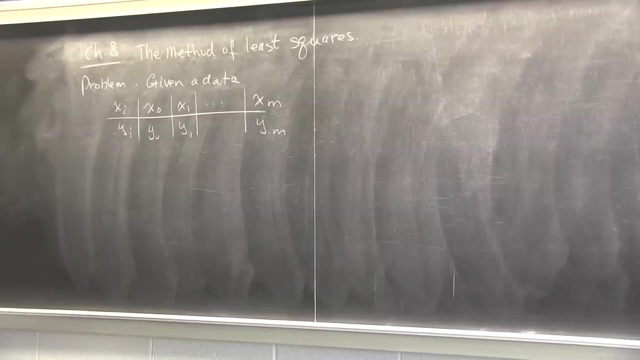 then I have y, zero y, 1 y, and so I have a plus one points given in the data, okay, And they can be data from experiment, from measuring data, and it can contain arrows. It's not accurate. You might be doing some lab and you get some data and then you know, you have some idea what. 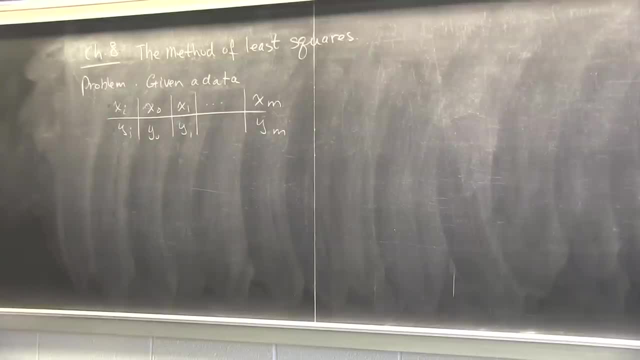 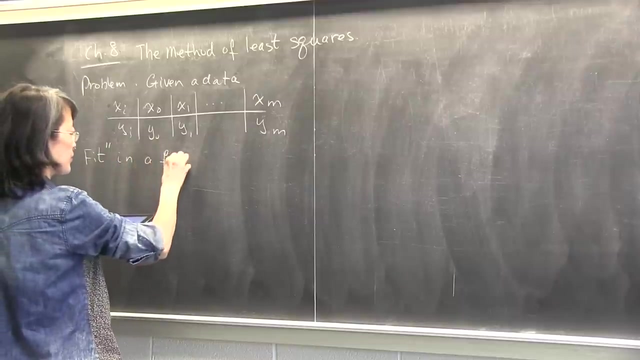 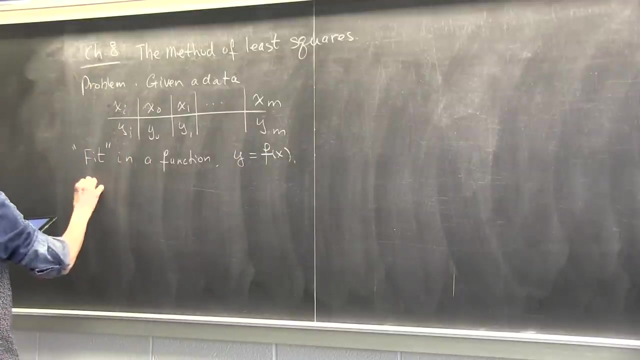 what the relations shall be and there might be some parameters and you have to fit in. Okay, So the goal is to fit in. we'll have to explain what mean Fit in a function. so y equals to F, x, such that the arrow. so what will be? 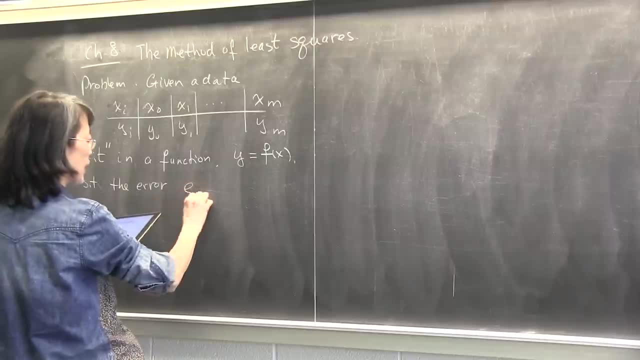 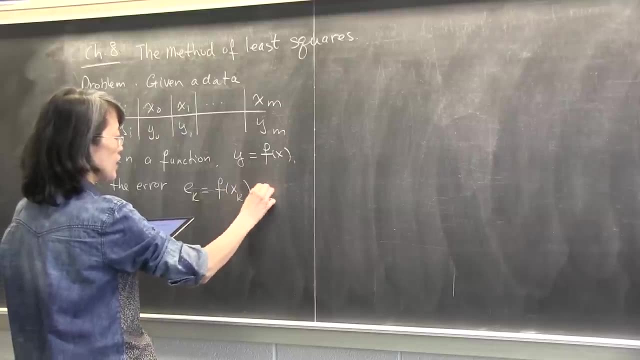 your arrow. if you fit in, So your arrow will be e k will be e k. if you fit in, So your arrow will will be e k. what will be the error? less, less, less, which is equal to f of xk, the exact value minus your. 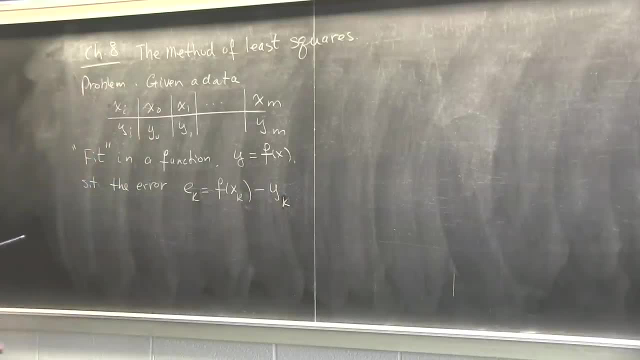 measured value yk, right. And then you have m plus 1 of such points, right. So you have to come up with some notion. It's minimized, And then we have to define What do we mean by fitting And what do we mean by minimize the error? 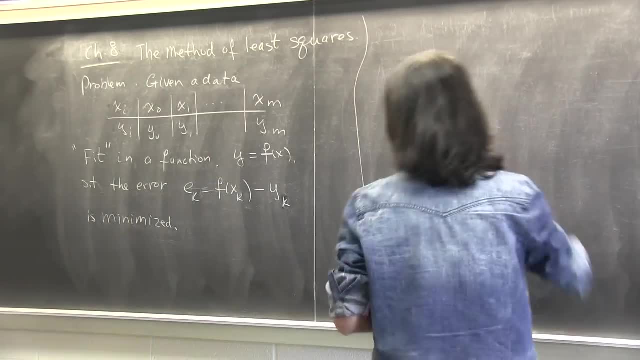 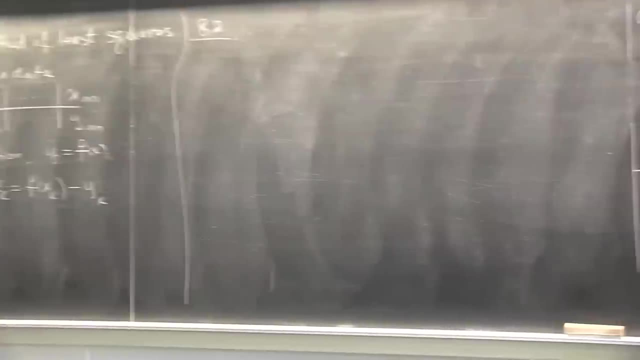 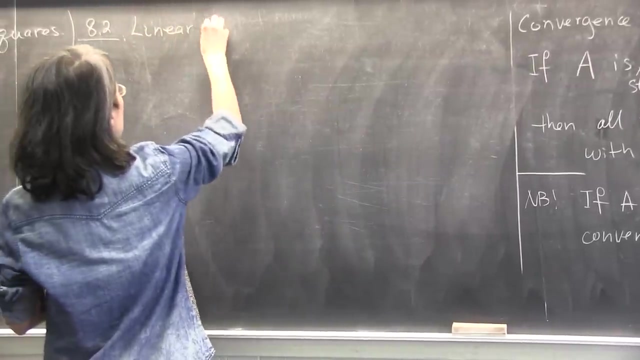 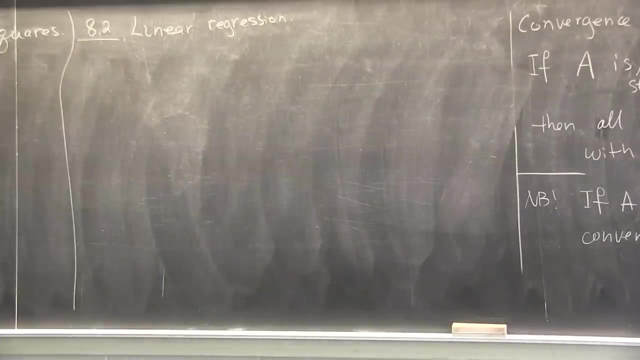 Is that clear what we do? So let's start with a simple choice. That is, I'm trying to fit in a straight line, So this is called linear regression. So I'm trying to fit in a straight line and go through some derivation. 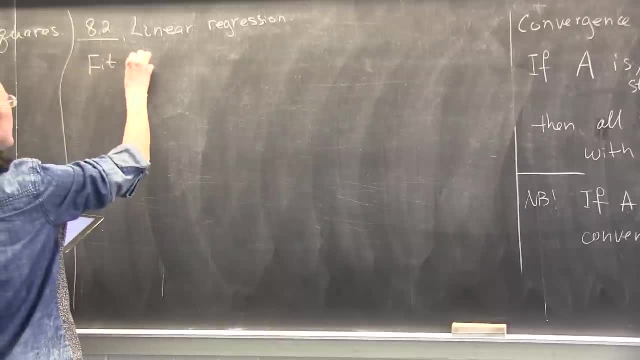 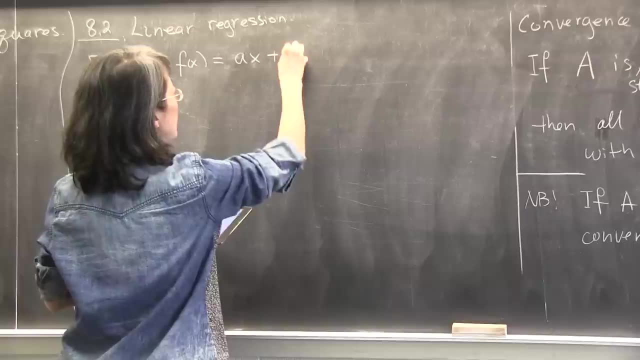 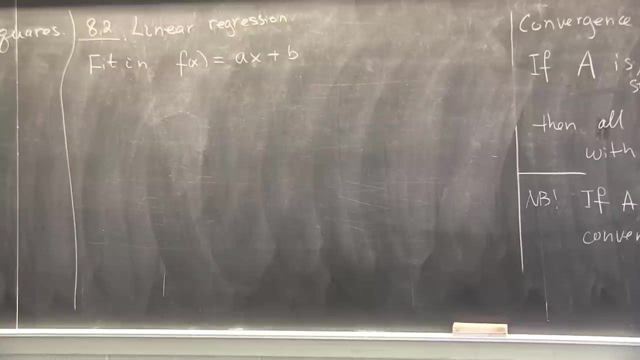 So We will want to fit in a straight line. That means we'll want to fit in the function f of x, so equal to ax plus b. So a is the slope and b will be the intercept, And we want to fit into this data. 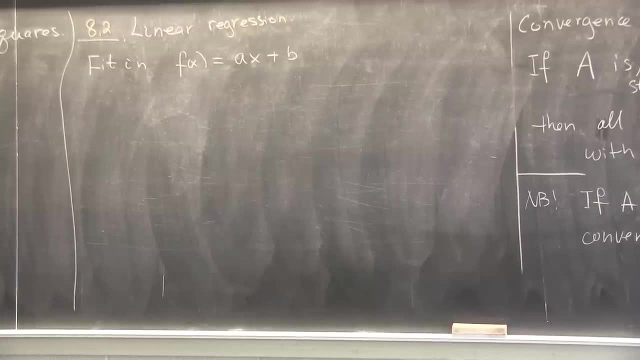 And you know this data might lie in a neighborhood around that straight line, but it will not be a straight line. So if this shall be your lab result- and you know it has to be a straight line and your result lies perfectly in the 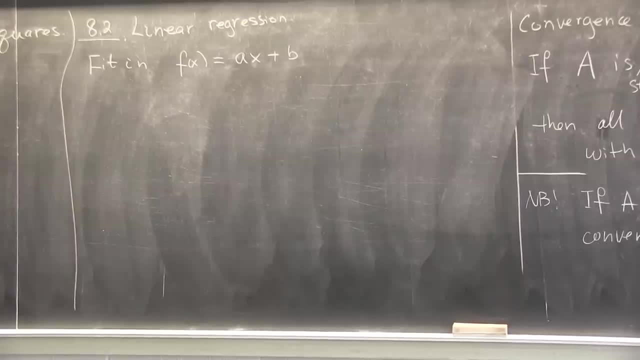 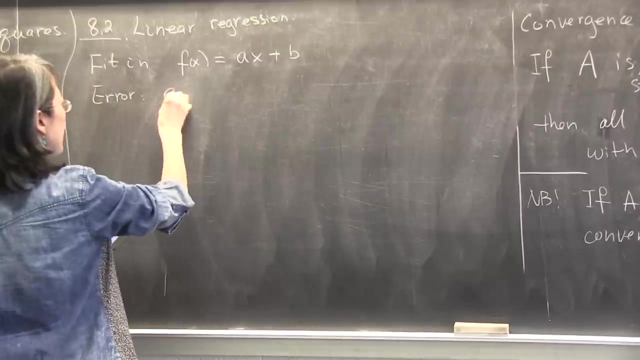 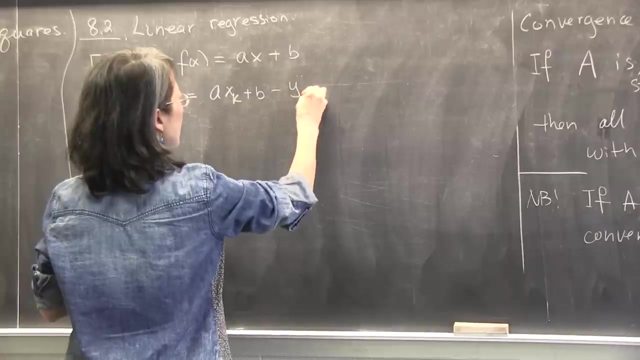 straight line. that causes a lot of suspicion on how you get those data right. Usually you don't get it. You have to fit it in, OK, And then what will be your error? Error at a point. Each point. ek will be axk plus b minus yk, right. 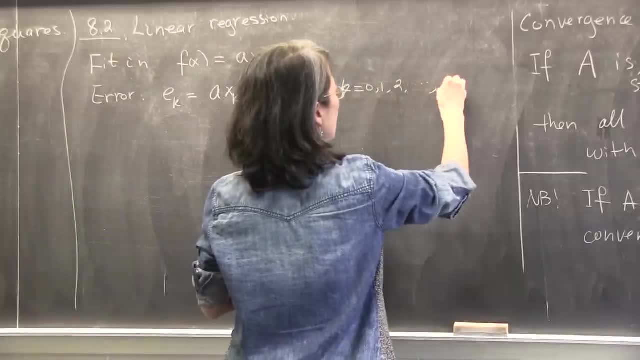 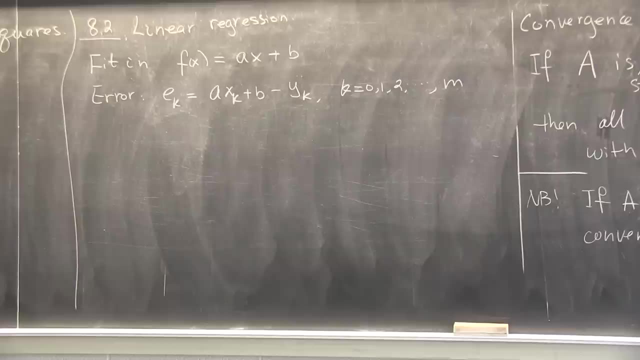 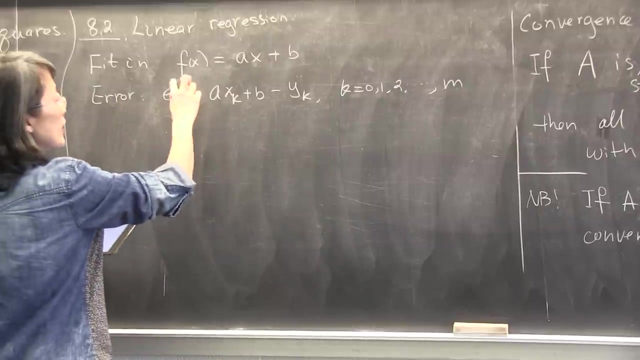 k equals to 0,, 1,, 2. And all the way To m, m plus 1 points. And we want to choose some lines. So here the choice you have to make will be this line, right? So you have two parameters, a and b. 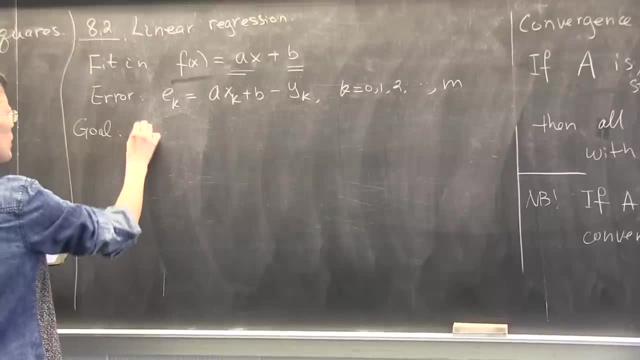 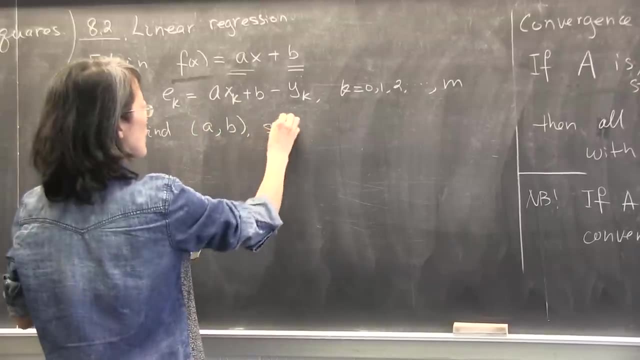 So now your goal becomes a bit clearer. Now it's the following: I want to find this pair of coefficients, a and b, such that this arrow is a And this arrow is a, So I can use k as my кажemeter. 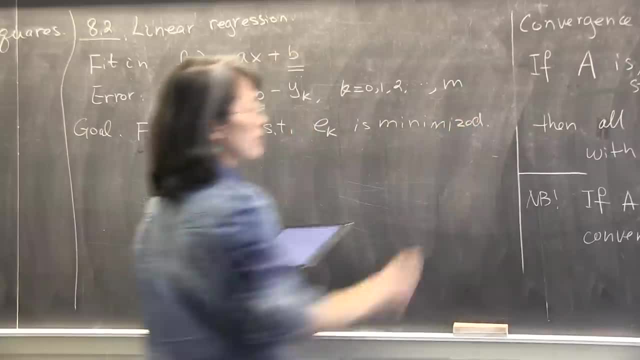 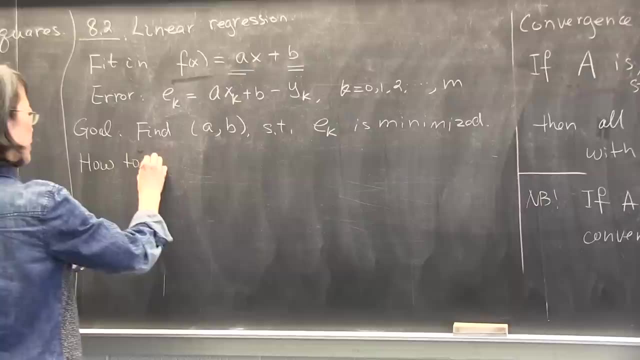 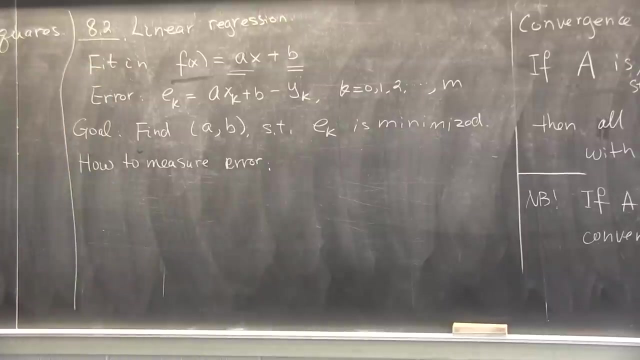 Now, when you calculate this, I just go with the equation given by limit used in the chi line on the basic data drop, that's what we call. it equals And that around it this e to the k is minimized. Is that right? 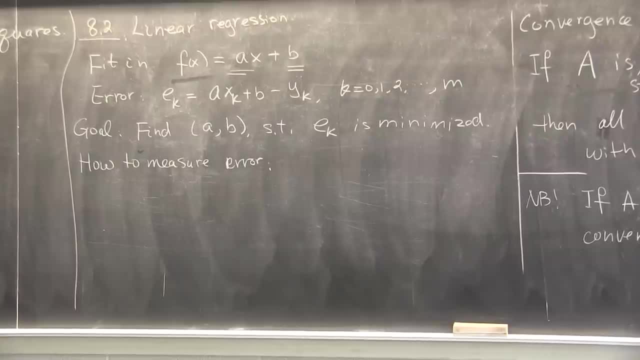 OK, How do you measure a vector? We just talked about norms for a vector, is it? Can we throw in one of those norms? So let's look at those three choices. Say, you can throw in the infinity norm. that is the. 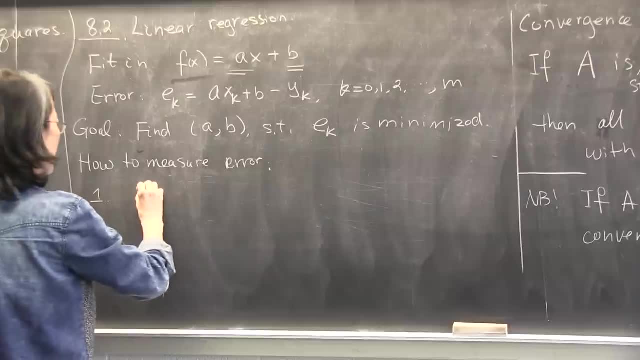 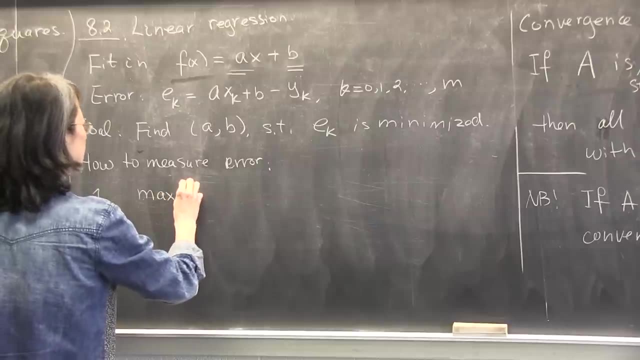 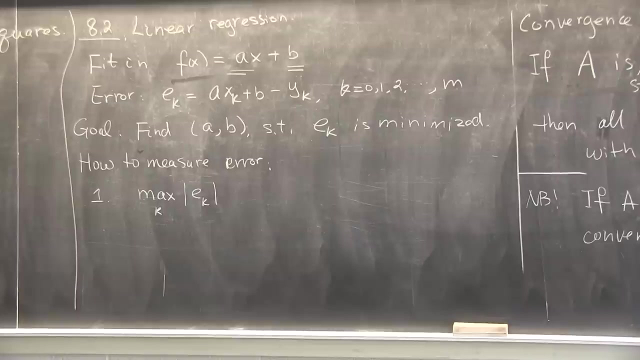 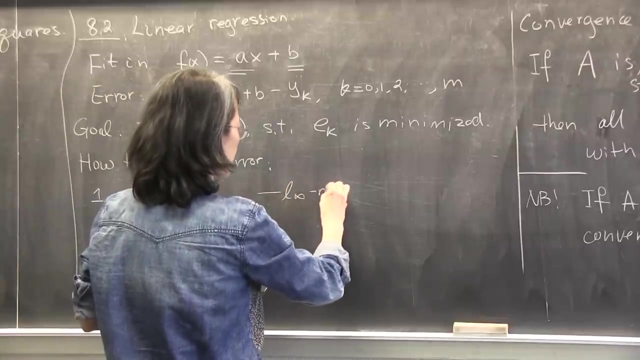 absolute value at every point is measured. So you will be looking at the maximum of absolute value of e k over all k. You can try to minimize that guy, Can we? Then you know this corresponds to the L-infinity norm for the vector norm. 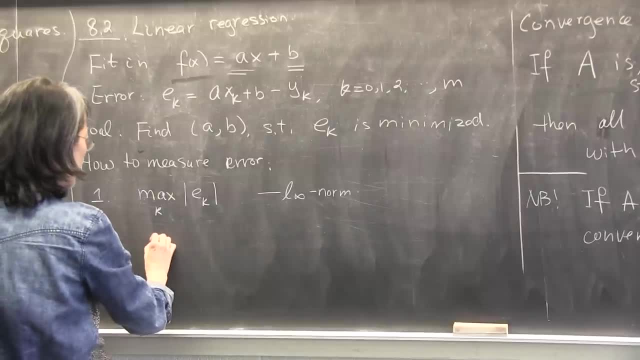 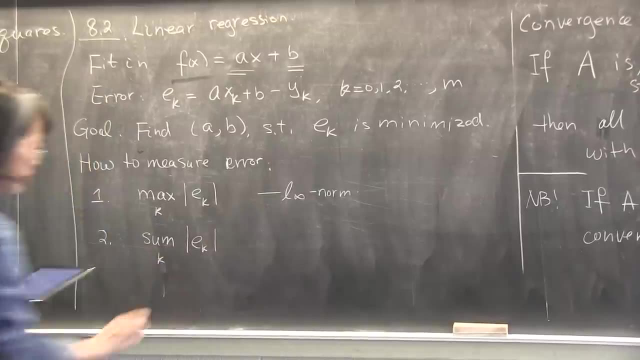 And also you can put in the L-1 norm, That is, I will be summing up all the e k's in absolute value over all k. So my vector, error vector- I just add them all up in absolute value. 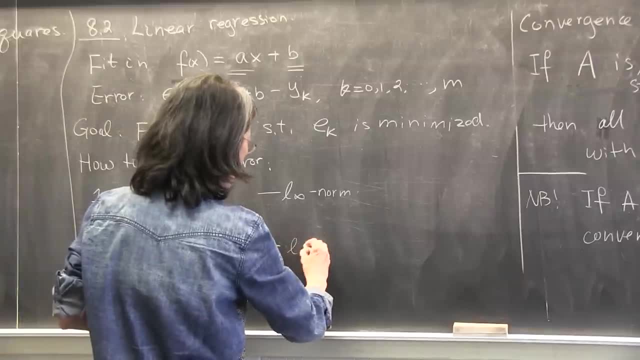 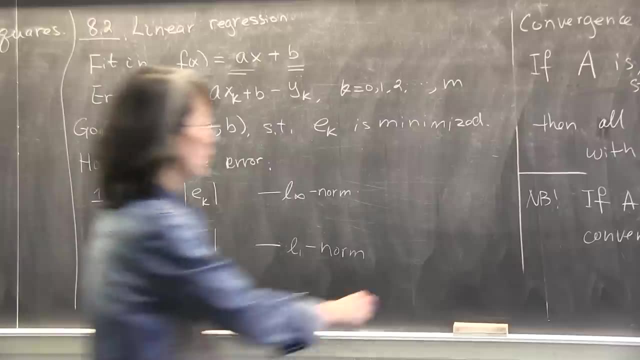 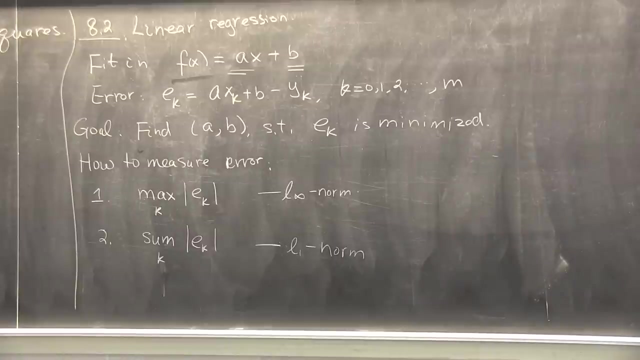 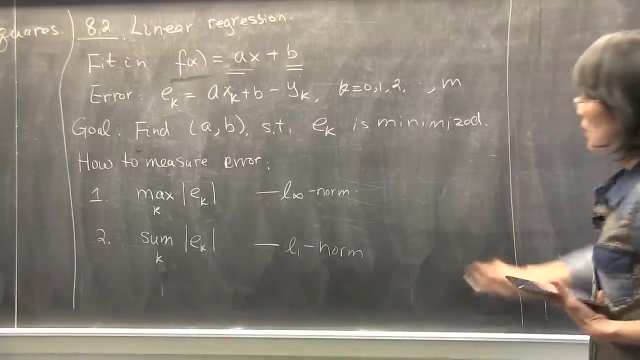 And I try to minimize this. So this is the L-1 norm. They are both legal choices. You could set them up and try to solve the mathematical problem coming afterwards. And the reason that we don't choose these two is that the problem coming from these are very bad, very difficult to 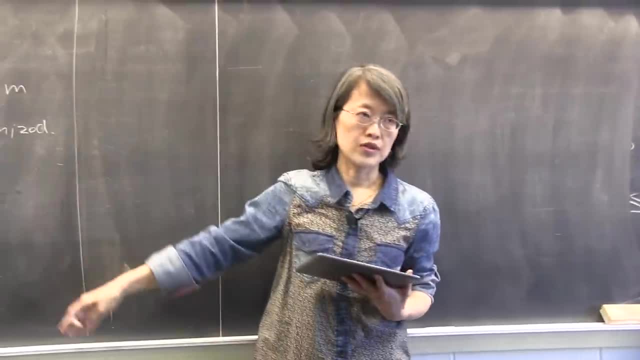 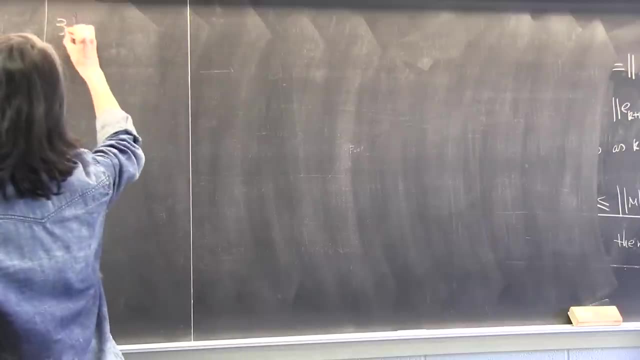 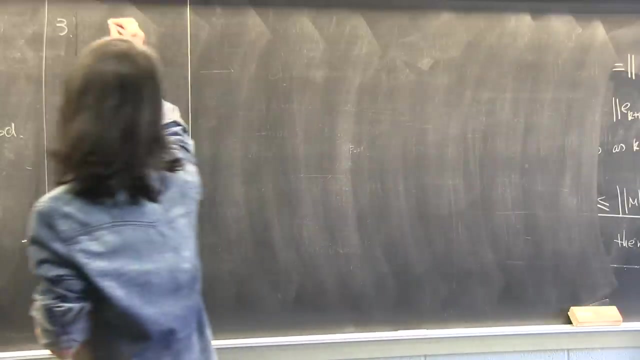 solve. They are nonlinear, The solution discontinues. It's a whole mess. The choice that we want to talk about now- using the L-2 norm- gives you very nice problems in the end, So that's why we'll be choosing that. 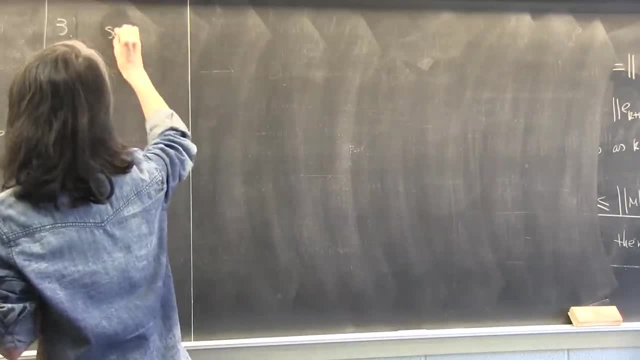 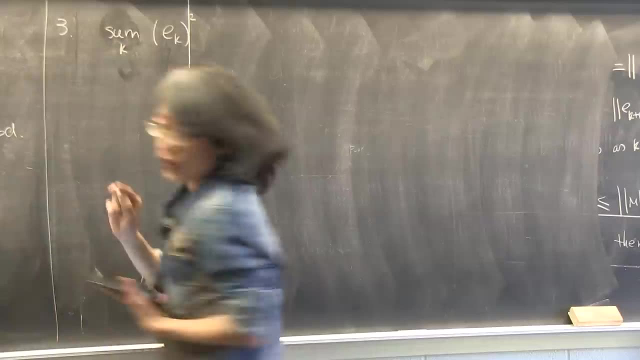 So we'll be choosing kind of the L-2 norm. Let me write some summation. Remember the L-2 norm. We'll be taking each element, square it and sum all over. So I know in the L-2 norm there is a square root on top of all. 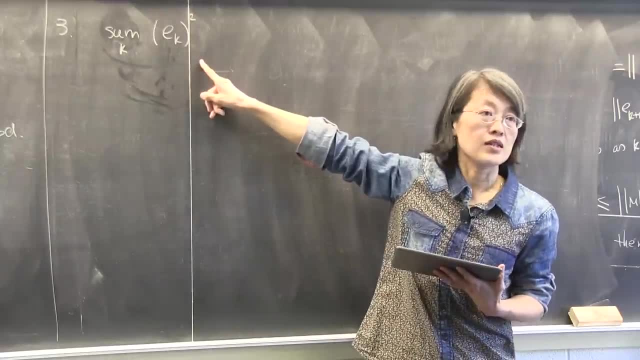 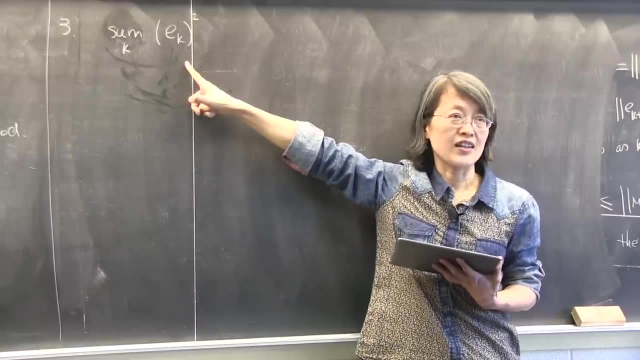 that. But if this guy is minimized, so is the square root of this guy. So there's no need for me to take square root. So I'll be minimizing this guy. OK, So that actually comes from the L-2 norm. 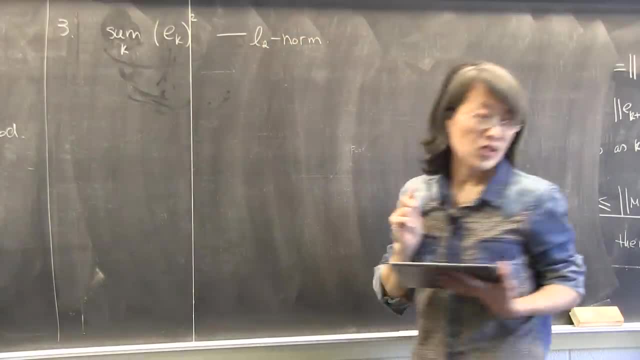 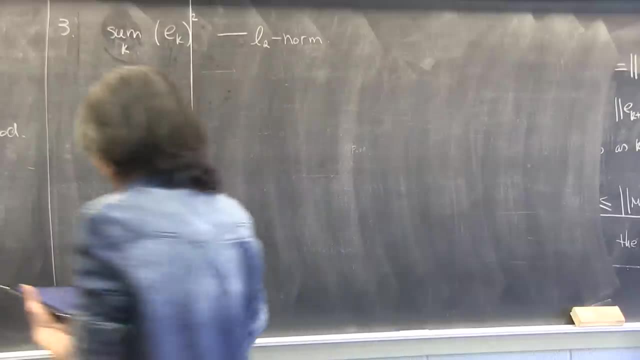 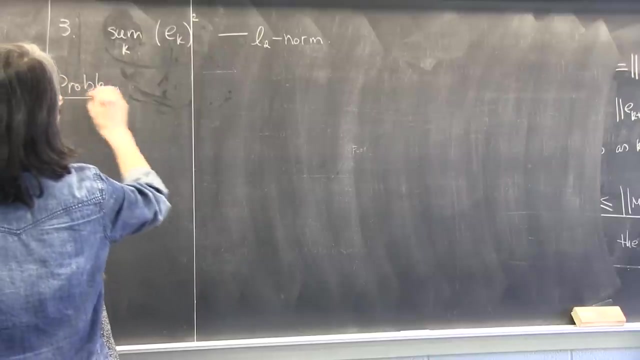 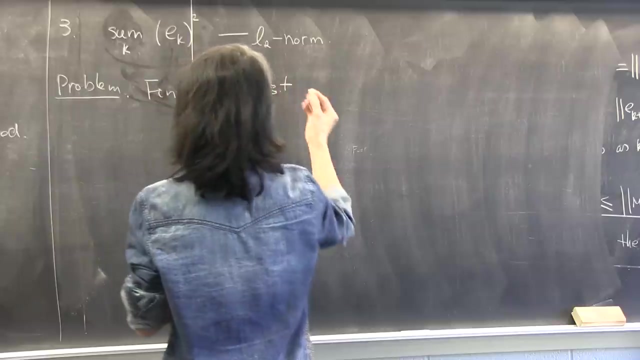 OK, That's why the name is called least squares. OK, out of all the squares and try to minimize it. OK, so now our problem becomes even clearer. Let's define. Our problem will be: find coefficients a, b such that: 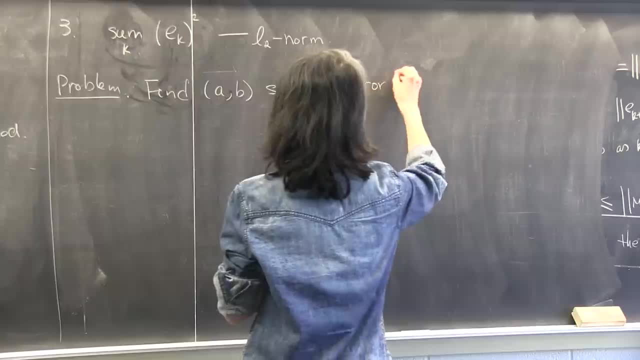 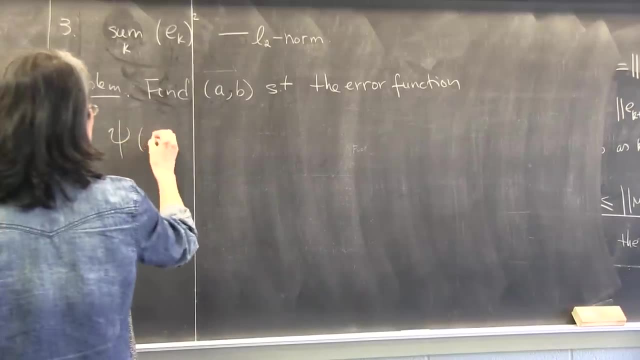 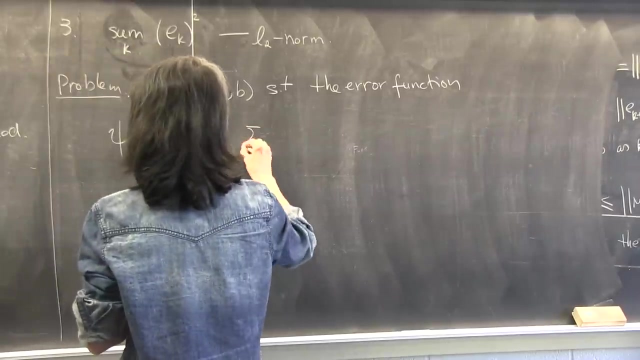 now I can define my arrow function. OK, so let's call my arrow function psi. I know the psi will depend on my choice of a and b. Let's define it. It will be just the summation i should I use i. 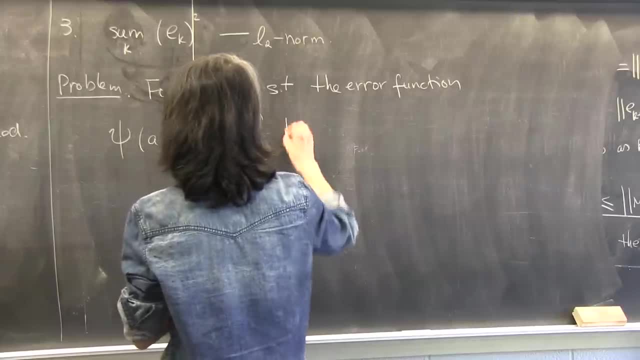 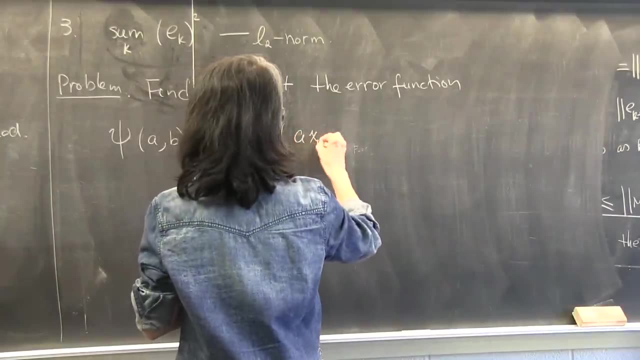 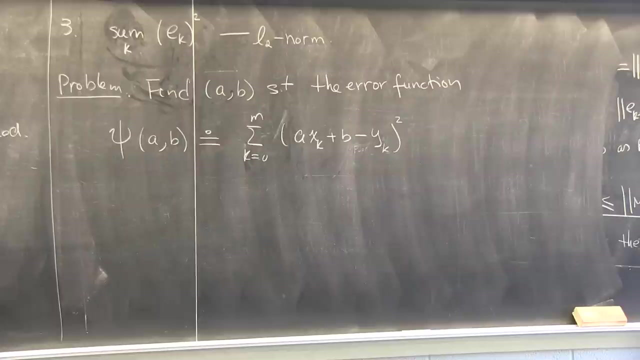 We're having k here, So k from 0 to m of the arrow, and I know my arrow Arrow is this guy, so let me put it axk plus b minus yk. OK, So I'm going to add up my arrow function and I'm going to 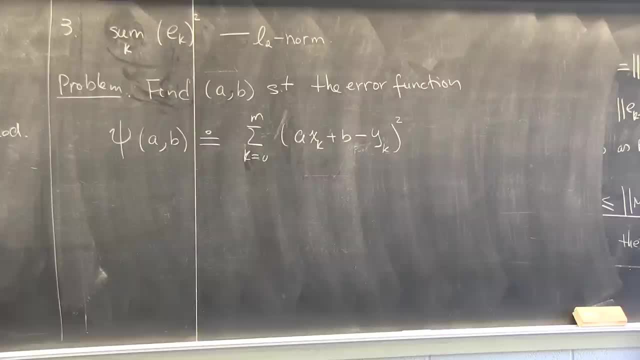 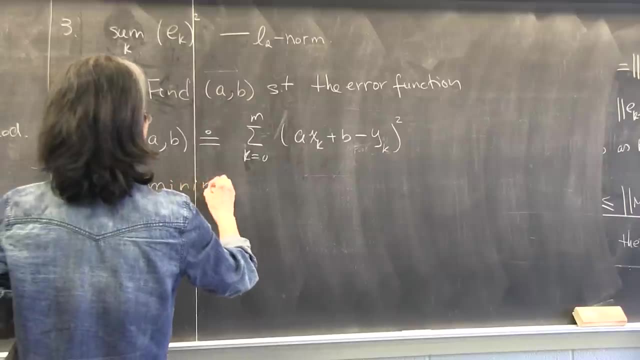 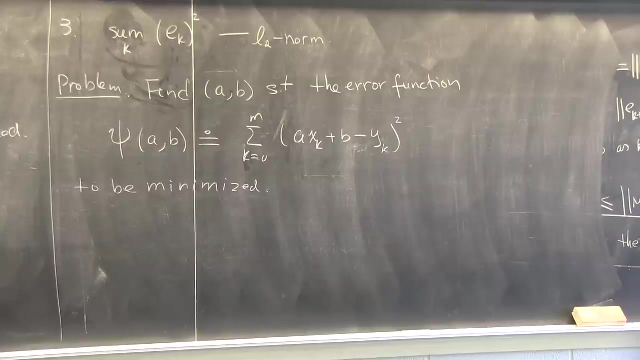 add up my arrow function. so I'm going to add up my square Right. I square arrow at every point and then I add them up. That's my arrow function. in the end, I want this one to be minimized, Is that clear? 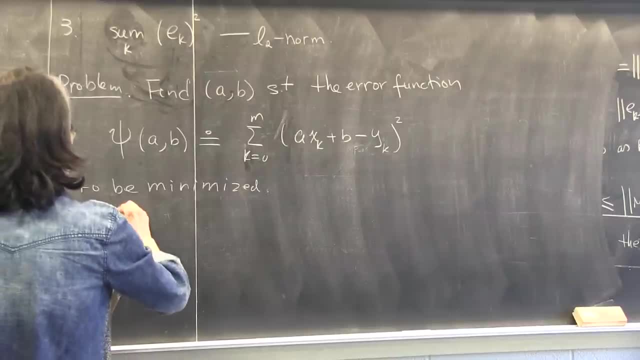 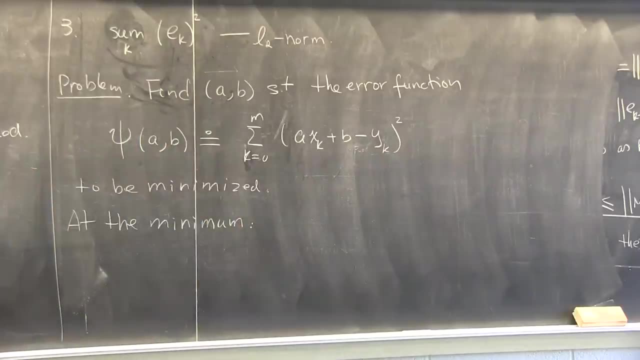 Now we have a very specific problem now, OK, So let me ask you the question: What do I know? What properties will be satisfied if I shall find the minimum of this function? This function now depends on two variables: Depends on a and depends on b. 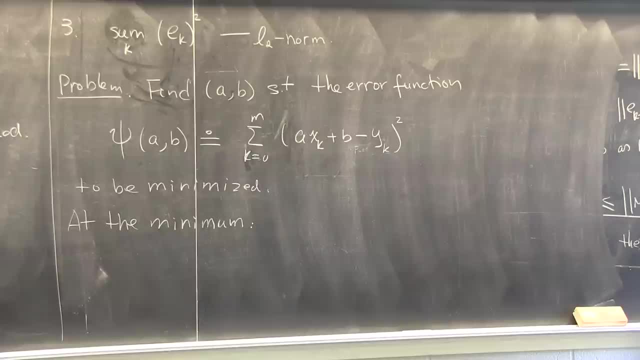 We've taken 230.. The minimum of a multi-valued function is a critical point. What property does it have? 3.0.. The derivative. Well, here I have two parameters, So you have to call those derivatives partial derivatives. 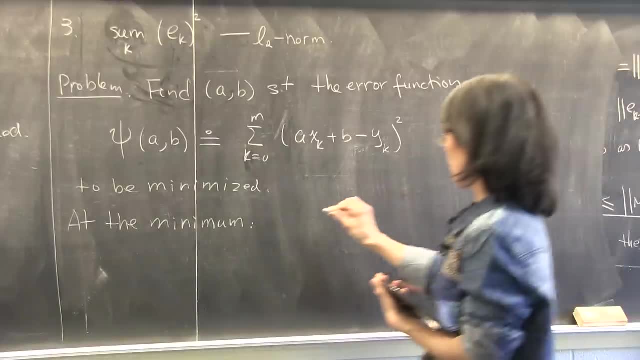 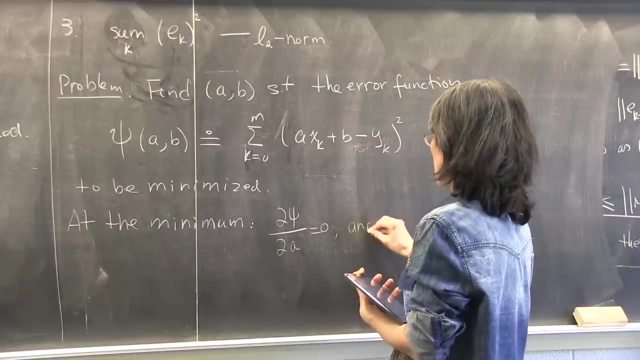 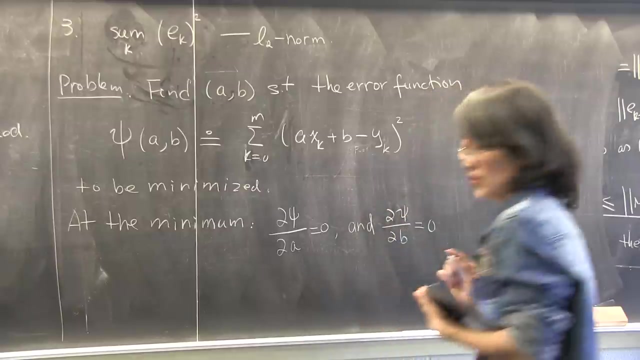 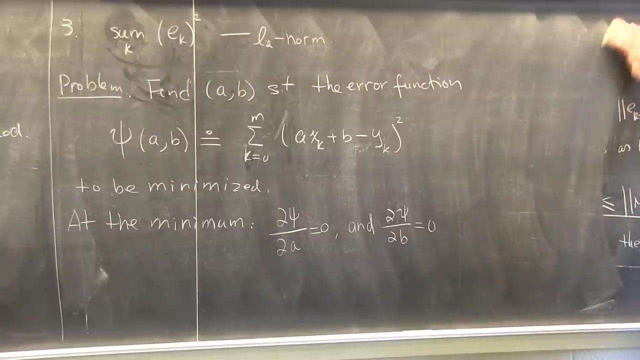 Is that right? So, at the minimum, I have the following: Partial phi over partial a equals to 0. And they must both be satisfied. OK, Partial phi over partial b has to be 0. Is that right So? but you know, if you want to make sure this is a minimum, 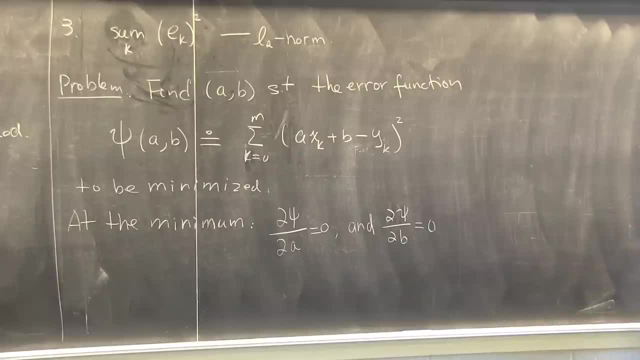 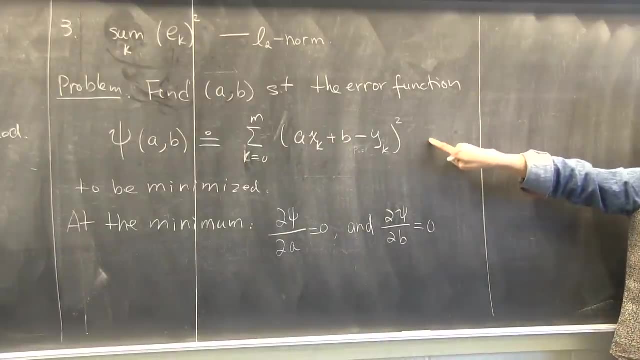 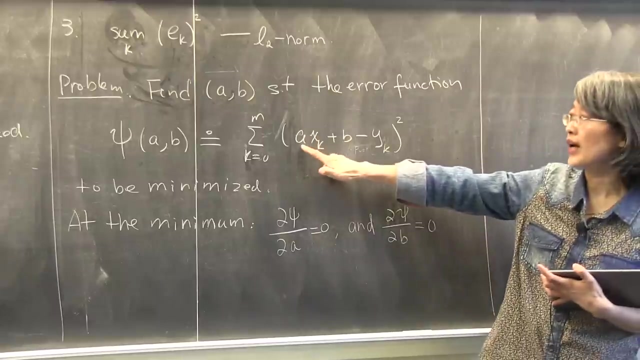 you have to have the second derivative test, right. So for the problem like this, setting up by minimizing the square, this is some kind of a parabola, OK, And then you're squaring it, And then what you have here is x squared. 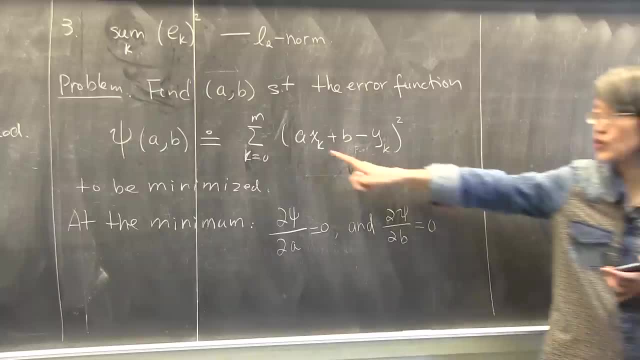 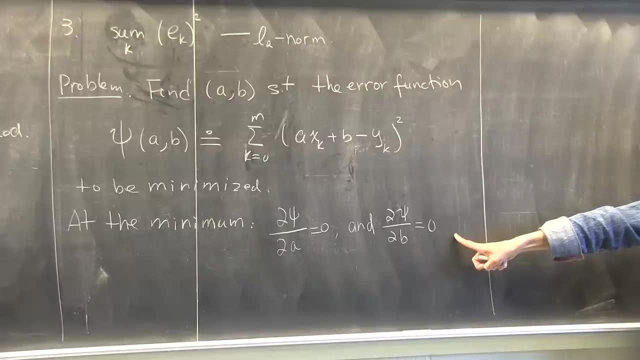 in front of a square, So all the coefficient in front of the square term will be positive. That's the only critical point for this function And it will be a minimum guaranteed if you are minimizing in this way, So that becomes the only thing you need. 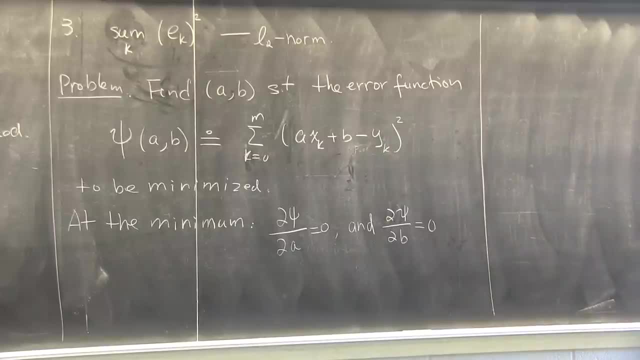 Is that clear? So you can go ahead and verify the second derivative. You can be sure that it works. So do I have time to go into it? No, How about we stop here, and then I will derive the detailed equation next time.